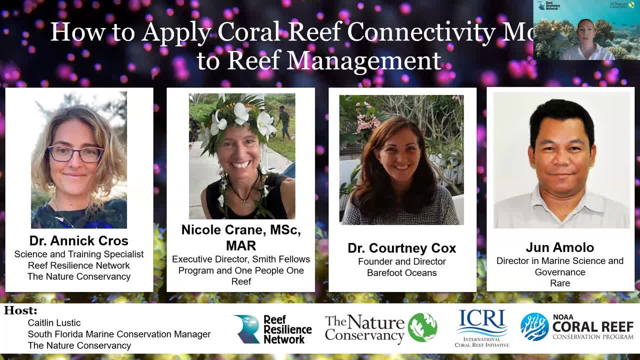 Her primary areas of conservation focus are on community-led coral reef conservation and management. The One People, One Reef collaborative is focused on authentic collaboration and co-creation of action plans with indigenous and local communities, developing conservation and management tools aimed at protecting reefs and the people who rely on them. And Nicole has some. 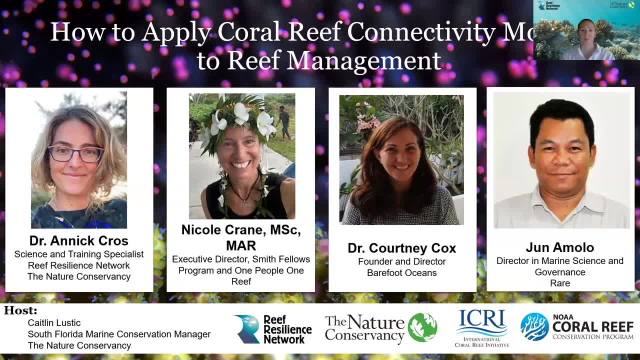 special guests that will be joining her and she will be joining us in a moment. She will be introducing them during her talk. Next we'll have Dr Courtney Cox. Courtney has a PhD in coral reef ecology and extensive expertise in assessing fisheries management strategies. 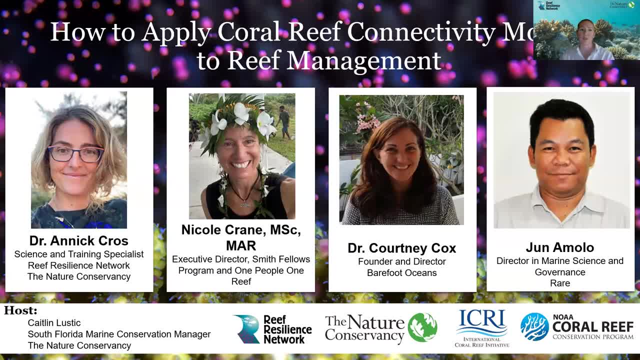 and identifying factors driving ecological and social change. She has supported teams across 12 countries in enhancing data collection methods, designing protected areas and implementing efficient adaptive management approaches. She is the founder and director of the One People, One Reef collaborative. She is also the founder and director of Barefoot Ocean, a social enterprise. 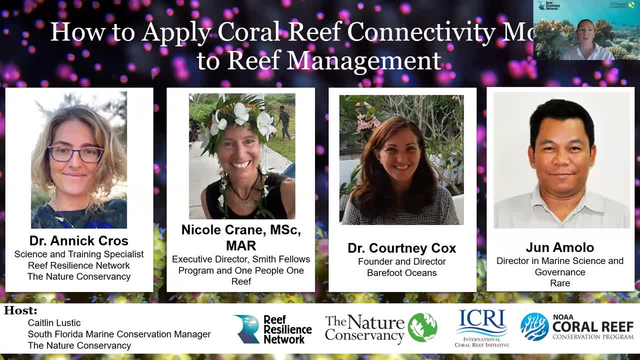 dedicated to empowering individuals, communities, governments and local organizations with science and data. And finally, we'll hear from June Amalo. June possesses more than two decades of expertise in coastal resource management initiatives spanning diverse sectors, including academia, national governmental bodies and non-governmental organizations. His professional 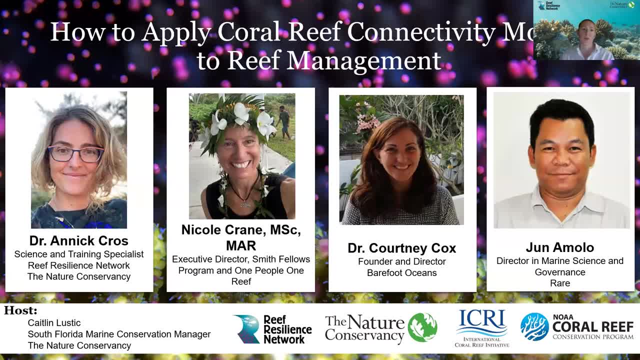 journey has been deeply rooted in the Philippines, notably focusing on the Visayas and Mindanao regions. Presently, June holds the position of director in marine science and governance at RAIR, where he has dedicated his efforts for the past 11 years. Next slide, Sheri. In case anyone is unfamiliar with Zoom webinars, here are a few. 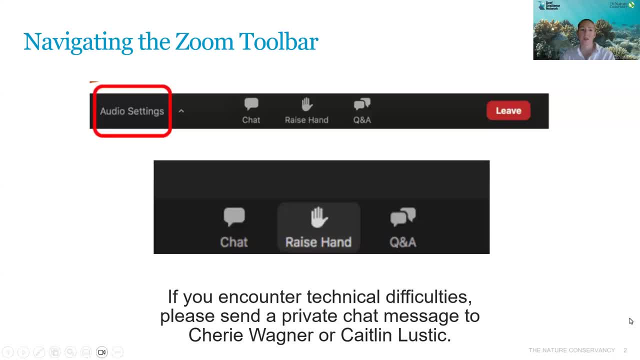 housekeeping items. On the left, you'll see an audio settings button. You can click on the up arrow and select from available audio output options, such as speaker speaker speaker speaker speaker speakers, headphones or other Bluetooth devices, If you experience any technical difficulties, 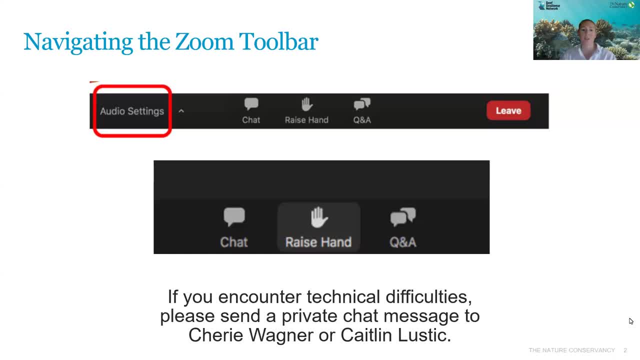 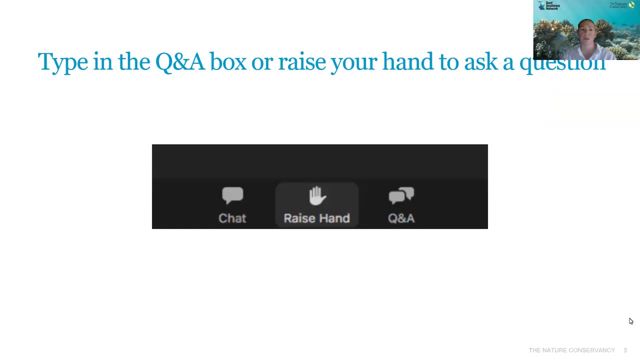 such as not being able to see the slides or to hear us. please use the chat feature to send a private message to Sheri Wagner or myself and we will be able to assist you. After each set of speakers, we'll have five minutes for questions and then we'll have a full Q&A session at the end. 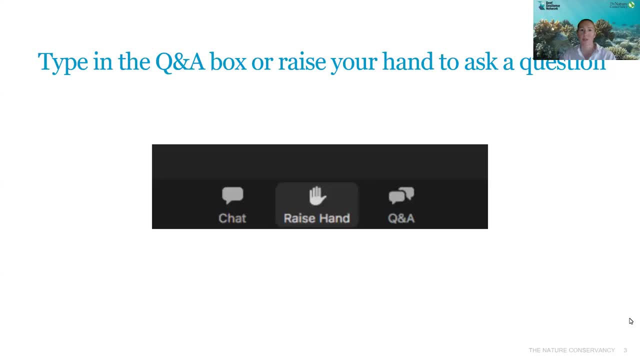 You can use the Q&A feature throughout the webinar to type any questions you'd like to ask. If you have any questions, please feel free to ask them in the chat box. You can do that either with your name attached or anonymously, And then during the Q&A session. 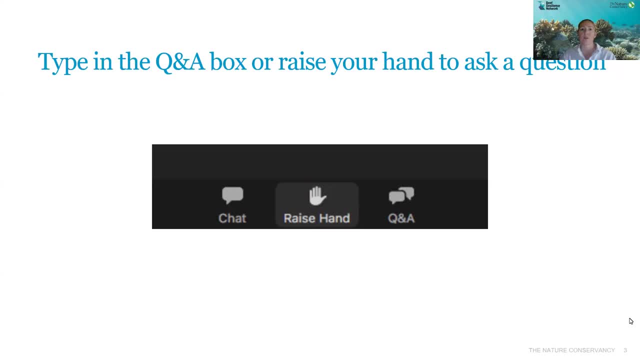 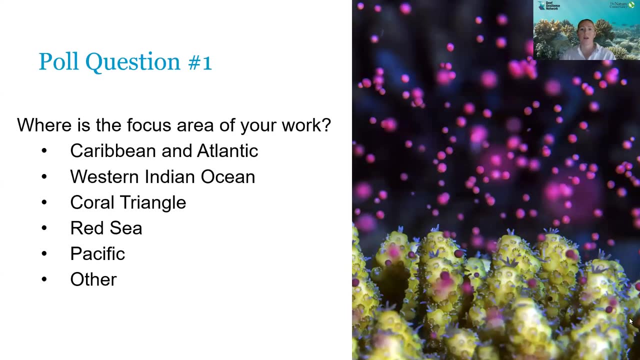 after the presentations. you can also raise your hand using the raise hand feature if you'd like to be unmuted to ask your question yourself. So first we'd like to get a sense of who's with us today. So we have two poll questions. First, please tell us where you work. 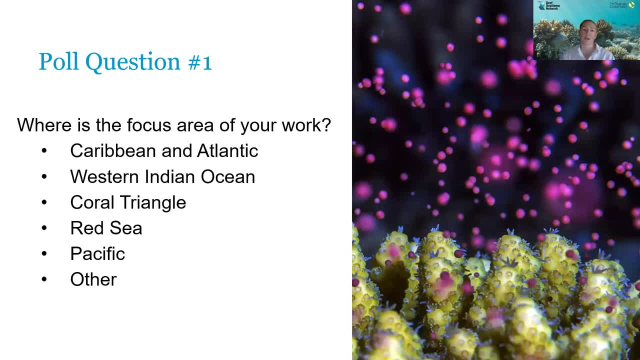 In the Caribbean, Atlantic, the Coral Triangle, the Pacific, the Red Sea, the Western Indian Ocean or other, And you can choose more than one. Okay, So we have mostly from the Pacific, which we assumed because of the timing, but also a pretty good showing from the Caribbean and the Coral Triangle. 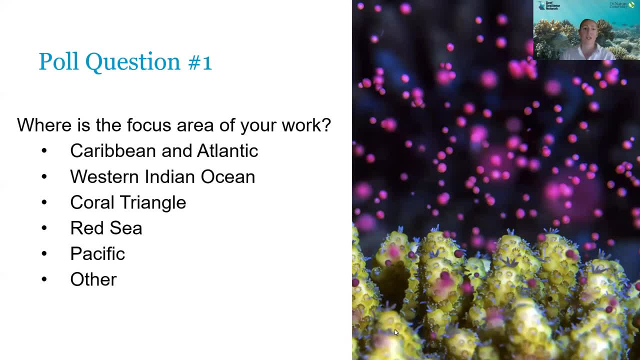 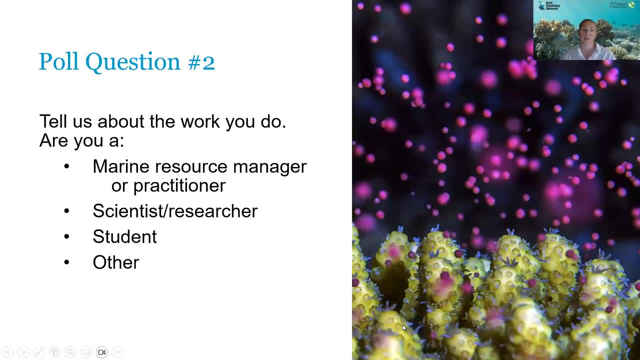 Okay, And then for the second question. we just want to get a better sense of what type of work that you do. So the question is: are you primarily a marine resource manager or practitioner, scientist or researcher, student or other? Okay, great. 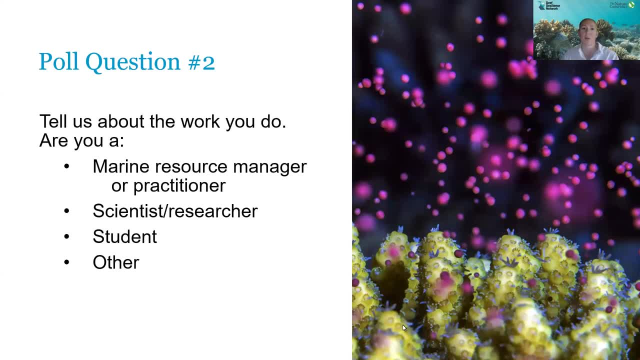 So we have mostly scientists or researchers, followed by marine managers and some students and other. Thanks for that. That helps our speakers understand a little bit more about where people are calling in from and what their roles are with their organizations. And with that I'm going to turn it over to our first speaker, which is Aneek Cross. Go ahead, Aneek. 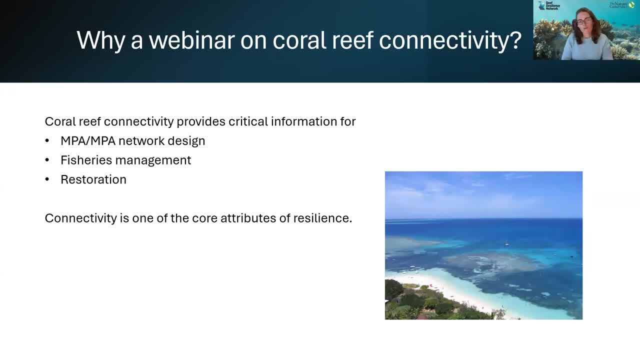 Thanks, Caitlin, for this great intro Today. before moving on to our other experts, I wanted to talk a little bit about why we're doing a webinar on coral reef connectivity and some of the challenge we've had throughout the years. So marine connectivity has been a topic of interest for coral reef managers for over three decades. 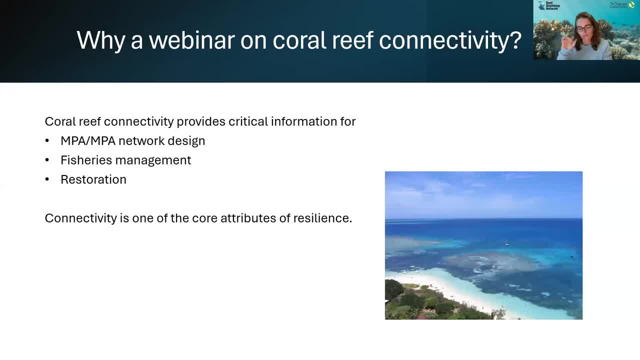 and it often seems like the holy grail for data for marine protected areas design. As we increasingly prioritize reef resilience and the maintenance of coral reef services, connectivity once again emerges as a critical focal point, both for the design and management of MPA and MPA network. 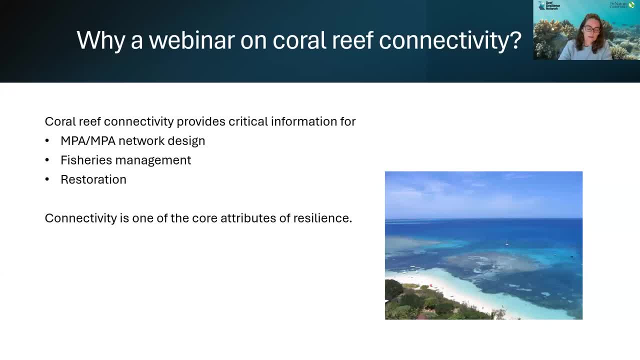 Serving as a cornerstone of resilience, connectivity plays a pivotal role in supporting coral reef structure and biodiversity and sustaining fisheries And, additionally, understanding connectivity provides crucial insights into where restoration efforts can yield the greatest impact, While connectivity can often be effectively understood through local and traditional knowledge, 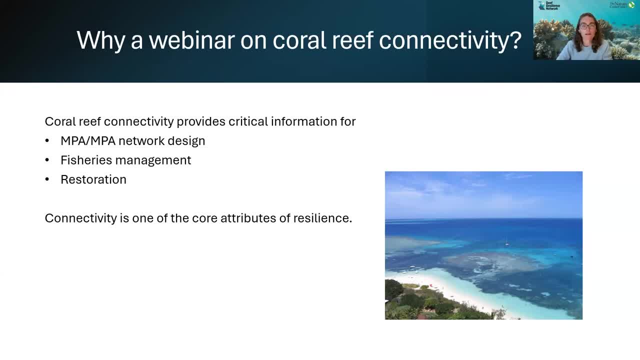 accessing information on connectivity remains a challenge for a manager. in the scope of their work, They frequently rely on scientists to gather or create the necessary data. However, this can lead to a frustrating process where the information provided by scientists may not precisely align with the management needs and where managers may struggle to fully grasp the potential needs. 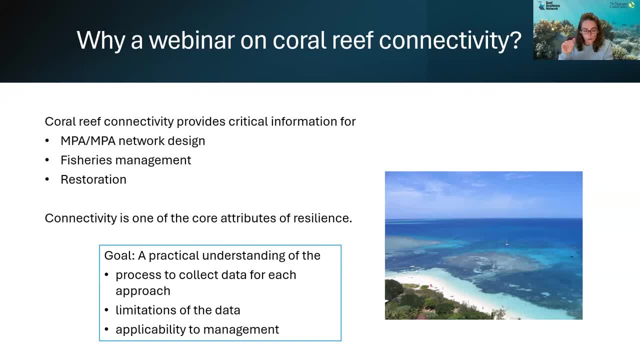 So the goal of today's webinar is to offer insight into two approaches to understanding connectivity. It provides a practical overview of the process of getting the data, includes questions that data can and cannot address, and provides a brief case study illustrating application of each of the management scenarios. 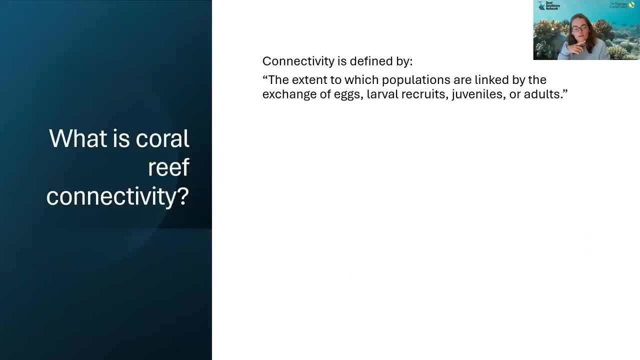 Next. So what is the definition of connectivity? So what is the definition of connectivity Defined by the extent to which population are linked by the exchange of eggs, larval recruits, juvenile or adults Next, And there's often two types of connectivity that are thought of. 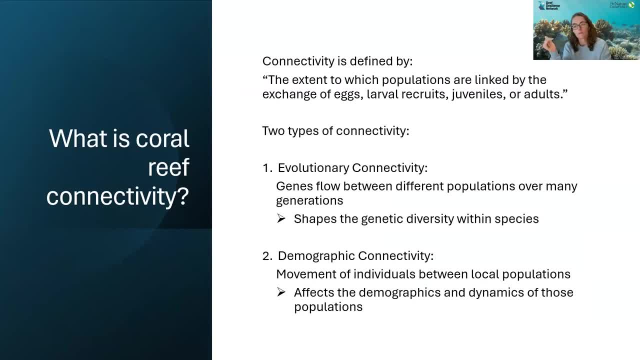 One is evolutionary connectivity, where gene flows between different populations over many generations and it shapes the genetic diversity within species. And the other one is demographic connectivity, where there's a movement of individuals between population which affects the demographic and dynamics of those populations. 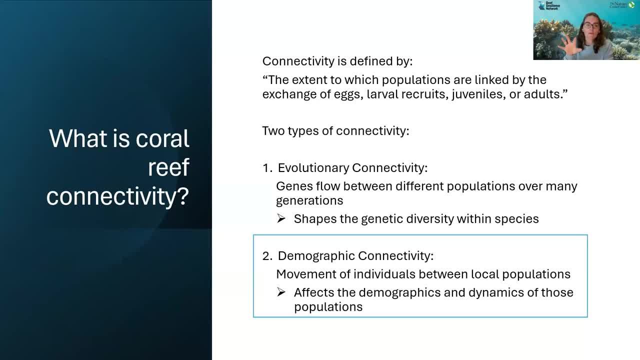 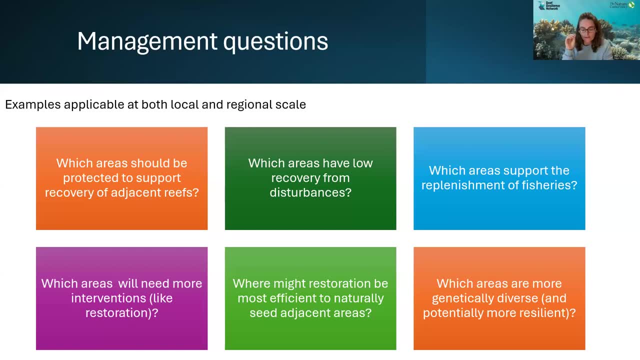 Next, And so for today, that's really what we're going to focus on Next slide. So studies on connectivity help answer common management questions such as: which area should we prioritize for protection? Which reefs act as important larval sources and contribute the most to resilience of the system? 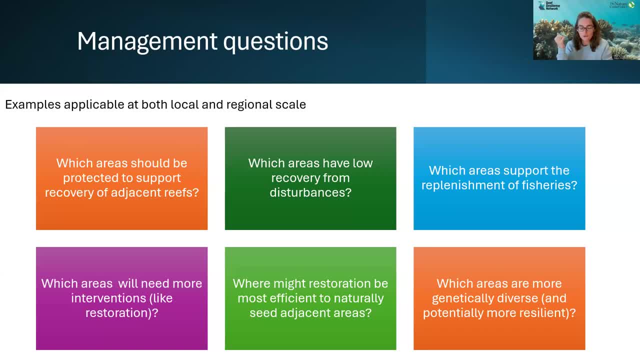 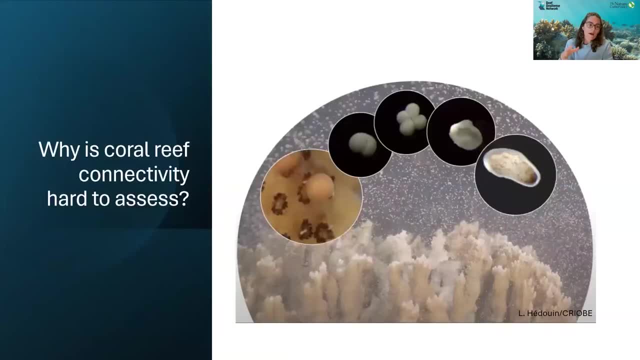 similarly for reef restoration- which are the areas where there should be outplanting to maximize the benefit to reef conservation, the benefit of restoration Next. So why is it so difficult to be able to answer these questions and assess connectivity? Well, most reef-associated species are stuck to the bottom, like corals, or are sedentary. 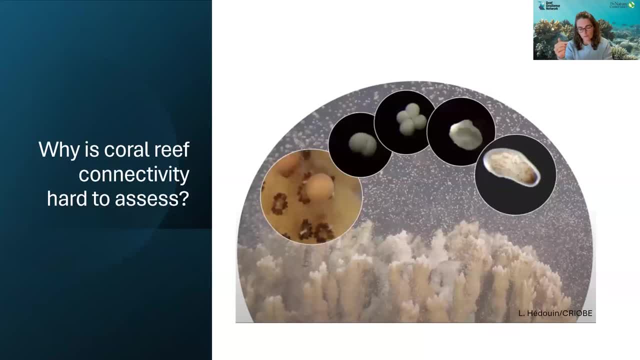 like most reef fish, Most disperse through their pelagic fate, which occurs during sexual reproduction, resulting in a pelagic larvae. This is particularly important because not only is it the opportunity to disperse, but it's the opportunity to disperse new genetic material that contributes to resilience. 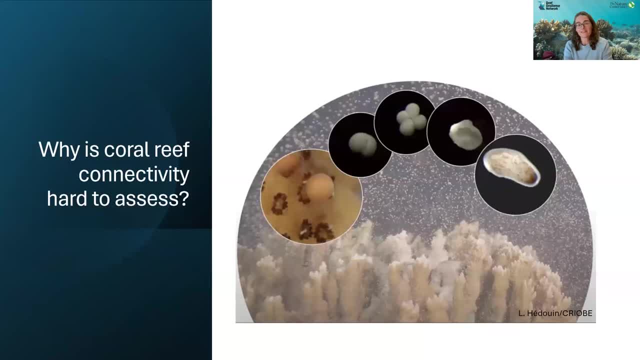 Unfortunately, that pelagic larvae of most marine species is tiny so it's very hard to track. It's difficult to assess the length of time it stays in the water column because it behaves differently in situ and in lab settings, And while many of them may be caught in common currents- major currents- we know that most. 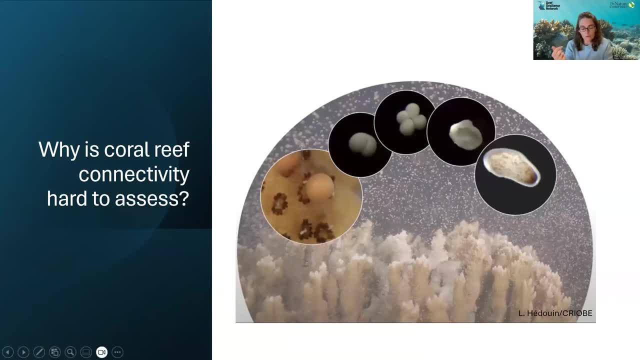 pelagic now can survive. They can swim, respond to cues to settle and control buoyancy So they can be caught around reefs in small eddies that will either retain them or make them flow counter-current-wise. So it's complicating predicting their dispersal pathway. 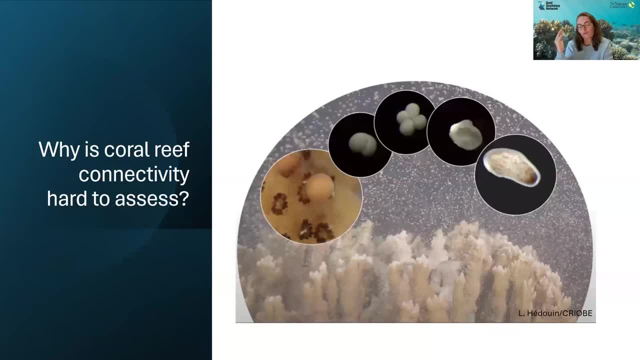 And additionally, there's thousands of larvaes produced during single dispersal events. so it makes it really difficult to track parentage And all of that translated, not knowing with certainty where larvae are. but it's really important to know how larvae travel and how they shape the reefs around them. 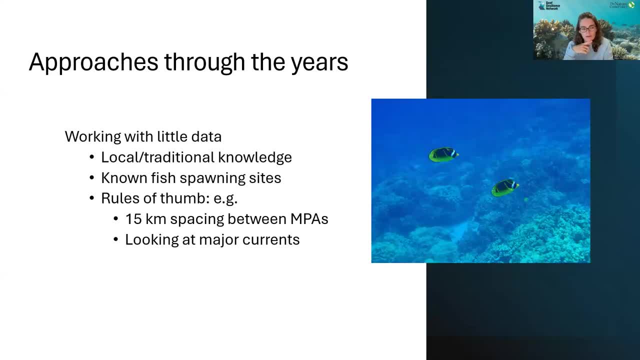 Next. So what have managers done without a lot of data? Well, one they've turned to local and traditional knowledge, looking knowing areas of recruitment or fishes knowledge of spending sites. Throughout the years, we've been getting more and more data. 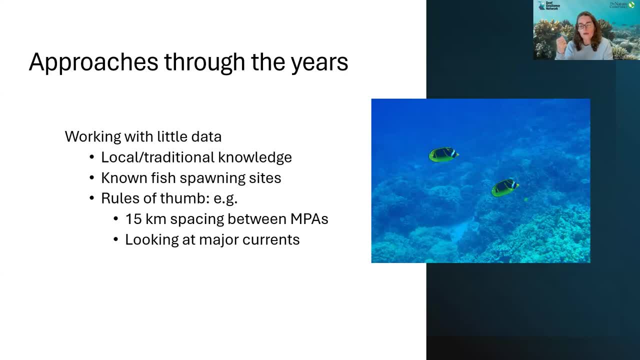 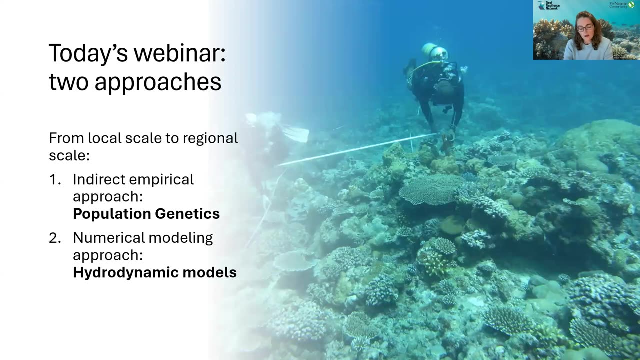 And so scientists have been coming up with rules of thumb, like the Mora et al paper, who'd done studies on connectivity, saying that 15 kilometers spacing between MPA was the most efficient, or simply looking like at major currents Next. But we've made a lot of progress since all of this. 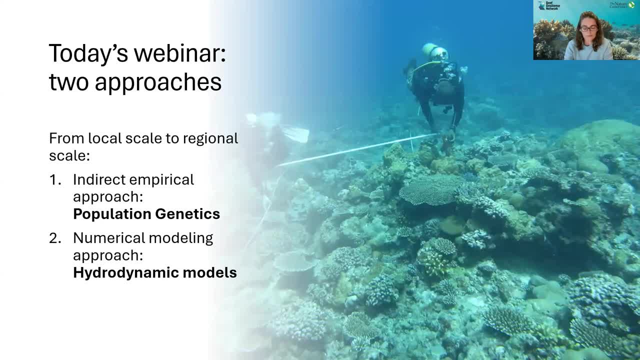 And so today we actually have two guest speakers who will be presenting two different approaches to connectivity, going from a local island scale, using population genetics, to a much broader regionial scale, using hydrodynamic models. So now we'll pass the presentation to Nicole. 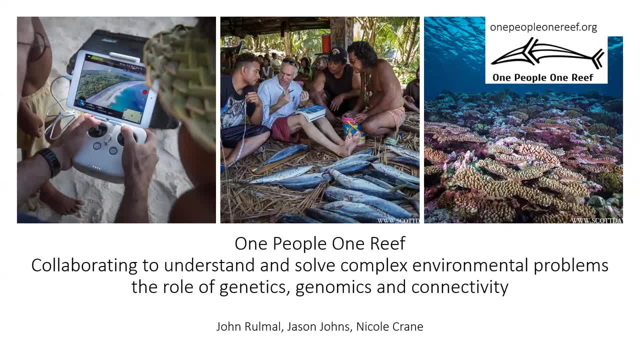 Thank you, Hi everybody. Thank you so much And thanks everybody for coming to the webinar. First I want to introduce colleagues of mine who I believe Magul John Rumal is here. I'm not quite sure who's really the person who's sort of supported all of this work on the. 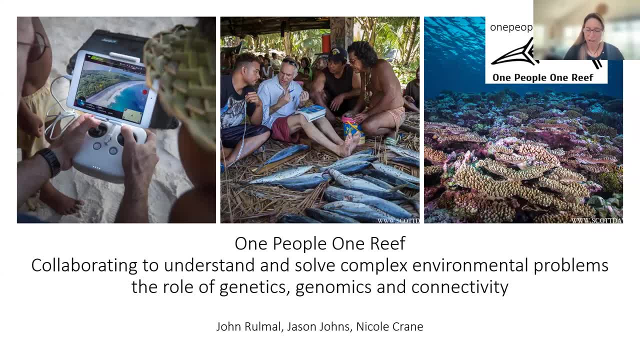 atoll of Ulithi in Yap State, where we work. Dr Jason Johns will be speaking with me today. He's our postdoctoral researcher, with One People, One Reef, Splitting his time between University of California, Santa Cruz, and University of California. 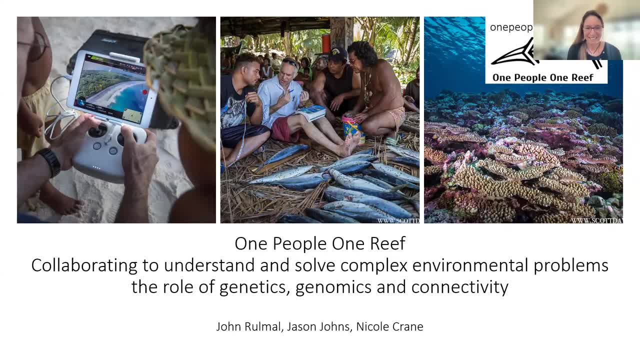 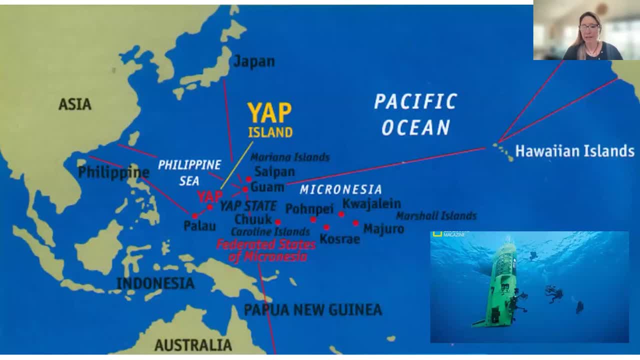 Santa Barbara and in the field with us, of course, in Yap State Next. So I'm just going to start, before I get into anything here, by thanking the people of Yap and Ulithi Atoll in particular for sharing their remarkable story with the world. 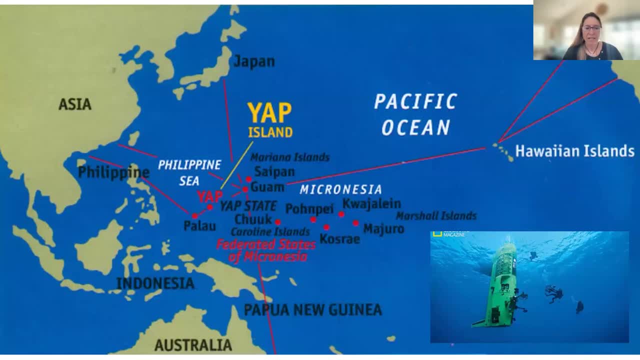 They have opened their ocean, their houses, their islands to us and have worked very, very closely with us in solving- first identifying and solving- some of the management challenges that they've had Over the years. We've been working there for a little over 10 years now and they're just remarkable people doing. 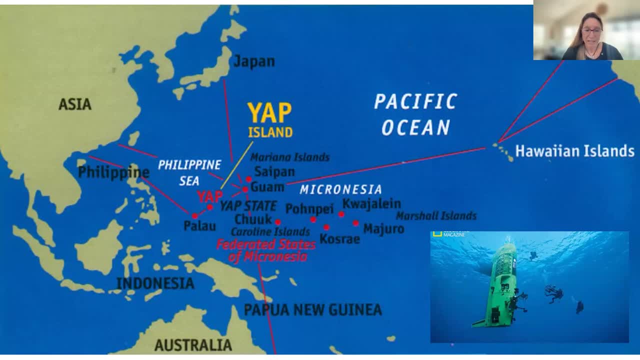 amazing things, And so I just want to thank them before I go on anymore. Just to situate us here: where we work is in Yap State, which is south of Japan, east, just east, and north of east and north of Palau. 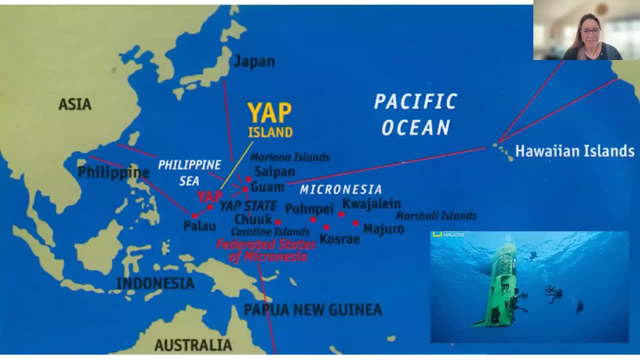 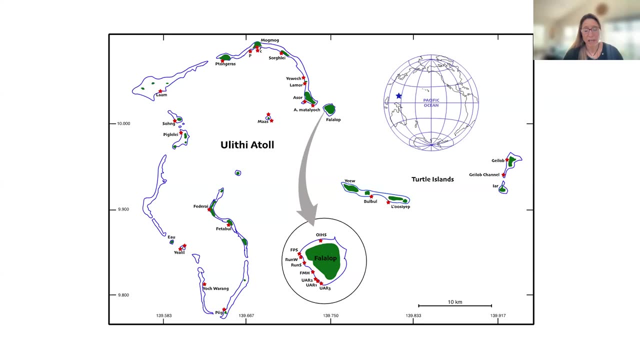 It's one of the four states of the Federated States of Micronesia. Next Yap consists of many, many outer islands. It's a vast archipelago. It's in a giant, otherwise empty, West Pacific Ocean. It's a real conservation opportunity and a place that has been understudied and under-resourced. 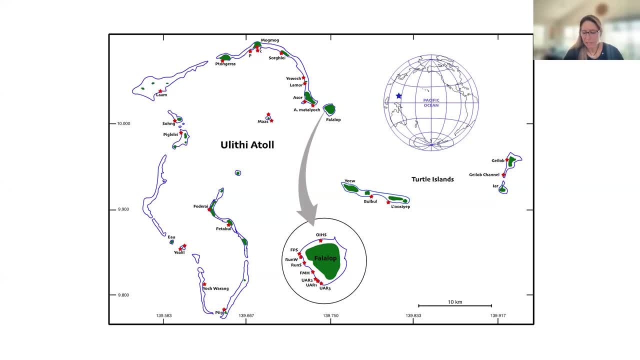 We've done most of our work on the atoll of Ulithi, which is approximately 30 kilometers long and about 16 kilometers wide, inside the lagoon, about 580 square kilometers of ocean. It's the fourth largest lagoon in the world. 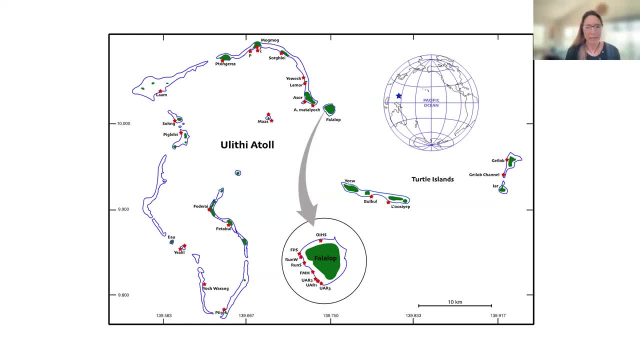 So I just want to point out here, just to situate you, because we're going to be coming back to this map, in the north You will see- maybe you can't read it- Mogmog and Aesor and Falalup, And these are inhabited islands, as is one to the south here called Federi. 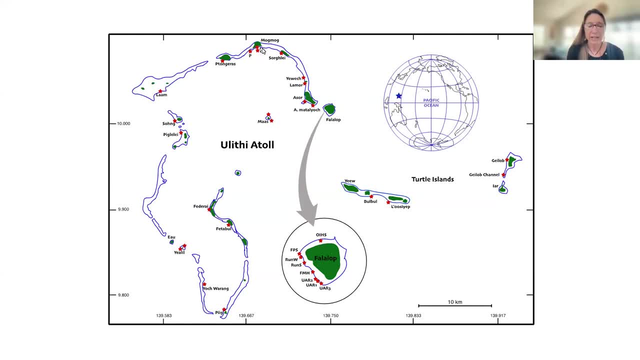 I don't know if you can see my pointer or not. So there are four inhabited islands in this otherwise giant atoll And we're going to be talking a bit about how the reefs are very different in the different parts of the atoll. 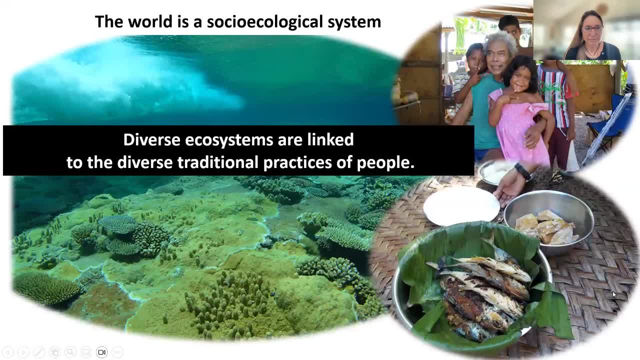 Next. So I want to just bring us back here to a people-centered approach to management. All the work that we do is led by the people of Ulithi and Yap. The world really is a socio-ecological system and the diverse ecosystems of our planet are really linked. 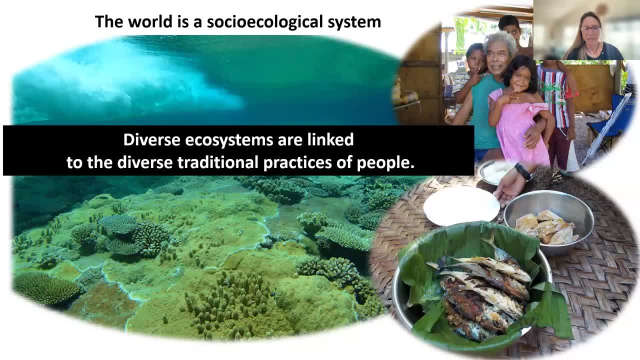 to the diverse traditional practices of people, And as we lose those traditional practices, we also lose some diversity. There are consequences to that. So our work really centers on traditional practices, while understanding the need for adaptation in a changing world today, both with climate change and with socioeconomic changes. 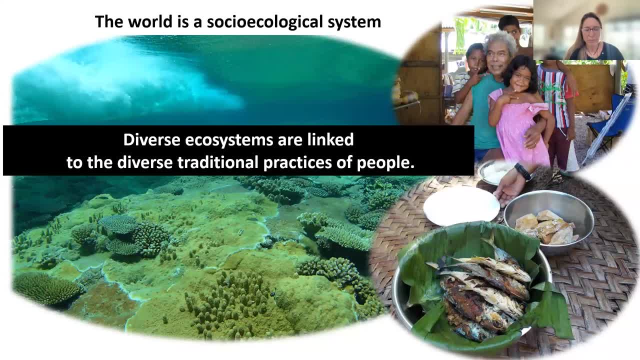 So we're aware that it's not a fairy tale. We're also aware that people can't always rely on only traditional systems, because the world's a different place. But connecting those things stands to reach a lot more people and achieve a lot more success. 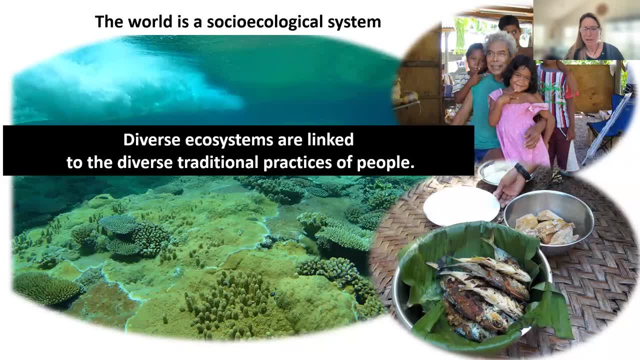 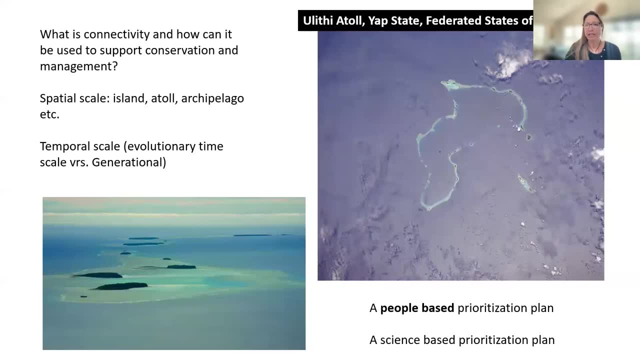 If we don't put people at the center of some of these initiatives, they stand to not be nearly as successful Next. So we'll talk a bit here about connectivity and what it is, And I'm actually going to present here a couple of different types of approaches that we've used to connectivity. 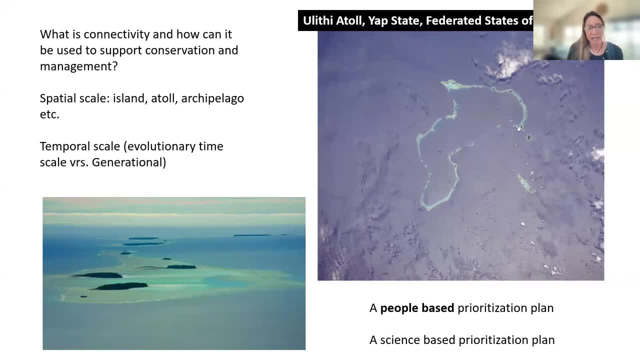 We can do different spatial scales, as Anik mentioned: an island, an atoll, an archipelago, depending on what you're using- And Courtney is going to be talking about some of the larger scale approaches using currents- And then also there are different temporal scales, whether you're looking at evolutionary time, as Anik mentioned, or sort of generational time. 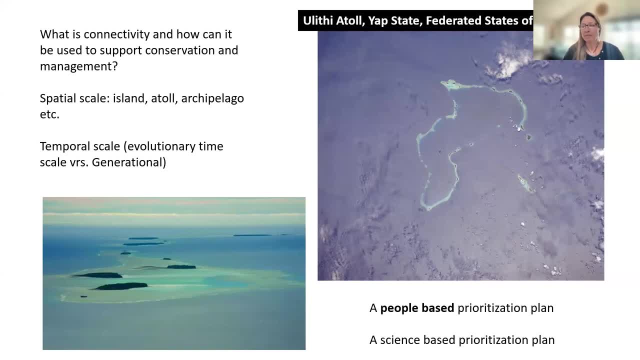 And I think all of these connectivity studies are really based on what managers are trying to achieve in the work that they're doing, What we can say in some cases and what we cannot say, for example, in the work that we'll be producing. 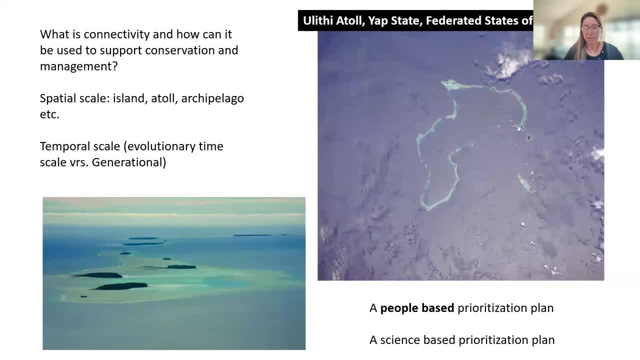 Today we cannot really talk about directionality. In other words, we can say north-south, We can't say from north to south or from south to north. Managers might have a goal to see how sort of healthy reefs might impact less healthy reefs or vice versa. looking at resilience, 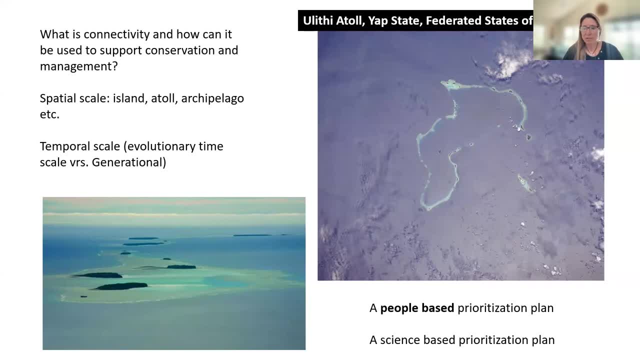 They might be interested in reservoirs or sources of healthy corals to, for example, seed or populate places that are less healthy or may have bleached, And in our case, we're very interested in how management can be connected Between jurisdictions. 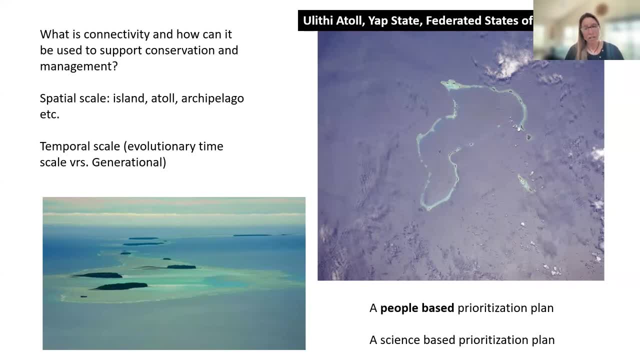 Sources and sinks are important to identify, but those can also change as physical parameters change: Species get introduced, reefs get degraded, currents change, So those parameters can change, And so the context of the work also needs to be taken into consideration. Those are all science-based prioritizations. 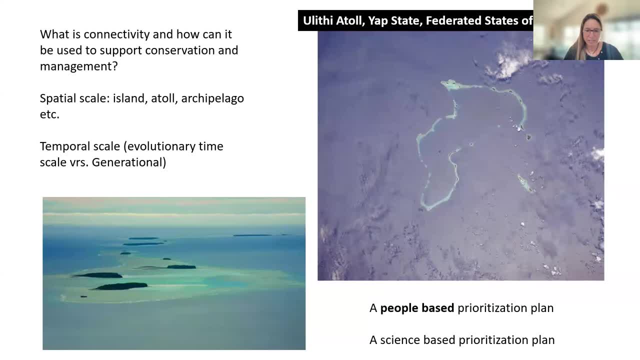 And I'm just going to point us to that lower statement there- a people-based prioritization plan, because that's what we're using. So we're asking the people first about what they're most interested in and what they're most concerned about. 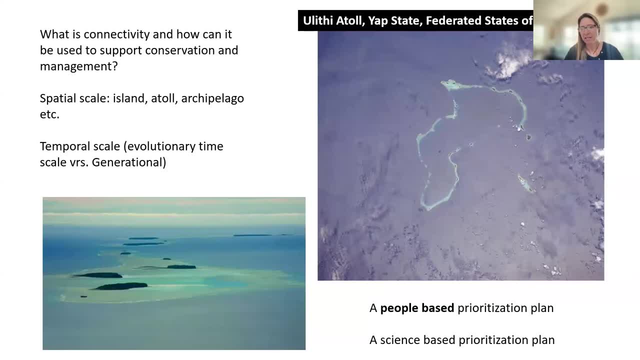 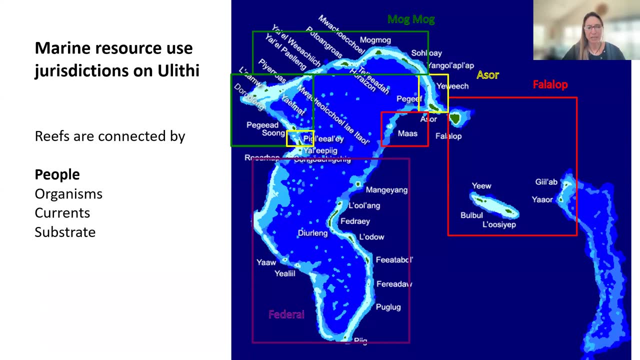 And then we're going to put that on their reefs so we can put it into the context of what they most need. Next, This is a map here. This is the reason why I don't want anything to do with developing these management plans. 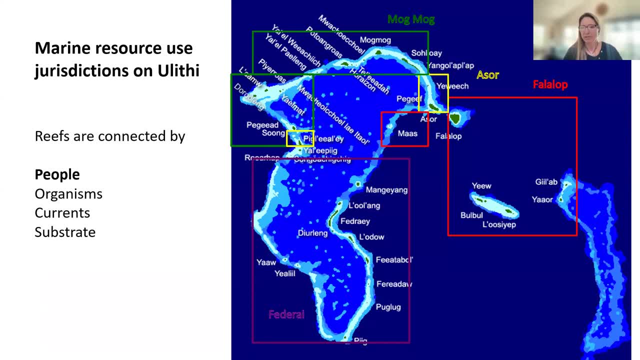 This is the jurisdiction clan jurisdictions of the reefs of Ulithi. They're extremely complicated, They're based in a vast and complex history And for me to come in and say, well, there should be an MPA here or an MPA there based on the science, is really going to be counterproductive. 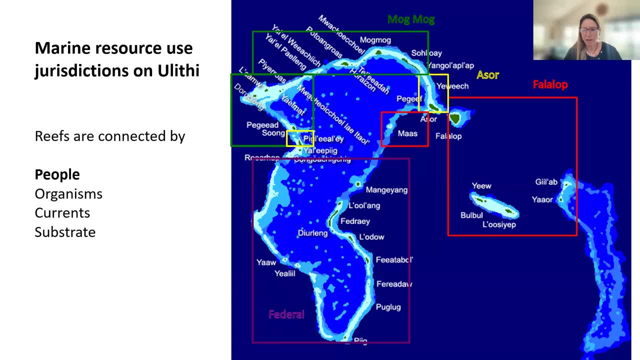 Because the management system and clan jurisdictions are what drive this And in Ulithi, as in many Pacific Islands, those jurisdictions and the management itself is very socially based. It's based in a deep social foundation, not really a direct biological or ecological foundation. 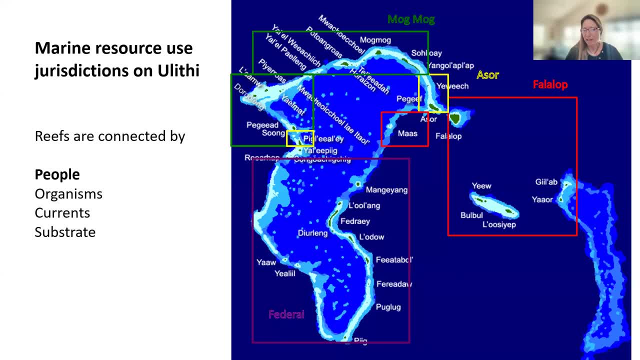 So if we come in and try to present that perspective, it's not going to do very well when you're trying to talk with people who are really much more socially based in their management. However, if we can overlay our ecological map, let's say, and the data we're collecting, with the social one. 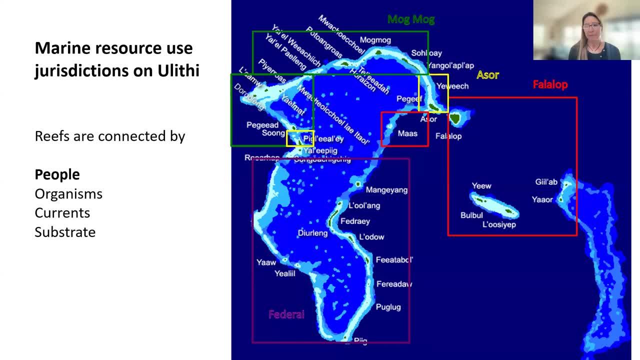 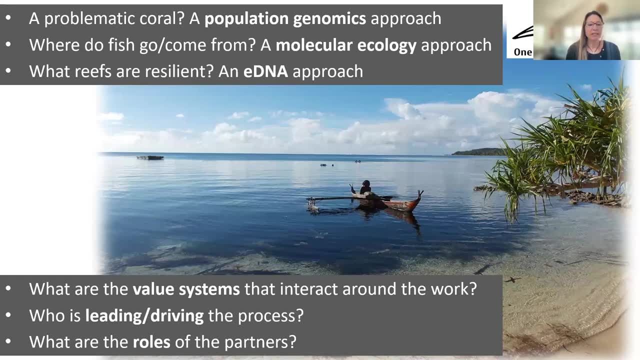 it does open up new ways and new insights into the importance of adaptive management. So that's really where we are with our work Next. So we're going to talk about three things here. a problematic coral. So one of the first things that the people mentioned to us was that there was a coral that they were worried about. 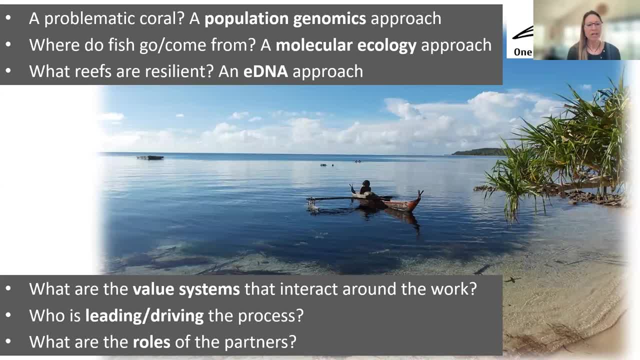 So we're going to talk about a population genomics approach to looking at that coral- Where do corals and fish go? and come from A molecular ecology approach, And then I'm going to finish up with a brief introduction to our brief conclusion as to how we're using DNA. 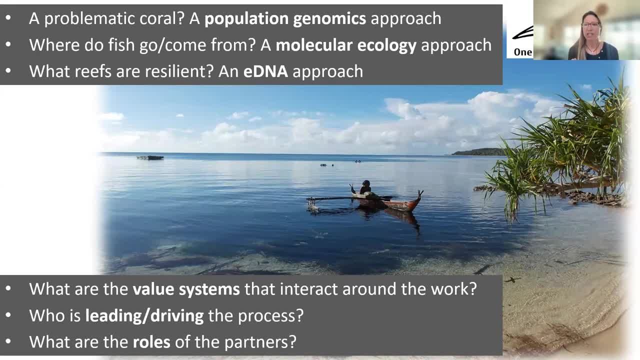 So just a little bit of context here. Remember, genetics really is the study of genes, things like heredity contributing to disease. Genomics is a much newer approach due to much better computational power and technology that we have today: Studies of the whole genome, how genes are related to one another. 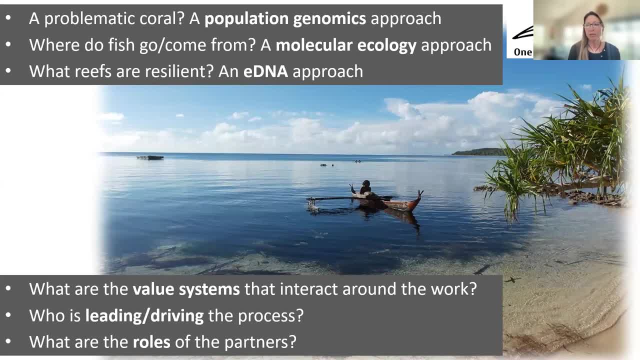 how genomes change over time. Population genomics, then, can determine gene flow and migration, looking at average movement of individuals over many generations. So we can look at how populations change, which can give us some insights into how they're changing, for example, under climate change regimes. 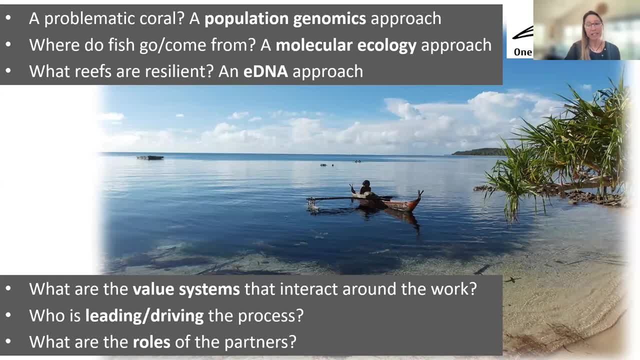 However, those tend to be over longer time scales. We can also use molecular ecology, using a more forensic approach, to look at parentage, for example, or kinship analysis, which is what we did here. So looking at who on which reefs are related to who. 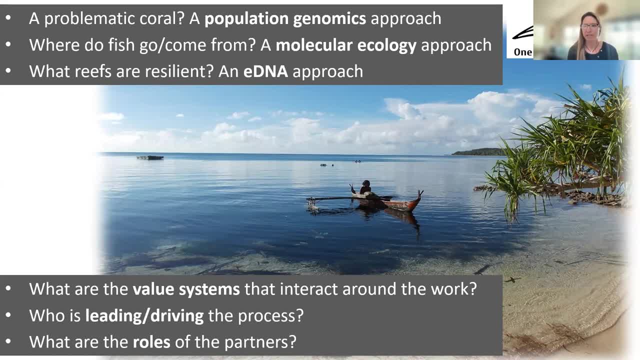 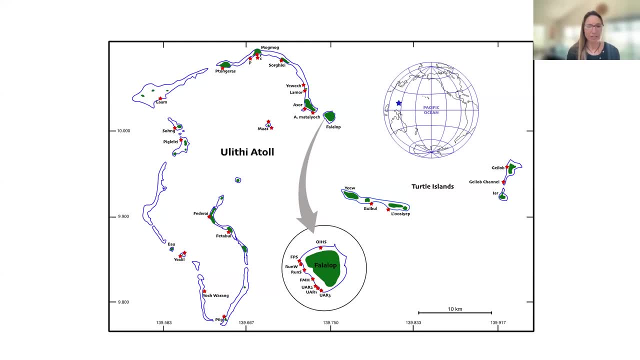 so you can see where they might have come from. So that's sort of the source and sink piece Next. So back to this map. I just want to point out that Ulithi has very different reefs, And so those northern reefs up there are very different than the western reefs on this map. 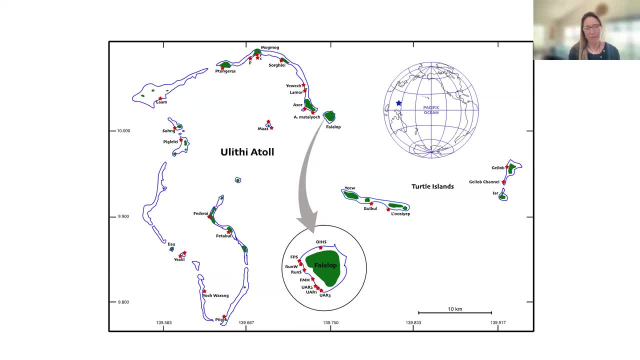 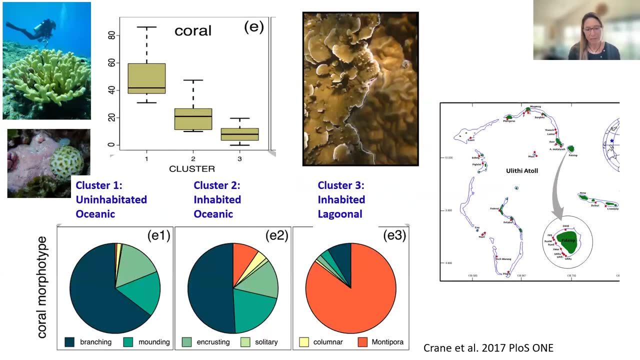 So I'm going to show you some pictures here and relate them back to this map of the atoll Next. So you'll see three circles down at the bottom. The one on the far right, this mostly orange, are the reefs that are at the top of Ulithi Atoll. 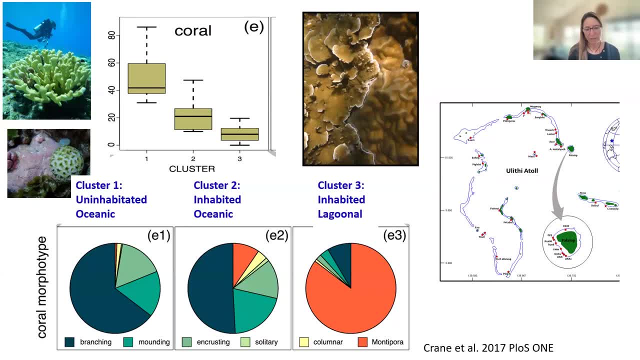 for the most part where people live so close to the villages. And that orange color is Montipora Capitata, or a close relative thereof, And it's growing in a very weedy fashion on those reefs, overtaking other corals. 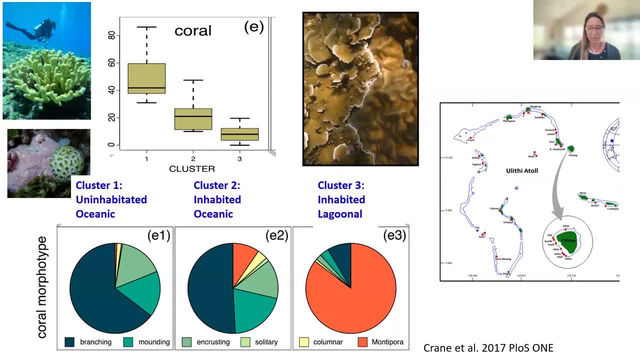 creating a mono-specific reef. that fish don't tend to like, So this is problematic for people. Although there's lots of coral, it turns out to be a problem: coral In the middle. there you see reefs that have some of that: Montipora. 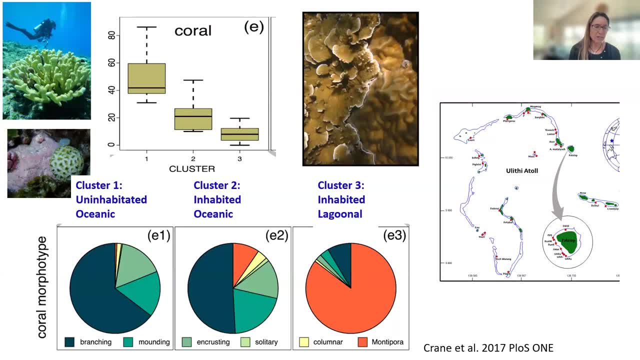 but they've also got much more diversity And on the left circle we see much more branching corals, so really healthy reefs, mostly on the western side of the atoll Next, And the fish biomass mirrors that. So in those healthy reefs, 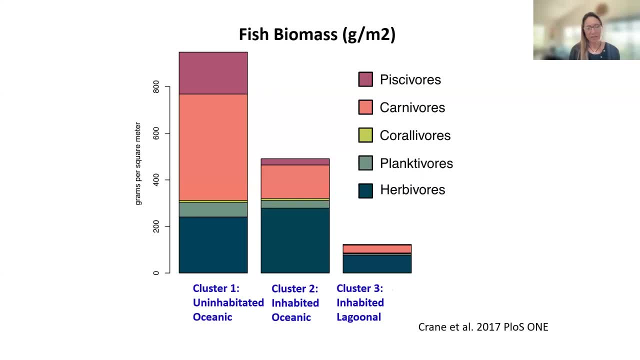 you see cluster one, lots of fish In the less healthy reefs. cluster three, we see much lower fish. So I'm showing you this just by way of saying that we characterized these reefs before we started looking at connectivity to better understand the differences. 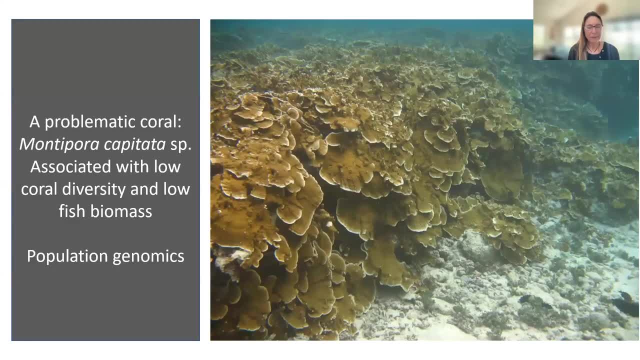 in the reefs that were there Next. So here's Montipora and you can see that it has taken over this reef. The people don't like it. It tends to drive fish down. It also takes away octopus hiding holes. 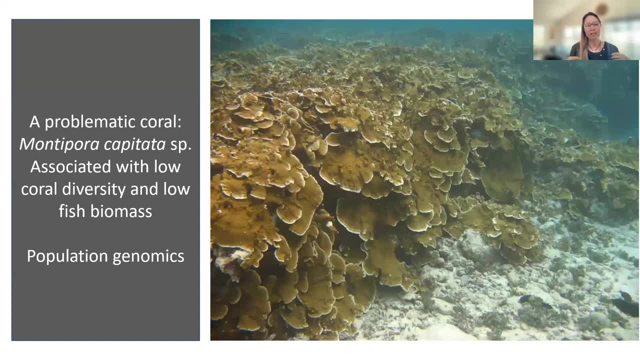 So we decided to take a look at this, and you might want to consider doing this, for example, after you've done a connectivity study, to look at what reefs might be connected to others, and then target on either a problem organism or maybe one you want to learn more about. 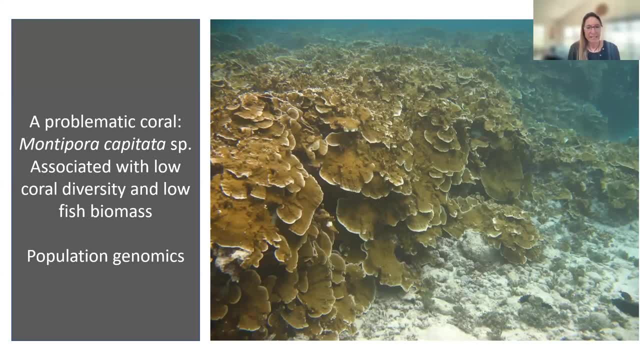 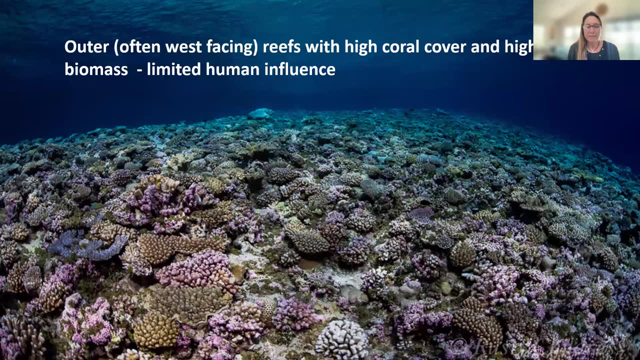 We focused on this problem, organism Next. So initially this coral seems to grow crazy weedy in those northern sites. This is the western reef and you can see how diverse these corals are from those western reefs. There is that same Montipora here. 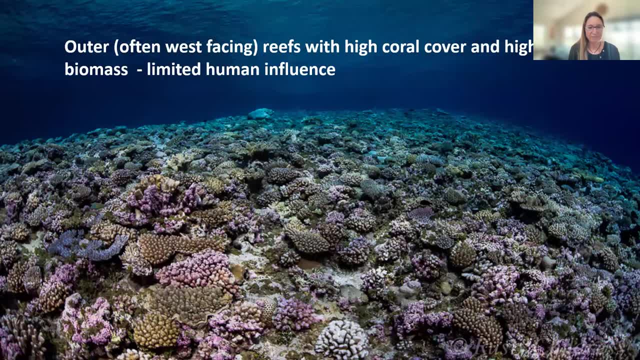 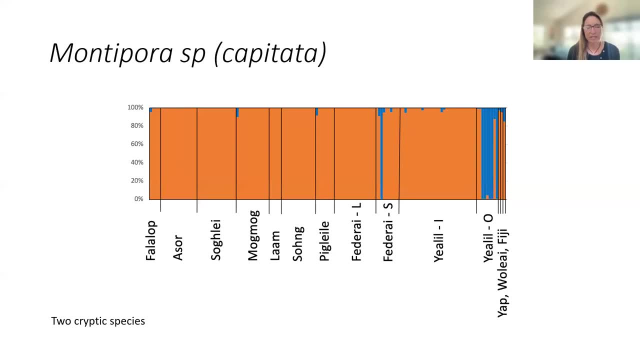 but it doesn't behave the same way, So this was really interesting to us. Next- So this is the first thing we did was to see if the Montipora in these different sites was the same species, because corals can be so plastic. 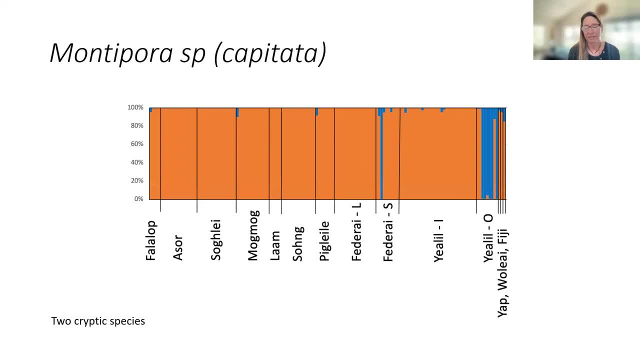 and it can be sometimes difficult to detect differences, And you can see the blue is one species and the orange is another. So there are two cryptic species that we found out there, although the orange one is far more common and that's the one we focused on. 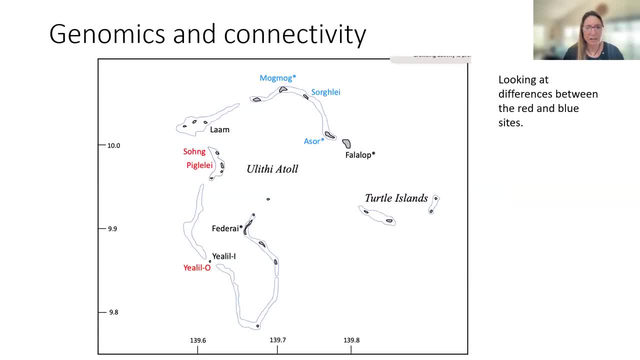 Next And you can see the blue sites. there are those sites that are in the north compared to the red sites on the west. So we wanted to compare those more pristine red sites with the really degraded and Montipora-dominated northern sites and see if we could find differences there. 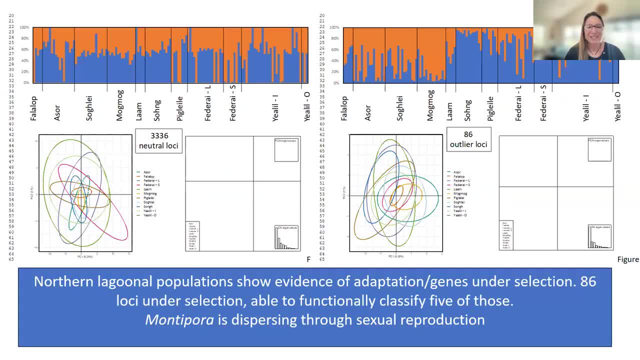 Next And differences we did find. So this is a complicated figure. I'm not going to go into a lot of detail, but I want to point your attention to the left side, on the top And you can see there isn't a lot of population. 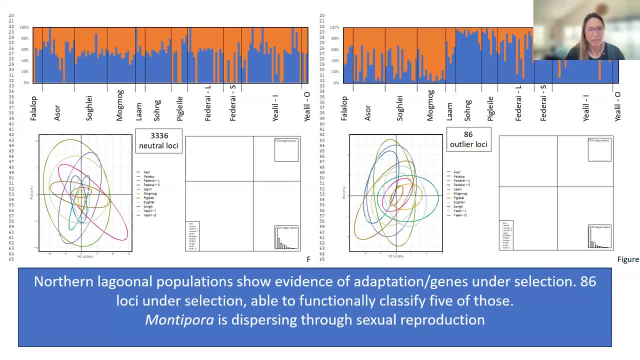 structure at those different sites. So those are all the sites laid out there, from Fulalip to Yalil. Not lots of population structure that we could find. However, on the left- sorry, on the right side- we do see that there were evidence of adaptation. 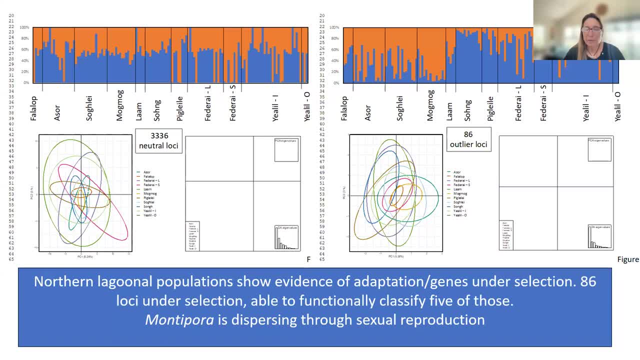 Eighty-six loci were under selection and we were able to functionally classify five of those. So you'll see that on that figure, on the top of the right, on the left side of that figure, there's more orange than on the. 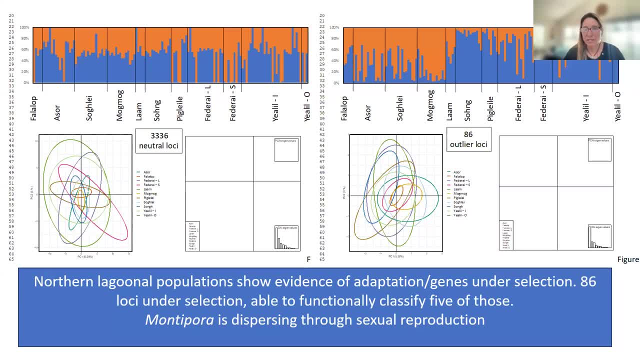 right side of that figure. So we saw definite differences and in fact, those sites that were in blue in the north part of the lagoon, with all that Montipora growing like crazy, that was the stuff that was under rapid selective pressure. 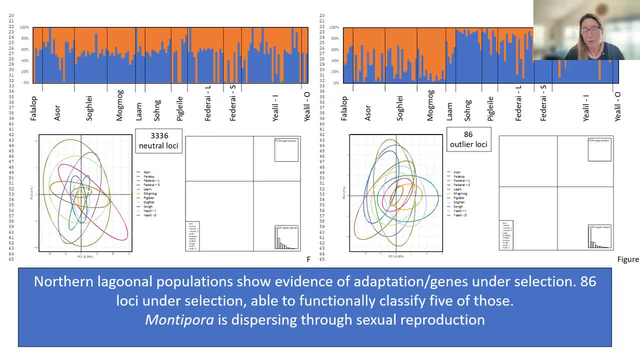 So our we consider, possibly, that those populations are responding actually quite well to climate change or to otherwise what we might consider unfavorable conditions. So there was a concern that those corals might move around- the bad ones, let's say- And start dominating in other sites. 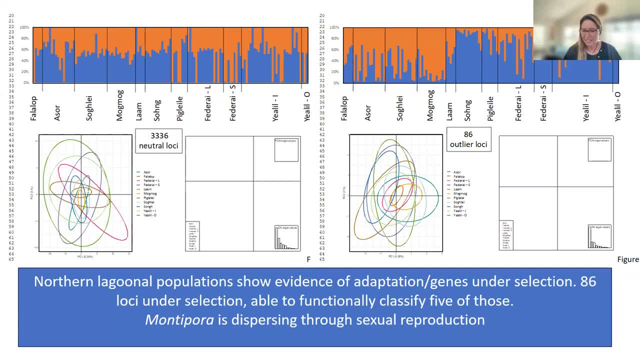 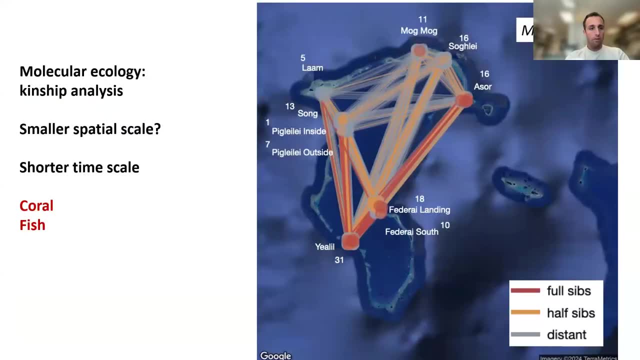 So here's where connectivity becomes important, So I'm going to bring Jason in here now to talk about his connectivity graphs. All right, Next slide, please. So we can do that kinship analysis that Nicole's been talking about by sequencing the genomes of a bunch of different individuals across the atoll. 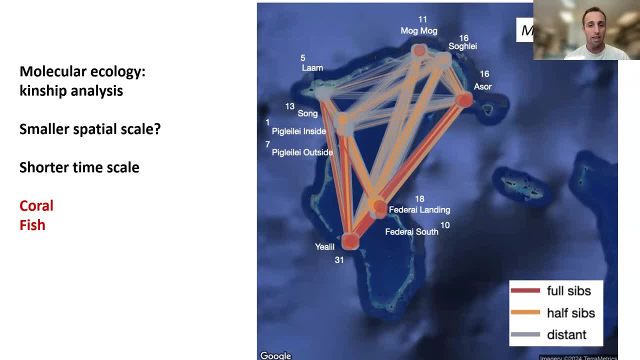 which is getting cheaper and easier to do by the month. So when we sequence all these individuals, we can compare each individual to the others in the population, determine their kinship and put that on a map to show connectivity. So are they related enough to assume that they're full siblings? 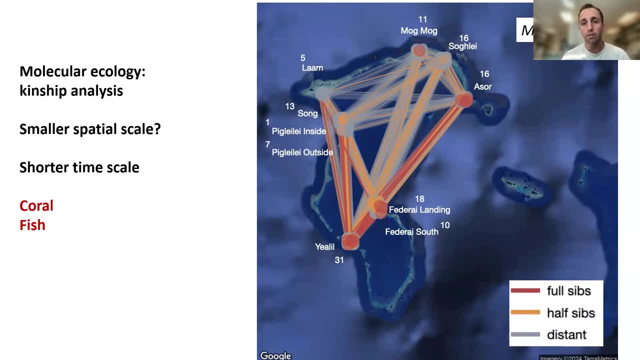 Are they just half siblings or are they unrelated? And so these dots and lines here are showing those relationships. The dots are relationships between individuals from the same island and the lines are connecting individuals from different islands, And so the red dots and lines are showing full sibling relationships. 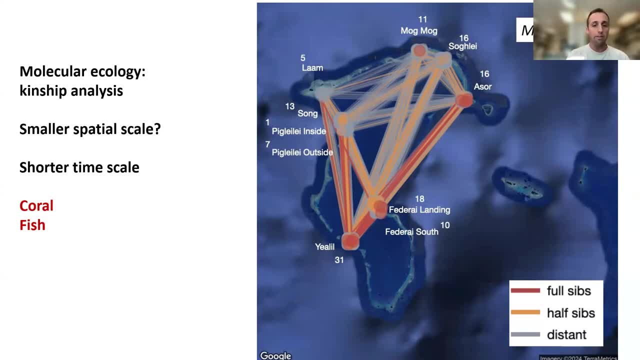 the orange half siblings and gray distantly related individuals. So here we're looking again at that invasive coral species, Montipora, And interestingly, here one of the first things we notice is that islands that are close together aren't necessarily the most connected. 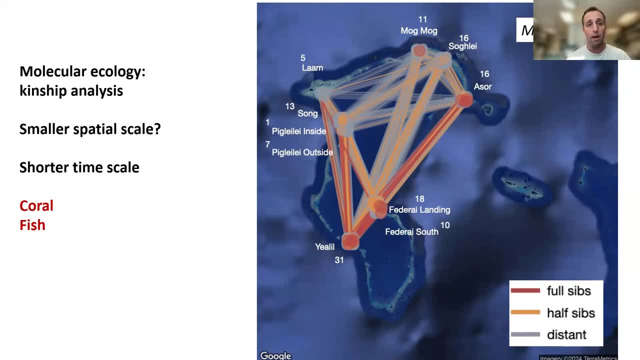 We see high levels of connectivity from north to south, even from islands that are really far apart, And so one of our fearless leaders that Nicole mentioned, Magul Rumal, who's from Ulithi, was really excited when he first saw this map. 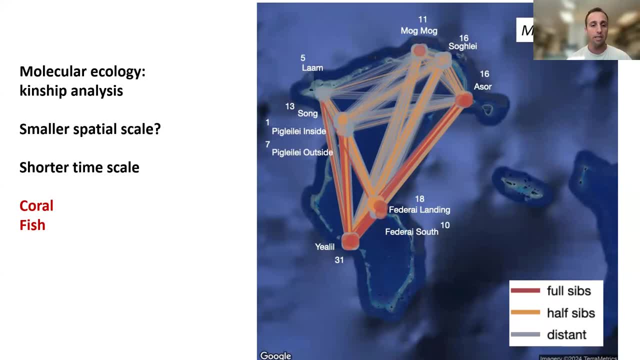 because it turns out that these patterns of genetic connectivity really parallel traditional patterns of social connectivity. So it turns out that these islands are co-managing their reefs on multiple levels and we're able to visualize that with these data. So for a species like Montipora that stays in one place, 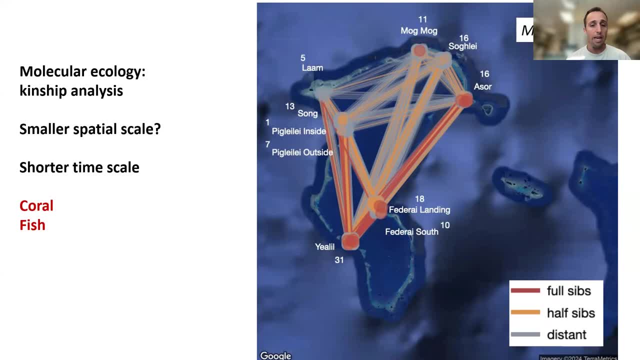 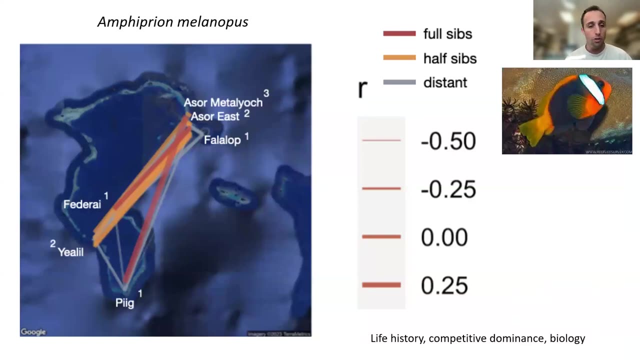 these patterns are largely driven by currents, but it may have to do with dynamics of adaptation and competition, which is where the analysis that Cole just discussed can come in handy. Next slide, please. So we can do this for fish, too, and this clownfish species. 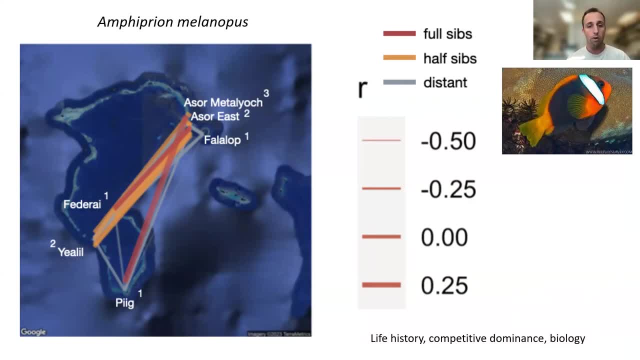 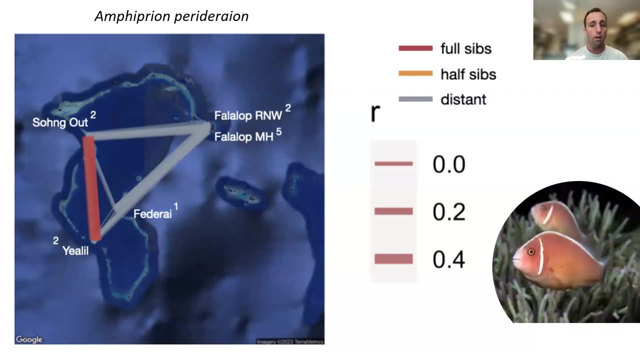 we see a similar pattern to what we saw with the coral, similar to Montipora, where they disperse at the larval stage and then stay put and we're seeing some strong connectivity from north to south. On the next slide we see a slightly different pattern, with a closely related 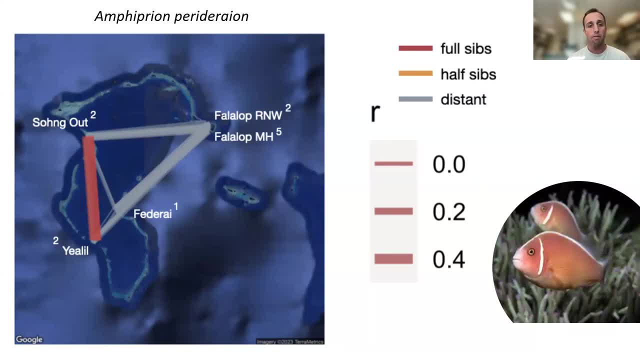 but different species, and this is where we can start to potentially visualize dynamics of competition and habitat preference. So if a particular island is not connected to other islands, it can be due to various factors, but one of those factors can be due to a low adaptation to a particular site or high levels of competition. 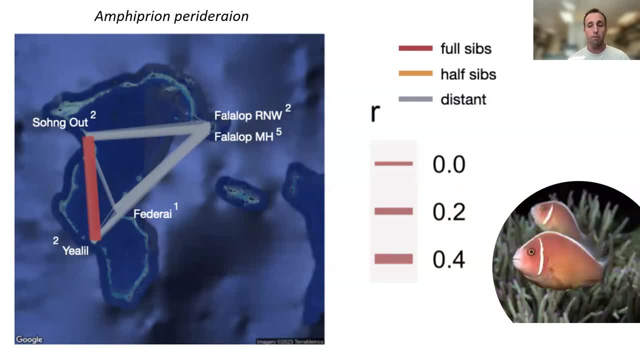 So coral or fish larvae can recruit from outside the atoll, but if they're poorly adapted and or out-competed, then they won't reproduce and thus they won't disperse offspring to other islands in the atoll, and so each one of these recruitment events will be independent from outside the atoll. 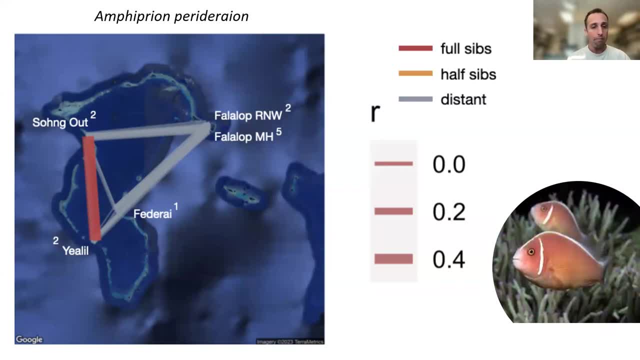 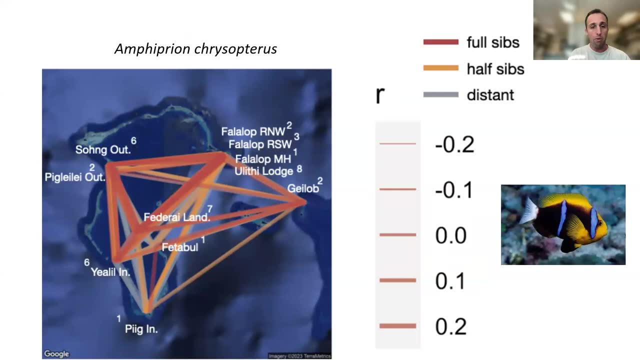 And this is the kind of thing that we can start to visualize with this map Next. So this species shows high connectivity across the atoll with a pretty different pattern than what we've seen before with Montipora and the other clownfish species. 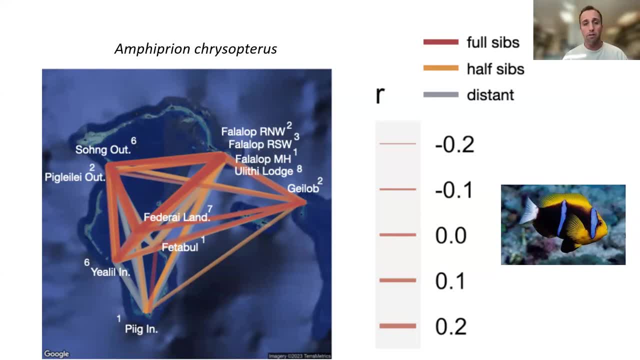 and this shows the importance of sampling different species with different dispersal methods and different life histories across the atoll. This can also be done for pelagic species. We're showing this for species that stay put the rest of their life, So importantly too. 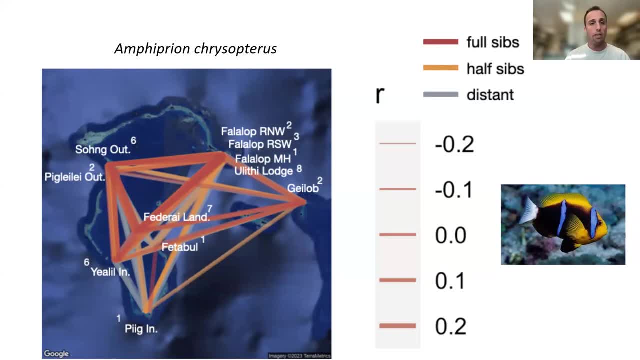 directionality isn't inherent in these data. right, We can say that they're connected from north to south, but we can't say that they're coming from the north to the south source to sink. but this is something that we can account for if we know something about the age of the individuals that we're collecting. 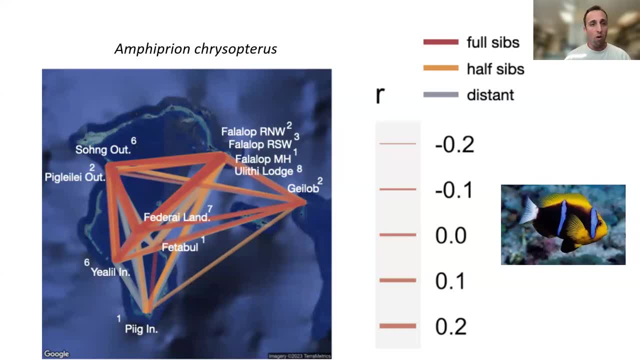 So we're showing these maps from clownfish and corals, but there's a lot of fish species that are really important to eolithians and as we speak, my background is blurred out, but I'm in the lab right now generating those data at the moment from some fish species that are really important to local people. 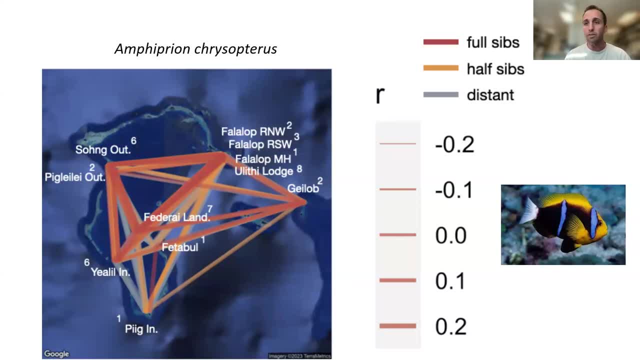 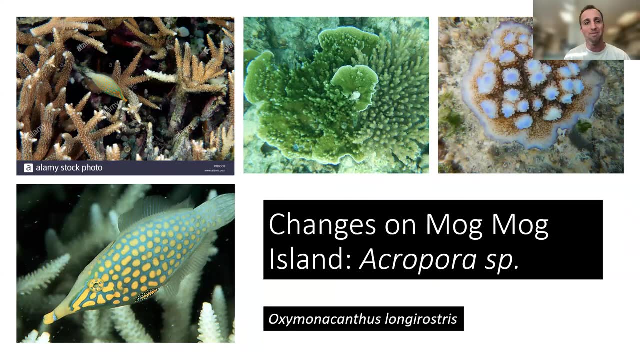 And now we'll pass it back to Nicole to talk about some resilience. You're muted, Nicole. Just a really brief foray into resilience. We have this one reef here in the north of the lagoon that was highly degraded and highly damaged. 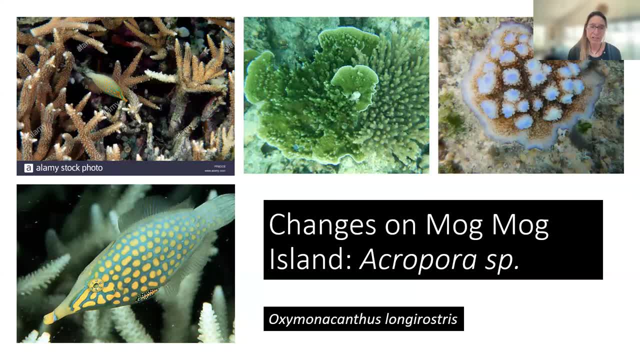 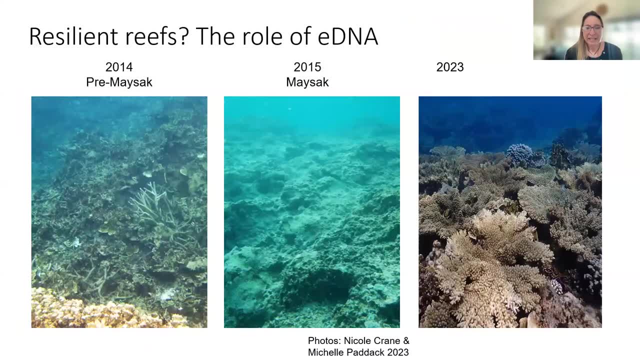 and we started to see a coral-dependent fish show up there and a recovery of some of the corals and this sort of amazing resilience happened Next, And so we wanted to try to understand what was happening out there. We suspect the corals are coming from some of those really pristine western reefs. 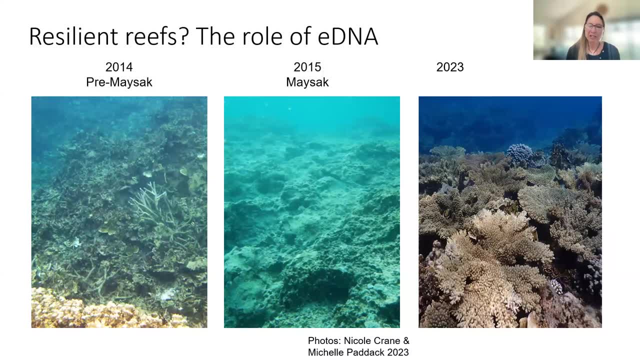 We don't know. there's some connectivity between those. So we decided to look at some eDNA, which is a really relatively fast and inexpensive way to look at biodiversity, to get a site. So you can see there in 2014 and 2015 how degraded that site was. 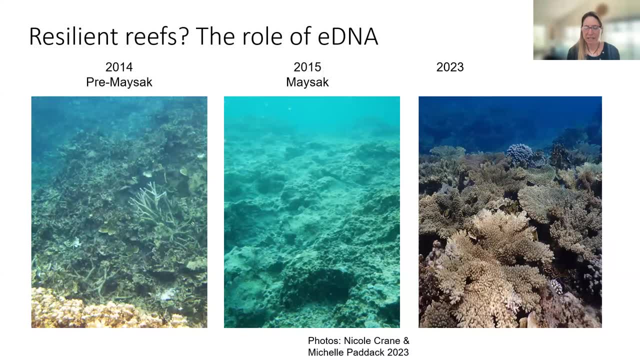 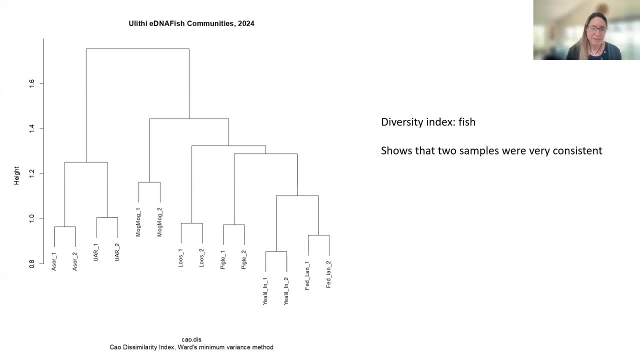 and by 2023, and it happened literally in three years. what happened to that site Next? So in the eDNA, it's really fast, easy. Jason actually collected it: Take a liter of water and filter it and ship it off. 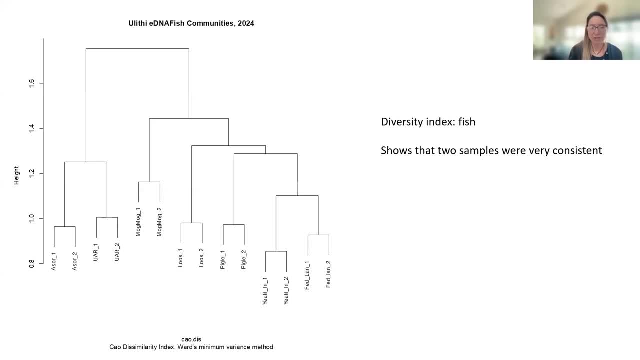 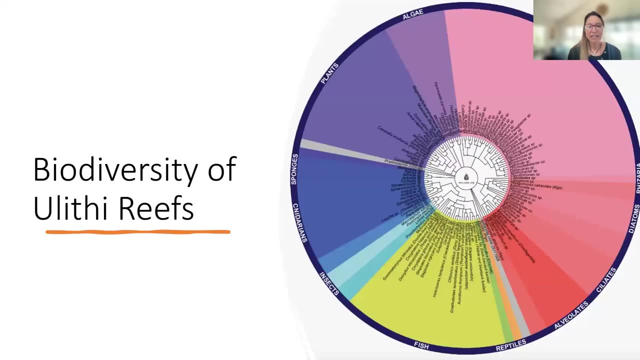 and you can see. we did two samples per site and the samples came out the same. So this is just showing you consistency between the samples. So our sample size was small and not so expensive. Next, And what you get is a beautiful colored circle of all the things. 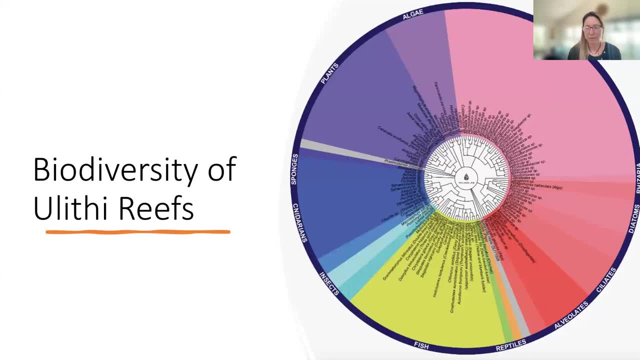 that you can find at the different sites, And so this is just one piece of the analysis, but you can really take a look at how these sites differ or are the same across space, And you can also do it across time, So this is really a good indicator. 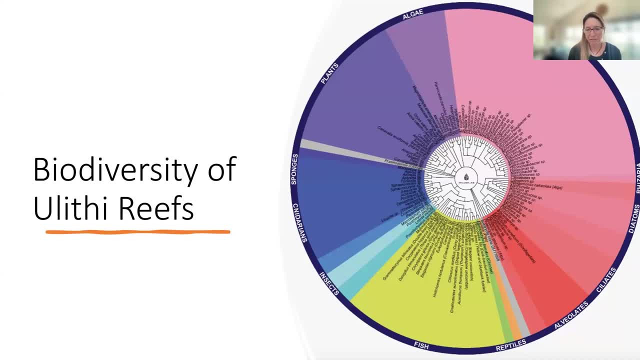 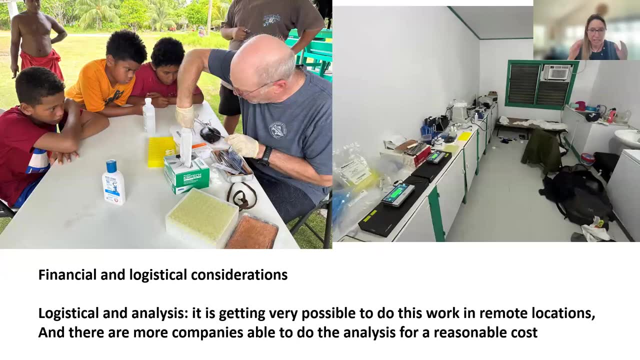 along with connectivity, to take a look at resilience and what might be happening on the reefs through time. Next- And I want to just point out that the financial and logistical considerations are getting easier- This is Giacomo Bernardi. He set up his molecular lab there. 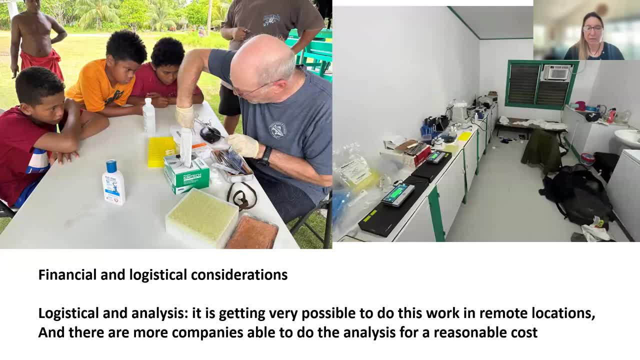 in the infirmary on the island collecting his samples, and he sequenced genomes right there in the infirmary. So the logistics are getting a lot simpler and the costs are coming down quite quickly. Next, I'll let Jason go through this. 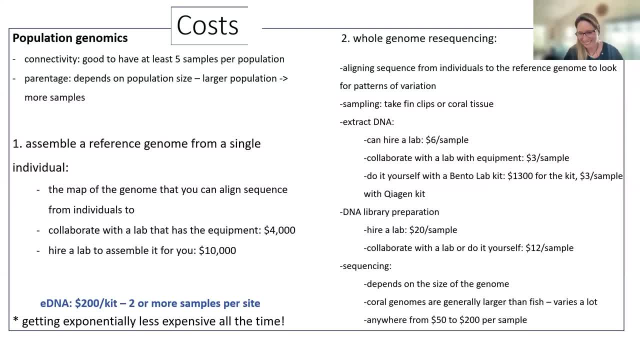 It's kind of a long slide, but we can do it really quickly. Yeah, so we put together a general list of procedures that go into these analyses, what they cost to do. So I won't read these to you, but we wanted to put this together. 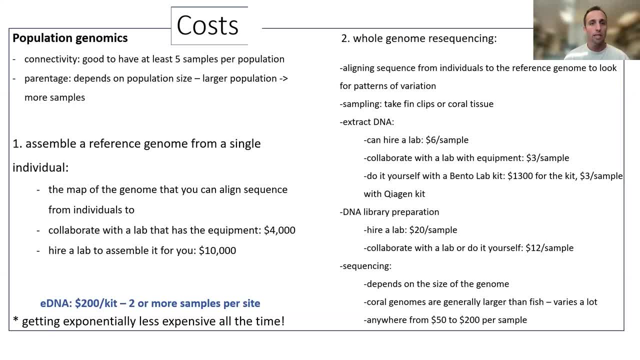 because this slide deck will be available after the webinar. Just to point out: generally, as with most things, it can be cheaper to do it yourself, but mostly if you have some of the tools and are already set up to do it, And so that's where collaborations with labs 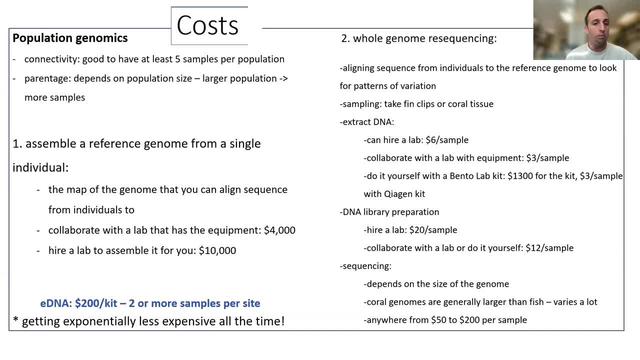 that are already set up to do this work can come in handy. These make for great projects and funding sources for graduate students For a term or two. I can speak from experience. But again, these numbers, they change really quickly and they always go down. 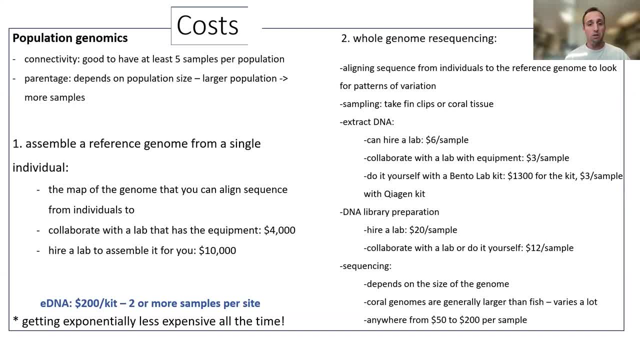 And so it's becoming more and more feasible to just collect the tissue and send it off to a lab and have them return an analysis, kind of like what we did with the eDNA work. And so, Nicole, more importantly, where does this land us? 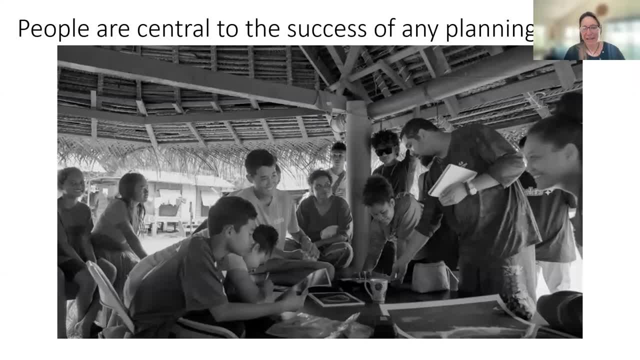 Okay next. So this lands us back to people, and what we're doing with all this work is to try to integrate it into a broader tool that puts connectivity in the context of other things that people are interested in. you know, coral cover and fish, biomass and all sorts of stuff. 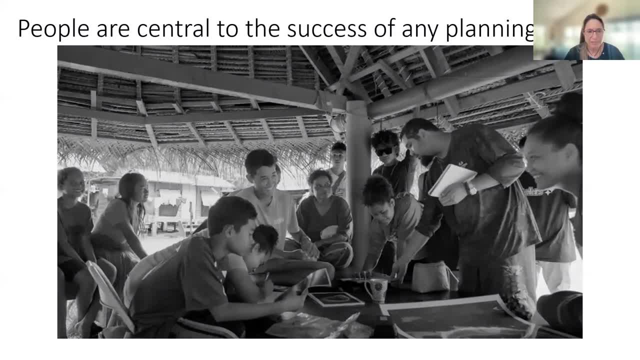 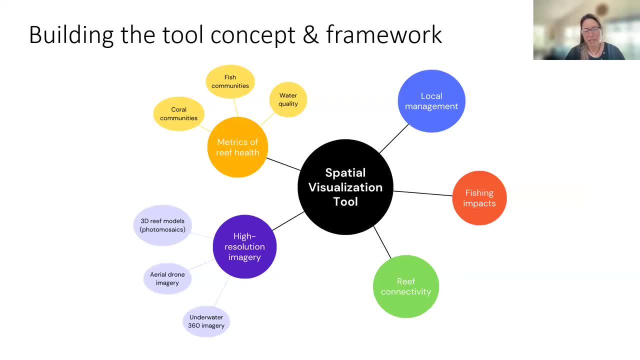 We're doing isotope work, So let me have the next slide here. So we're developing this spatial visualization tool and you can see that reef connectivity is a piece of that- as a way for people to visualize what's happening on their reefs over space and over time. 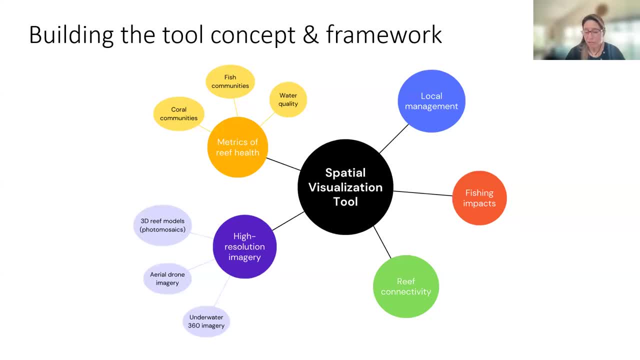 to be able to layer these different things on top of one another or look at them separately, depending on what people are most interested in seeing, so they can make decisions about their management And, again, if people understand the reefs from these kinds of perspectives. 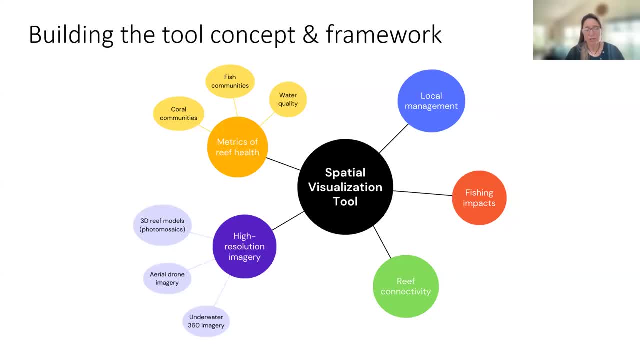 they can start working from where they really sit, which is from their own social and ecological and management perspectives, And we see a much greater longevity to those plans and in some cases we've seen results in less than a year when people just take action very quickly. 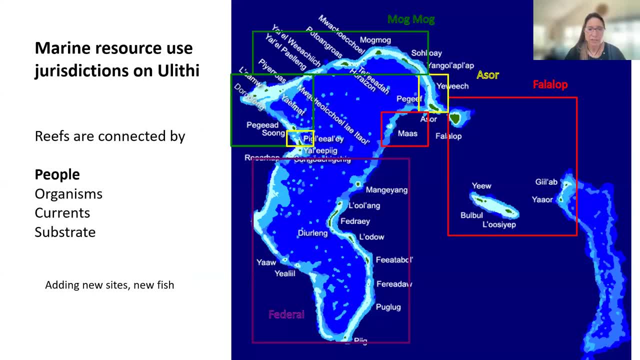 on some of their reefs Next. So back to this slide briefly again, showing that it's the jurisdictions and the people who manage them and the relationships between the clans that really drive all of this, and our science really supports it rather than leads it. 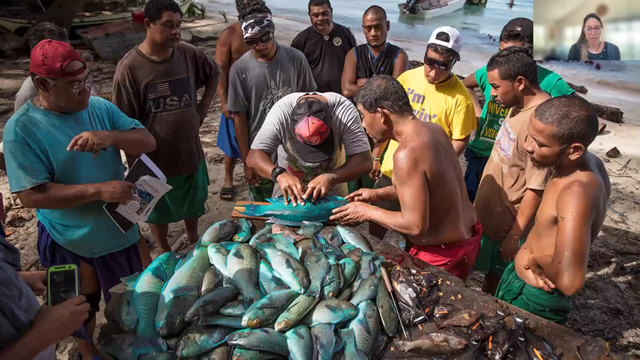 Next. So we are looking, as Jason mentioned, at some new fish. They're very interested in this type of parrotfish, so this is next on the docket for Jason's work- looking at connectivity in this fish, and so we've selected a few fish. 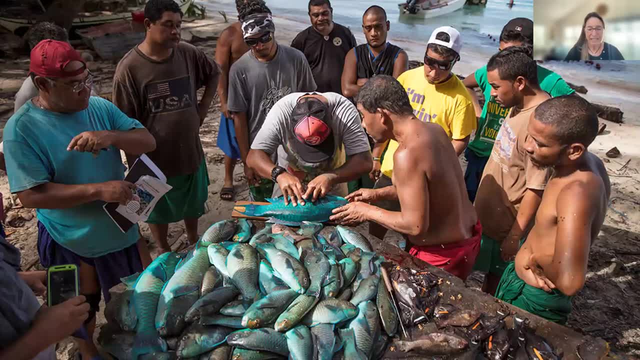 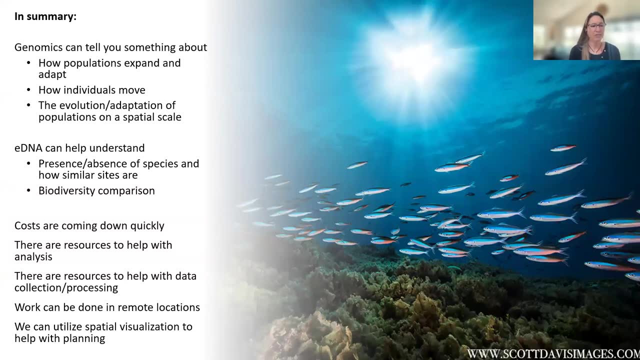 that they've really decided they want to learn more about. And next, and I think we're down to the end here. So, in summary, genomics can tell us something about how populations expand and adapt, how individuals move, The evolution and adaptation of populations on a spatial scale. 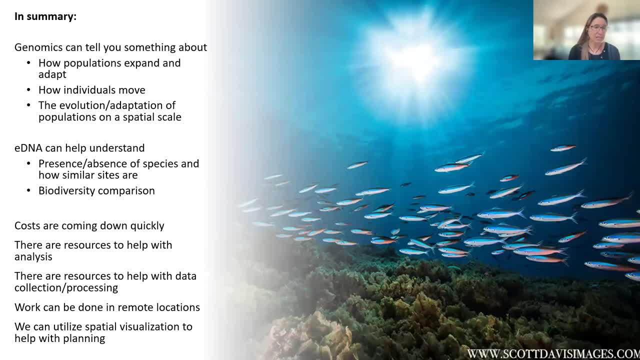 eDNA can help us understand presence and absence of species and how similar sites are or different, like a biodiversity comparison. Costs are coming down quickly. There's resources to help with analysis and with data collection and processing, and work can be done in remote locations, now more than ever. 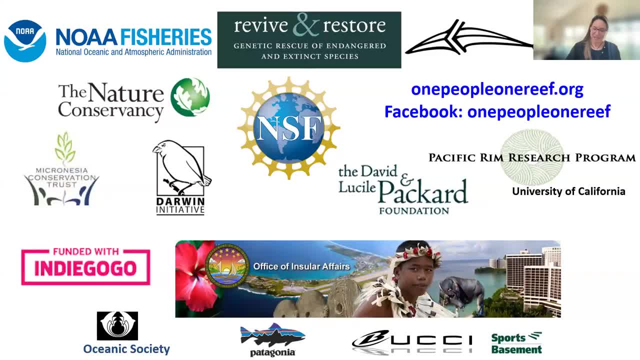 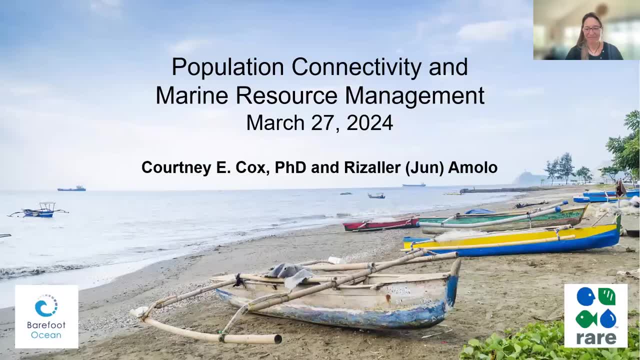 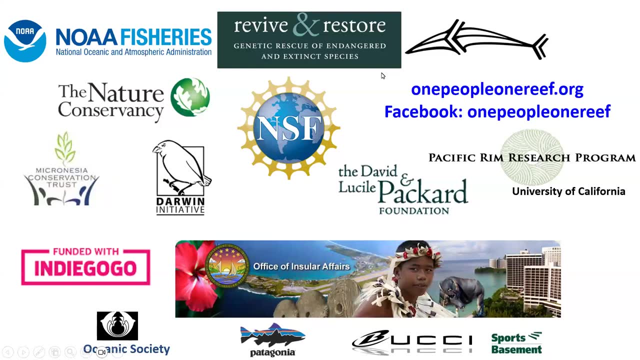 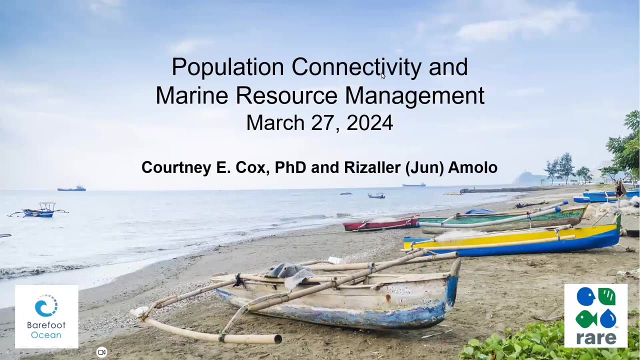 Next And last. So thanks so much, everybody, and looking forward to questions. Thanks, Nicole Courtney. We'll start yours and we'll do all the questions and answers session at the end. Great Thanks, Caitlin, And hello everyone. 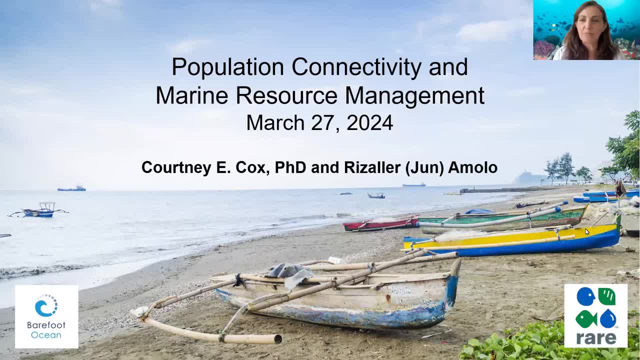 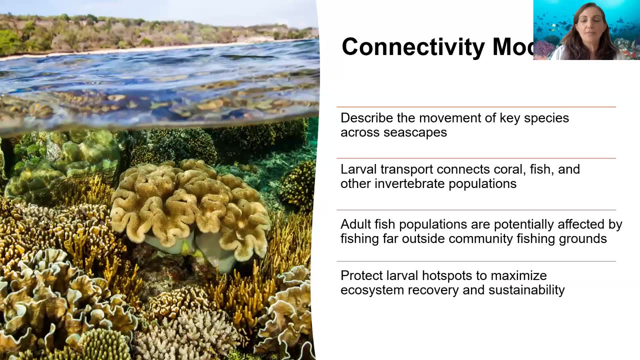 I'm thrilled to be here today to discuss our efforts over the past few years integrating connectivity into decision-making processes for our area-based management. Next, please. Okay, so we've been working on a modeling approach to understanding connectivity, So larvae can travel long distances. 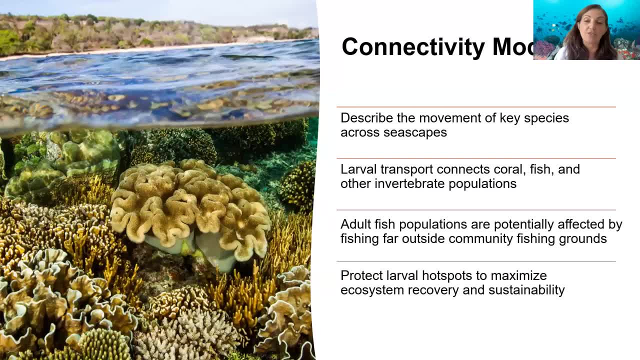 ending up in very far-off places or back to where they started. Our focus has been to simulate these dispersal patterns and understand how larval transport links coral fish and other invertebrate populations, the implications of those connections and how managers can use this information. 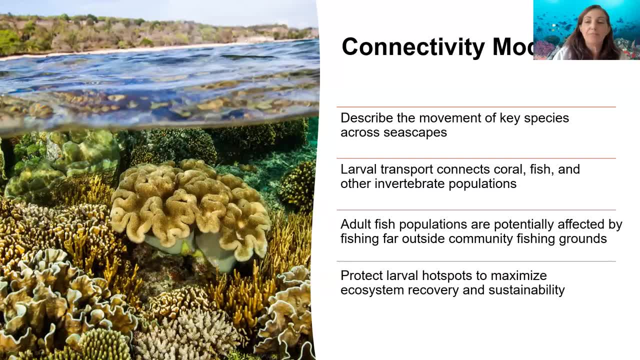 Adult populations, for instance, could potentially be influenced by fishing activities well beyond community fishing areas through the connectivity process. So we've been working with the National Center for Environmental Policy and Sustainability. Modeling We can provide data to aid in the protection of larval hotspots. 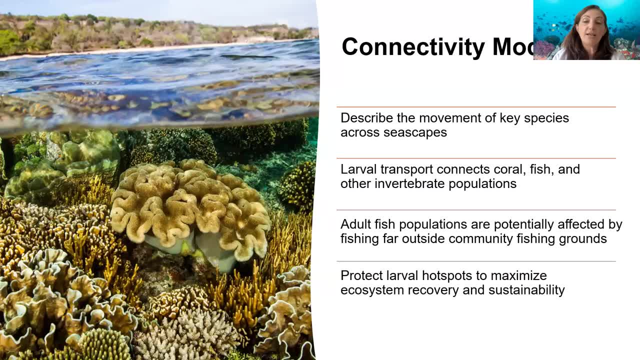 And protecting these hotspots can enhance ecosystem recovery and sustainability, as well as support the livelihoods of the communities that depend on them. So, as Nicole also mentioned, we are focused on providing data that can be used alongside other ecological, social and fisheries data to make decisions. 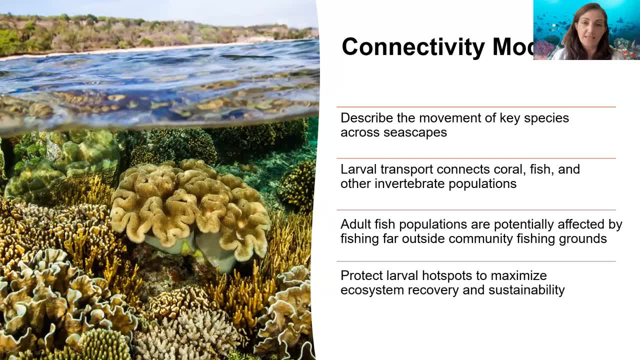 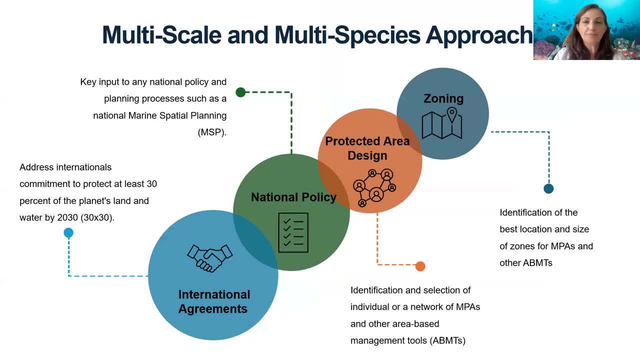 with the community, With the communities always at the center of the efforts and the data Next, please. So our objective has been to provide resource managers with a versatile decision support tool that can be used across geographical scales and species. We can use connectivity to support international commitments. 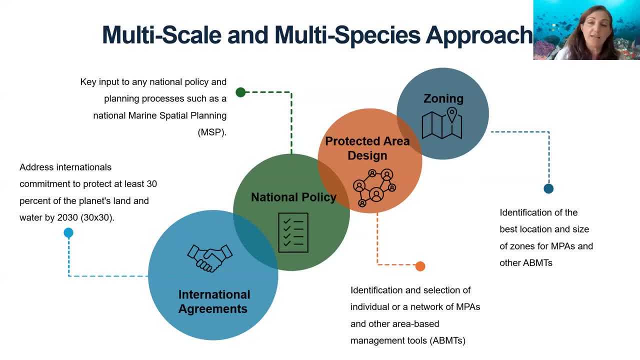 such as 30 by 30.. These can provide crucial data for national policies and planning processes, like marine spatial planning, And the data can be used to design networks of marine protected areas or other area-based management tools, as well as provide input into zoning strategies. 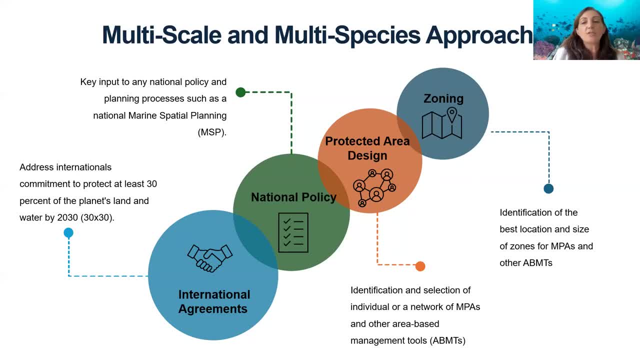 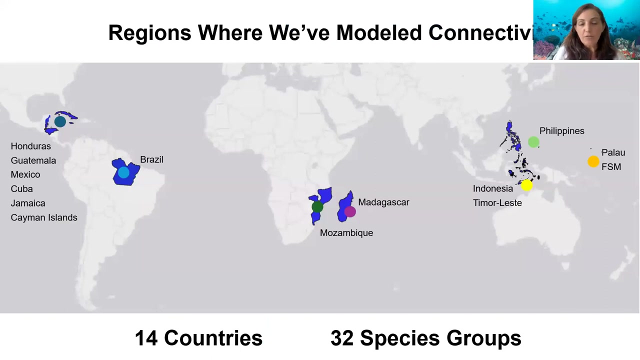 within those areas. This multi-scale and multi-species approach can empower resource managers to strengthen ecosystem resilience by pinpointing optimal locations for both conservation and fisheries management efforts at national, regional and local scales. Next: So, over the past couple of years, 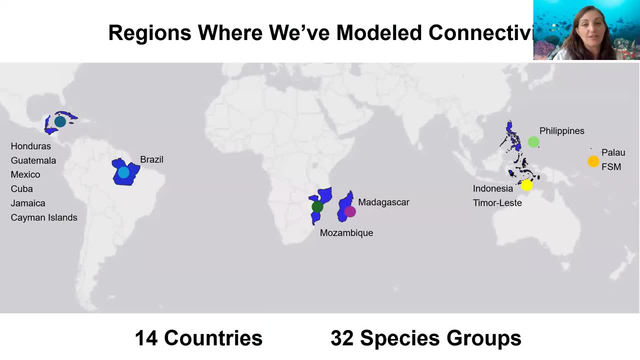 we've been working on using this approach in a wide variety of geographies. We've used this approach across 14 countries. We've modeled 32 species groups And I'll explain that in a minute. what I mean by species group. So from the Caribbean. 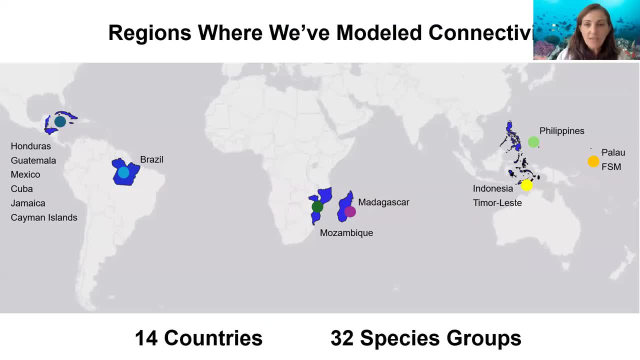 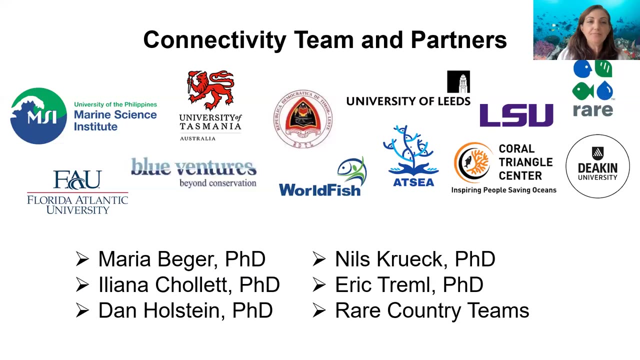 all the way over to Palau and FSM. we've developed larval dispersal models to help managers use these data in decision-making around area-based management. Next, And when I say we, this has been a big team of folks that has been involved in developing this approach. 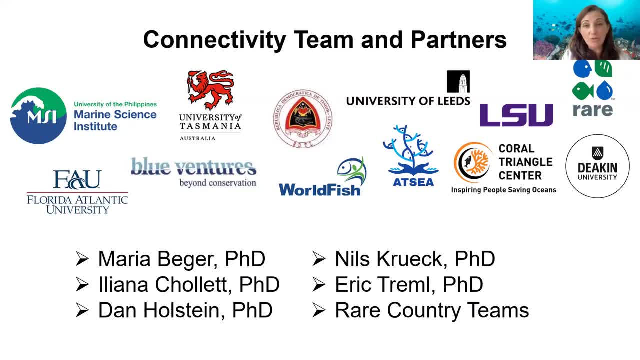 developing the connectivity metrics that we're using and how we're using them, both from the academic side and the practitioner side. So some of the key folks that have been involved in developing the approach are those listed at the bottom. We're in close collaboration. 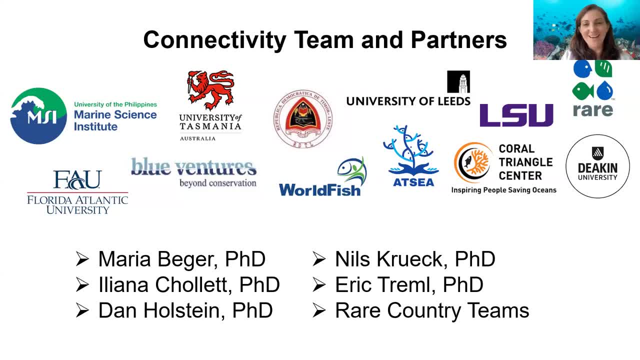 with these academic minds And then the rare country teams who were our folks on the ground, who were making sure it made sense and could work in practice And we'll be hearing from June in a bit on some examples of that. So we're excited to be partnering. 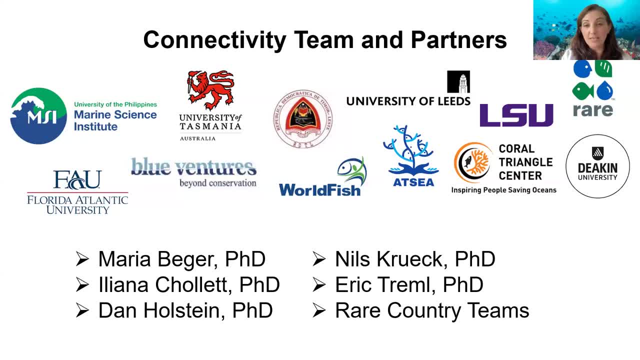 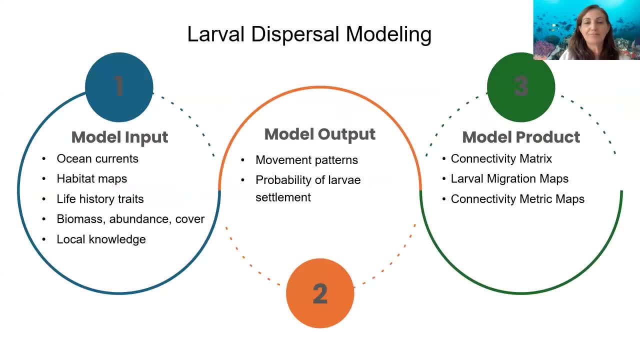 with many organizations to develop scientifically sound strategies that can work in the field. Next, Okay, so there are two primary ways that we can think about visualized larval dispersal: Where do larvae go and where do they come from? The ultimate products are maps. 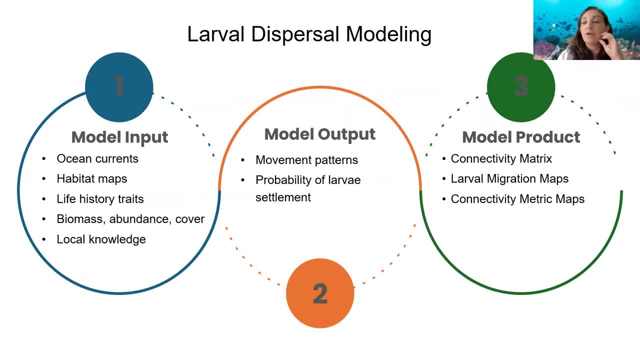 showing important export or source areas, Where do they go, And important import or sink areas where do they come from. So to get there, we first have model inputs, And there are five main model inputs: ocean currents, habitats, life history traits. 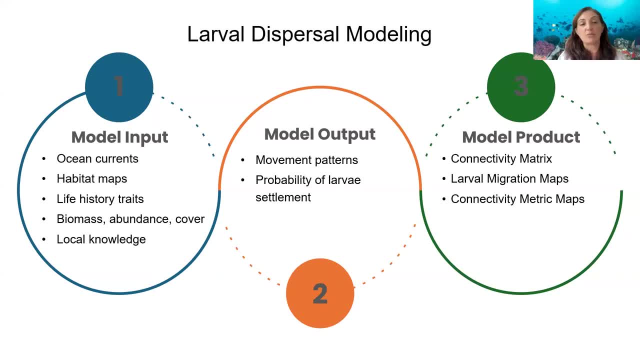 the biomass abundance or cover, depending on what species we're modeling, and then local knowledge, to ensure that any global data sets are accurate or as accurate as possible, And so the model outputs. we're looking at movement patterns, as I mentioned, and then the probability of larval settlement. 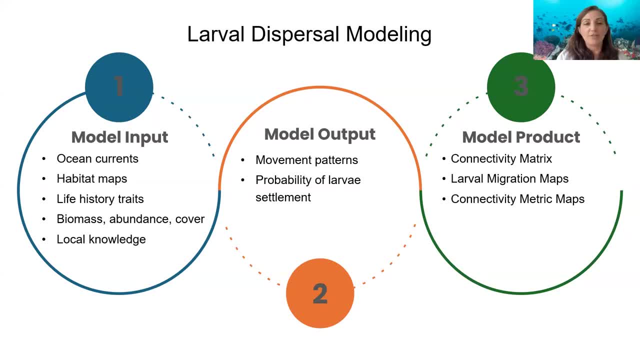 in habitat patches And products. we're looking at the connectivity matrix, which describes how larvae are moving from one habitat patch to another, And then visualizing that matrix in migration maps and the connectivity metric maps, which I will show you guys some examples of. 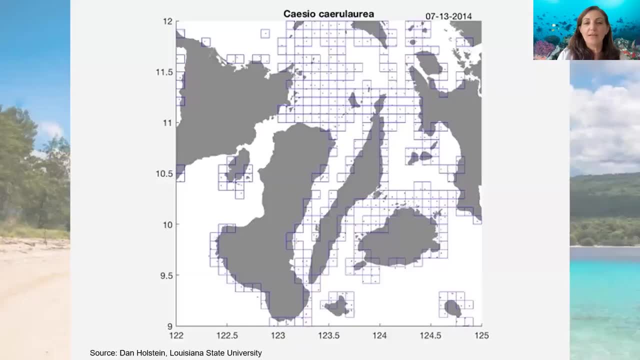 in a few minutes, All right, So, Caitlin, if you could press play on this one, Okay, so this is an example of what the model is doing. So each one of these polygons is a habitat patch, And so, like I said, 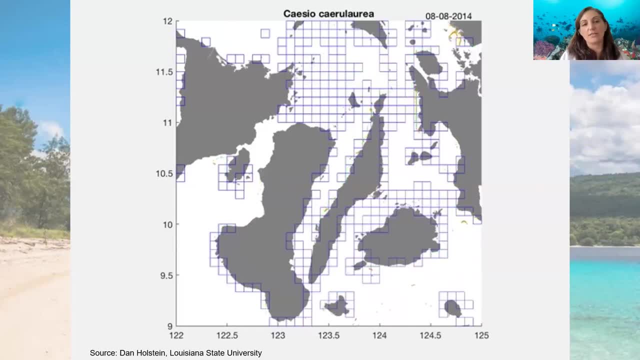 we're simulating how these larvae are moving across the seascape And with this information, we can then transform this information into metrics that can allow and enable resource managers to use this type of visualization or model to make decisions about where to protect or where to zone. 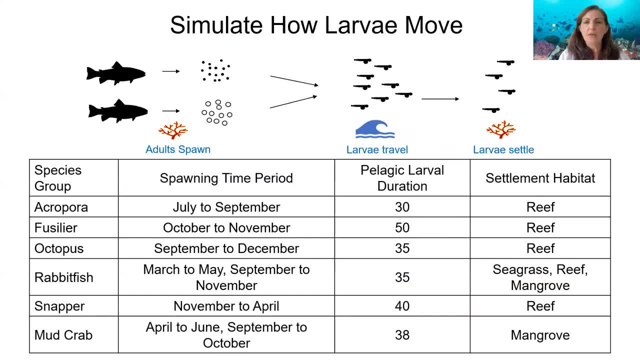 Next. So how does this work exactly? So the simulations is pretty straightforward. We are simulating adult spawning, whether it's a fish or coral or another invertebrate, how they travel across the ocean currents. So the hydrodynamic model or the ocean current model. 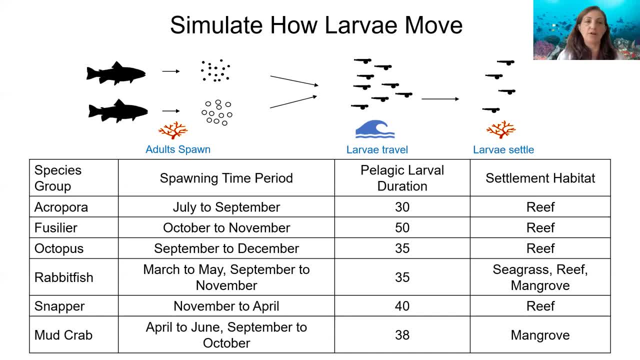 is critical in this process, as those larvae are being released in the larval dispersal model and then traveling across those currents, And then they're settling when they reach their habitat. So the habitat maps are being used to identify the areas where we can tell the model. 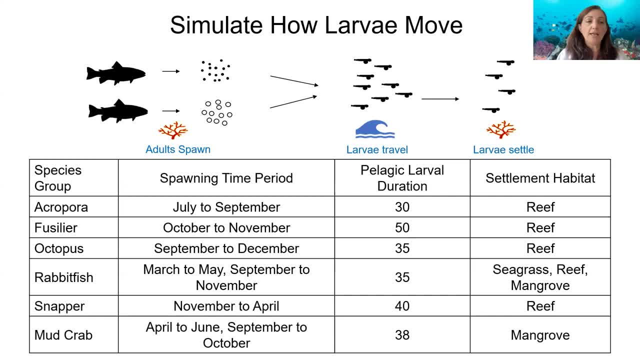 to settle the larvae And the multi-species approach. we've used the model to simulate movement across acropora species, octopus, various fish species and mud crab. And these are the different life history traits. some of the different life history traits. 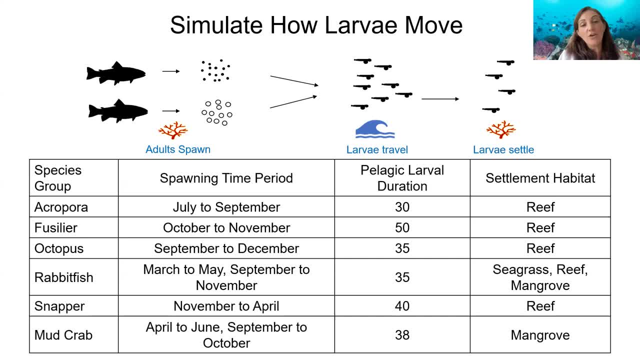 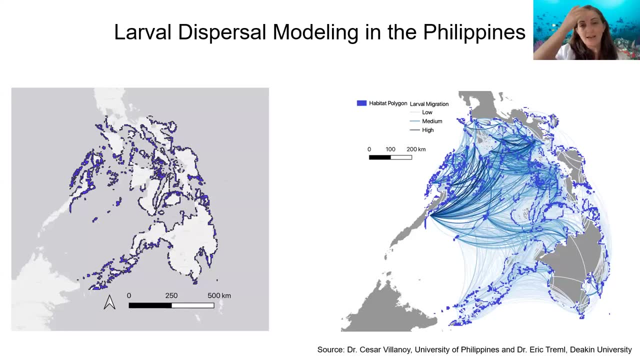 that go into the model, So that spawning period time, how long they spend in the water column and then where, what types of habitats they're settling in. So we're going to be focusing on the Philippines examples today, So this is an example. 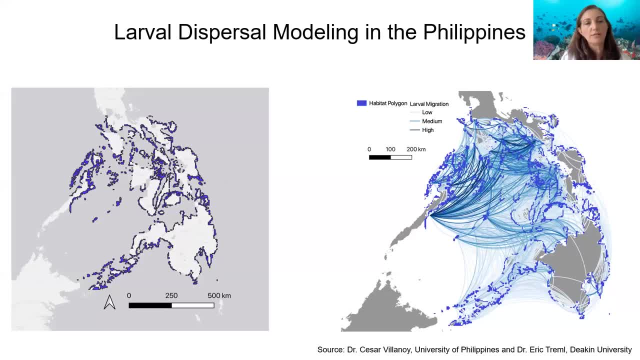 of. on the left you'll see the map of the model of the migration map across the Philippines And this is a map of the migration map across the Philippines. So the migration map is a map of the migration map across the Philippines and the habitat patch. 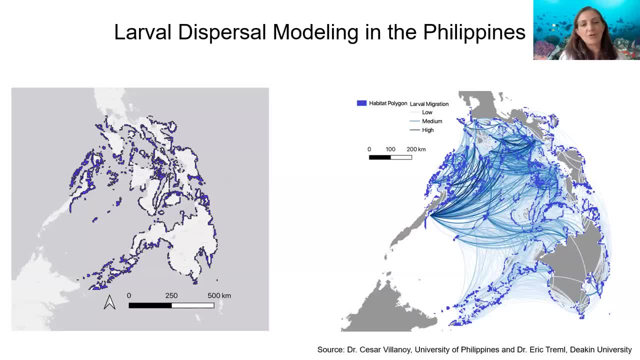 And so we modeled dispersal of 10 species across the Philippines. The map on the right will show you a product of the migration map, And so what this is showing you is the migration from low, medium, high, from one of those patches, and then the direction. 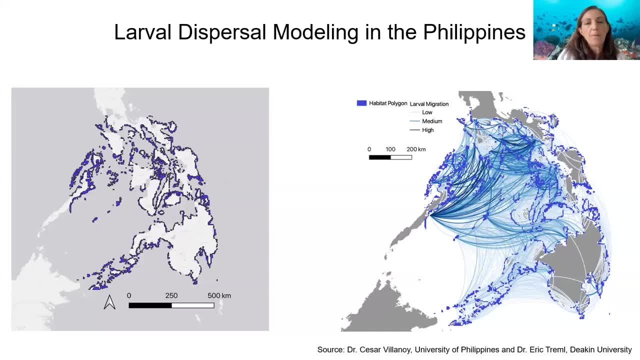 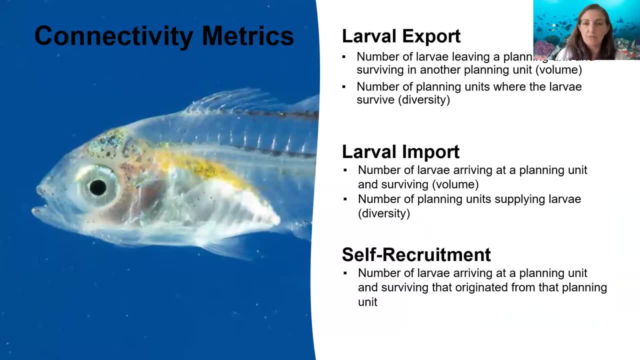 of that migration is in a clockwise direction. Next, And from those migration matrices, or that the quantification of the larvae that are moving from one patch to another. we developed three main connectivity metrics: Export, import and self-recruitment. So why are these important? 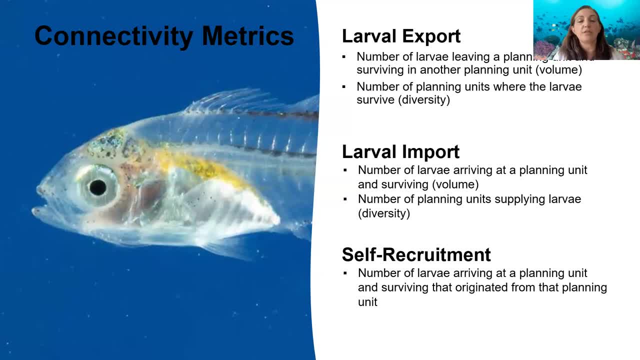 High export areas supply larvae to replenish depleted populations. High import areas receive diverse and abundant larvae, improving potential for recovering from overfishing or any other natural catastrophe or threat to those populations. The high import areas also increase the potential for genetic diversity as well. 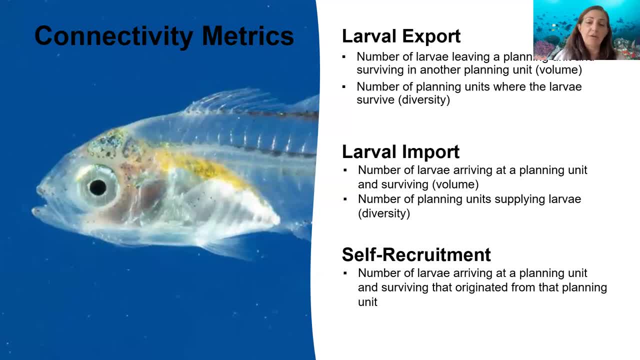 The high self-recruitment amplifies the benefits of local management, because larvae leaving a reef are likely to return back to that same reef. So the efforts to manage and conserve local habitats have a direct positive effect on replenishing and sustaining populations within those areas. 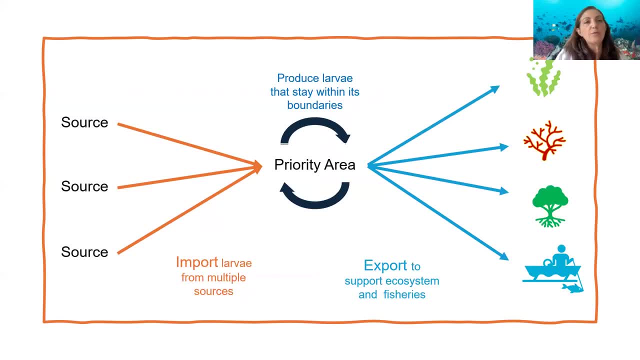 Next. So the way that we've been thinking about this is to select a priority area. We're looking for all of these things ideally. Often this is not possible, So we'll look at one metric over another, But ideally we're looking. 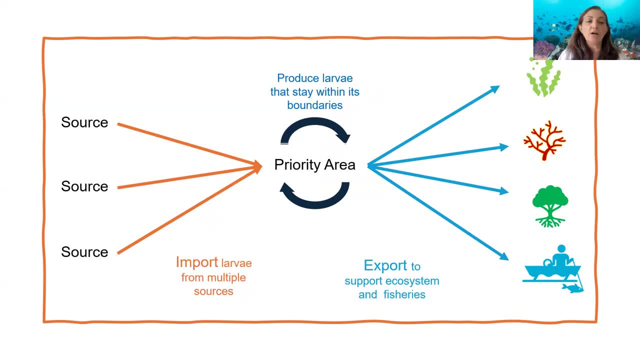 for priority areas that receive larvae from multiple sources receive lots of larvae from lots of places, which is looking at the volume of those larvae and the diversity of the larvae that are supplying the area, And then also the areas that produce larvae that stay within its boundaries. 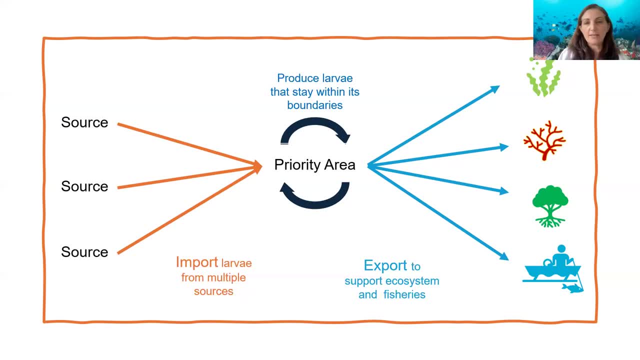 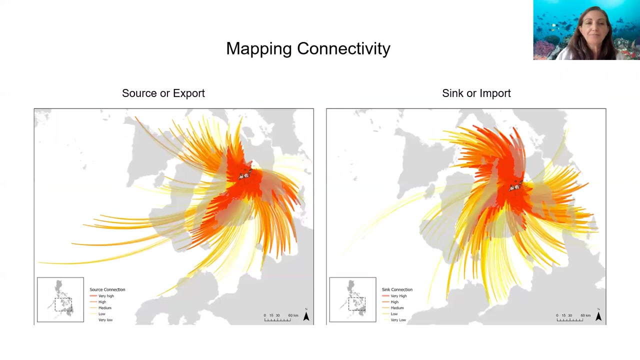 As I'd mentioned before, we're looking at amplifying the benefits of that local management back to itself. And then the export function, which is the supply function, And is this area supplying larvae to support ecosystems and fisheries across the region. Next, 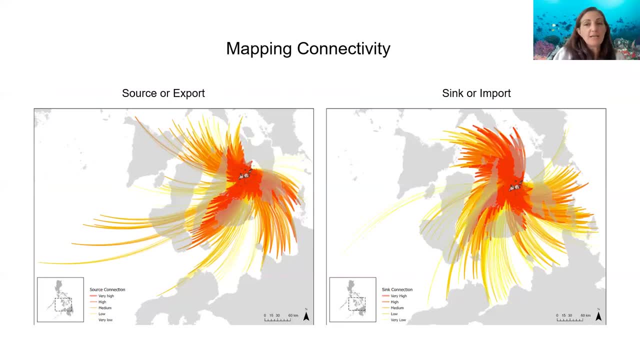 These figures show larval migration routes to and from comotes in the Philippines. So the migration routes, as I said, run in a clockwise direction And the strongest larvae transport are represented by the darkest red lines. So here you can see the extent. 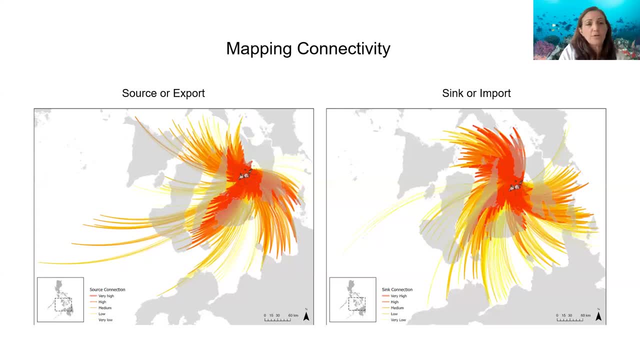 where larvae are going with that source or export area from comotes and where the larvae are coming from that settle in comotes. So with this information we can identify areas within comotes that are well connected to other reefs and prioritize those areas for protection. 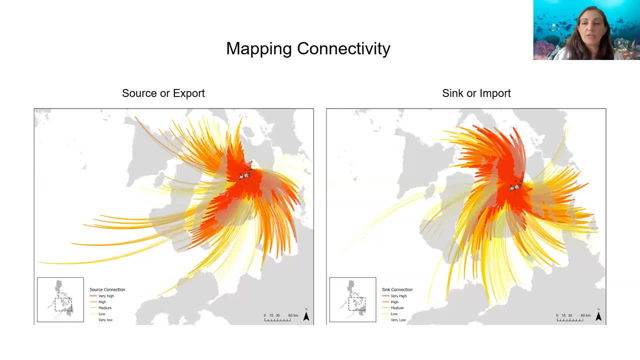 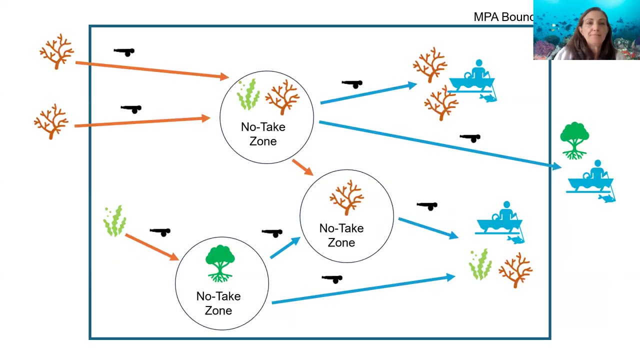 We can also identify municipalities or regions that are dependent on one another for larvae transport, And this can guide decisions around forming alliances or agreements across regions that can result in a greater collective benefit. Next, So then, when we're taking this approach to a network effect, 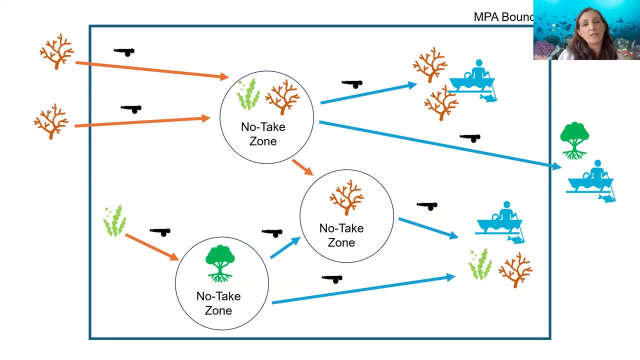 we're again looking- and this is an example of potential zoning- within an MPA, Zoning of no-take zones or any other area-based management approach, Selecting those areas that again have those high import, high export that are connected to one another. 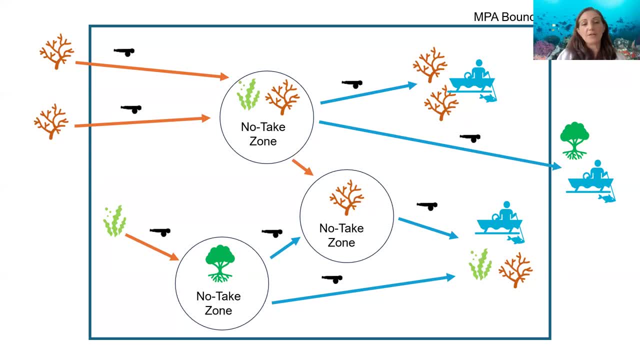 and also connected outside of the no-take zones, so that they are replenishing not only themselves within those no-take zones but are then providing a broader network of potential zoning and a broader benefit to the area, to the fisheries, to the ecosystem as a. 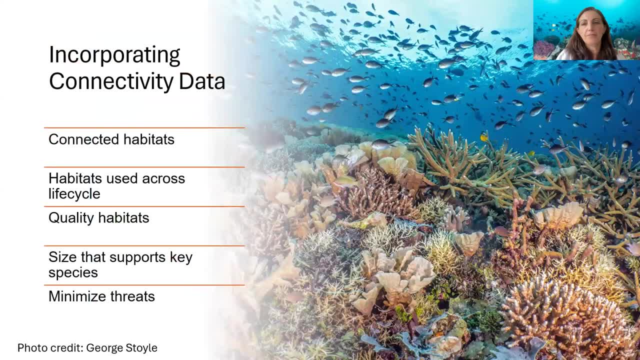 collectively, Next, And so incorporating connectivity data. this data is not meant to be used in a vacuum, as has been mentioned by Nicole as well. So, thinking about where habitats, where are the habitats that are well connected, also incorporating into the design of protected areas. 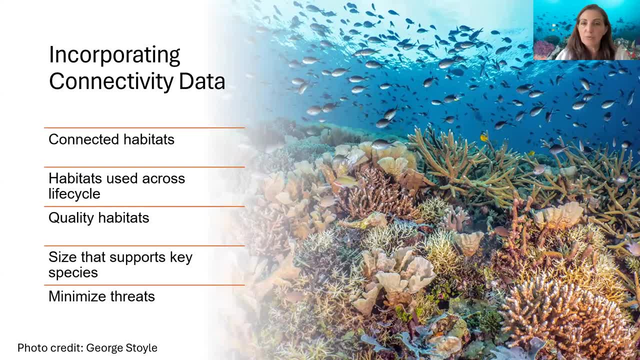 the habitats that are used across life cycles. So do species move as adults. And can we incorporate all of those habitats into protected areas, Looking at the quality of those habitats? so the larval dispersal model does assume quality because of its scale. 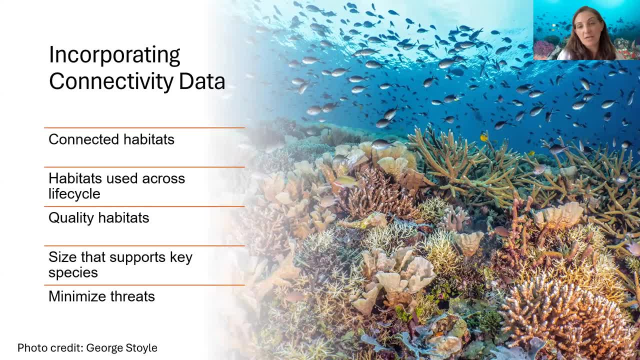 We don't have in-water surveys or habitat quality data in all of across the entire domain, So we do have to assume, so we are very reliant on local knowledge and folks just jumping in the water to make sure that these areas are quality. 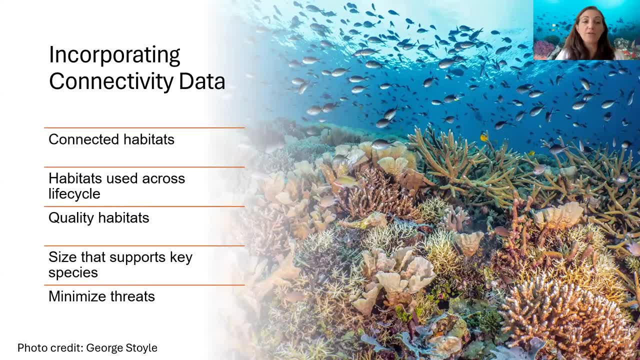 and that we protect the quality habitats. Also the size that supports key species. So size is a very important component as well to the design of protected areas And then minimizing threats And, on top of that, incorporating all of the social aspects, political aspects. 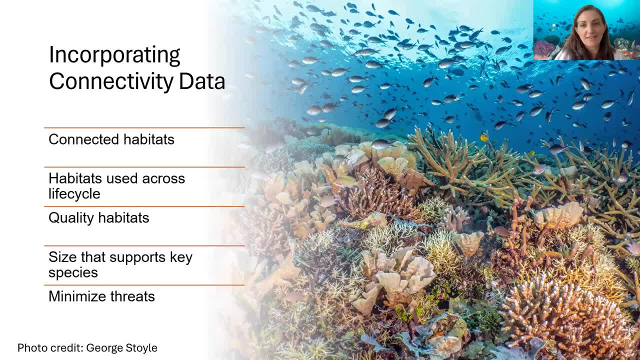 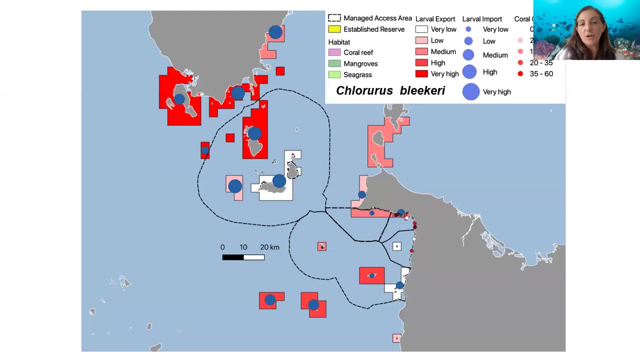 into this complex decision-making landscape, And so, when you bring all of this together, this is what this can look like. So in this map you'll see there's a larval export that are represented by the polygons, the regions of red polygons. 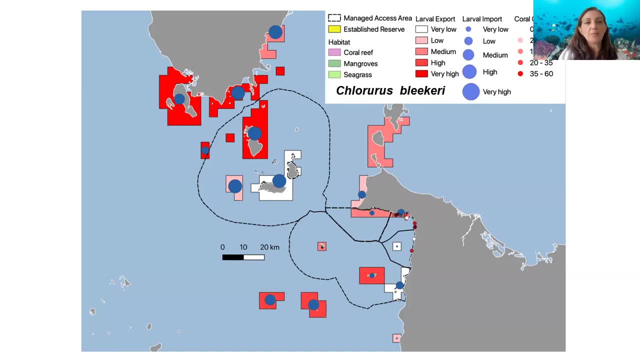 And we've categorized them from low to high. Larval import are the points, again categorized from low to high. by size. We've brought in some coral cover data as well, And then the overall habitat maps, And then bringing in some of the other boundaries. 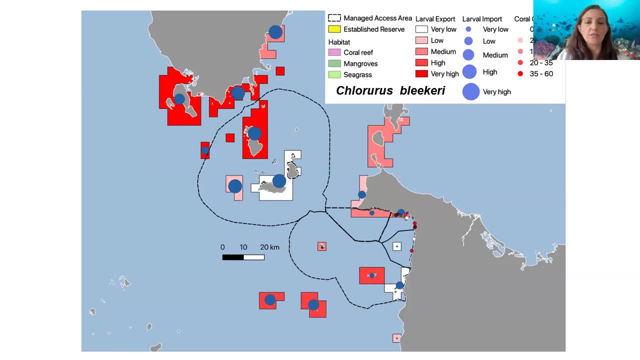 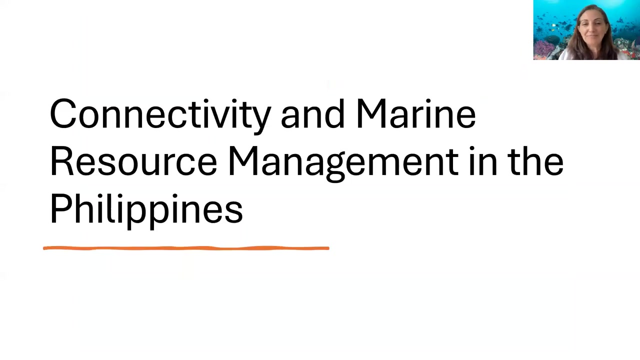 of existing protected areas to make those decisions around where to either focus for new zoning, expanded zoning, enforcement efforts. The data can be can be used in a variety of ways, And with that I'm going to pass it over to Jun. Yeah. 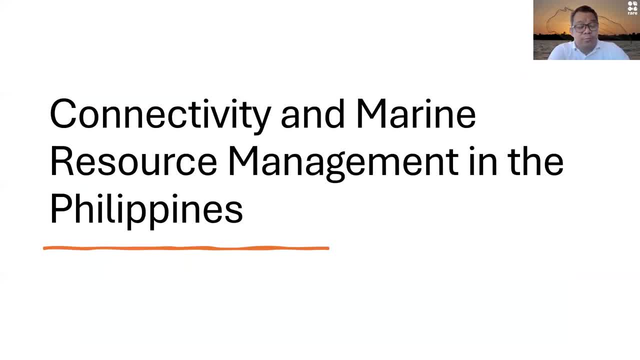 Good morning, good evening, wherever you are. So this is Jun Amohola from RARE Philippines. I'll be sharing the data of larval dispersal, along with other maps, other information generated from the models that Courtney was presenting in the Philippines. 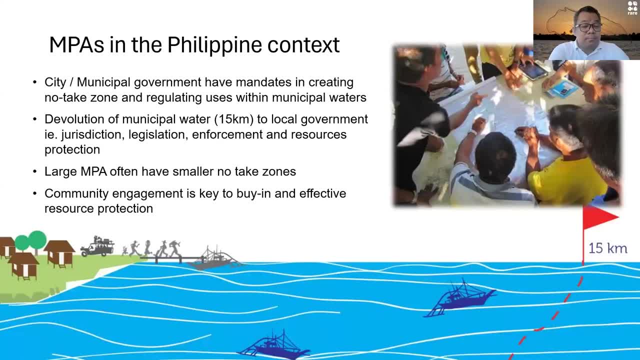 Next slide, please. So yeah, before that I'd like to provide some context In the Philippines, one of our uniqueness, of our marine protected area or marine local laws is really the management of coastal and fishery resources We devolved into the city. 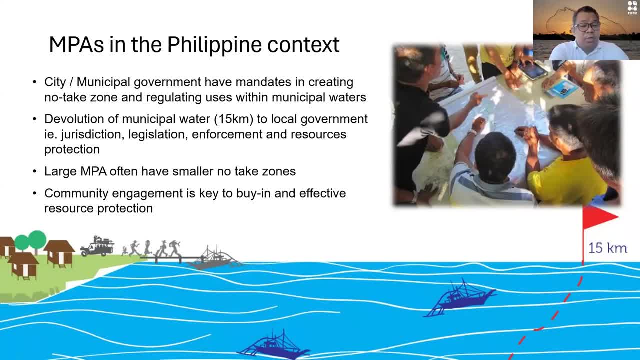 or municipal government. So the first 15 kilometer of this water is really managed by local governments, municipalities or cities. They have the jurisdiction, They can pass laws, They can enforce laws and declare areas for resource protections, And so there are. 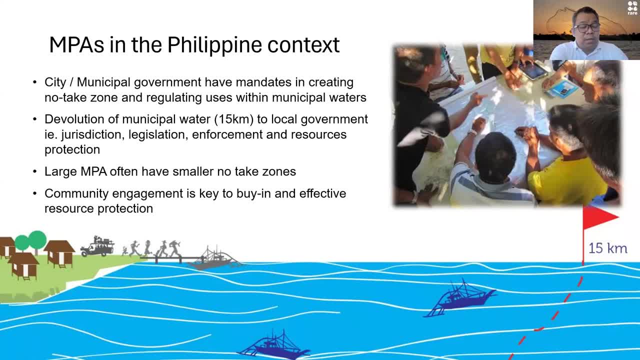 and national government also can declare areas with greater conservation values and declare it also as protected area. So in some areas or in many parts of the country there are big marine protected areas and within it are small no-take zones which are primarily used. 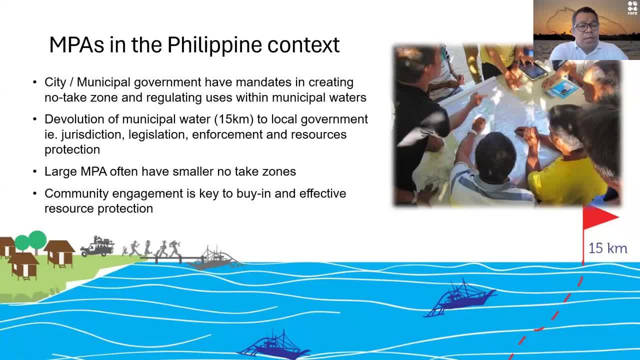 for fishery enhancement And then, because this is the laws, is devolved at the local government unit or the municipalities. community engagement is very crucial. It's key for the buy-in of these policies, of this effective for resource protection to be effective. 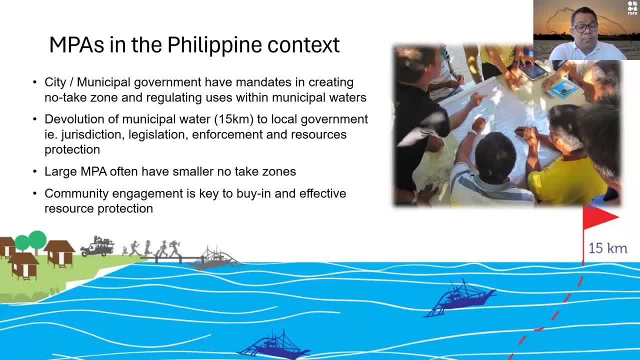 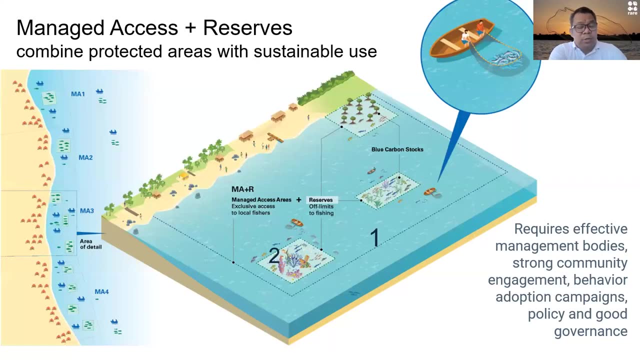 So yeah, municipalities, peoples, are very much engaged in designing, in creating these areas, no-take zones and marine protected areas in their waters in the first 15 kilometer. Next slide, please. So if you look at it, if you look at the municipal water, 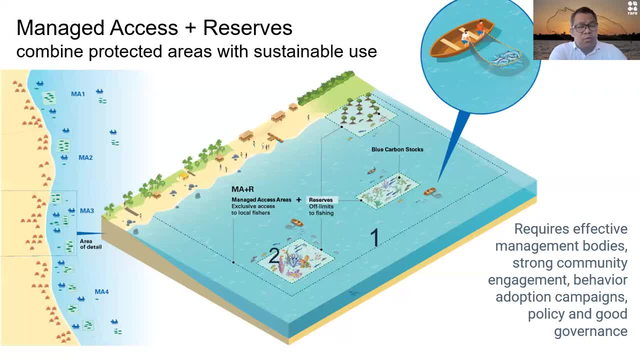 you need to manage who's fishing, who's using within this municipal water. Plus, you need to also establish important, well-connected, adequate size of reserve where no-take zones, no fishing, no human activity is allowed. So if you look at a municipal water, 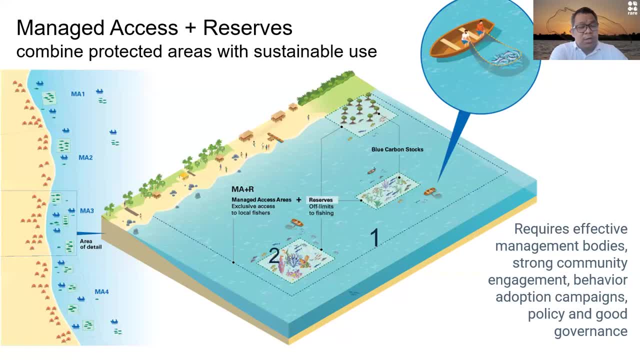 areas under the cities. you can manage this. There are areas that are. you know, management is access: who's managing who's accessing, who's using. that is, you need to talk to the community as well as you need to talk to the community. 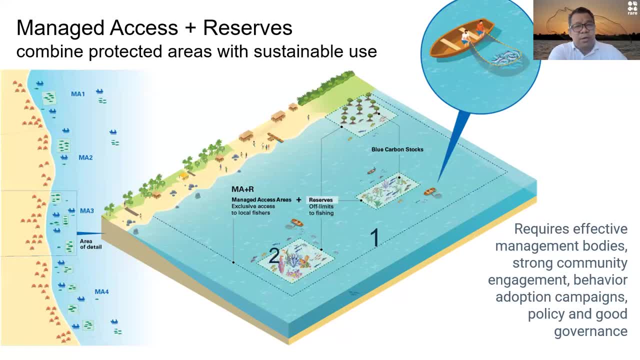 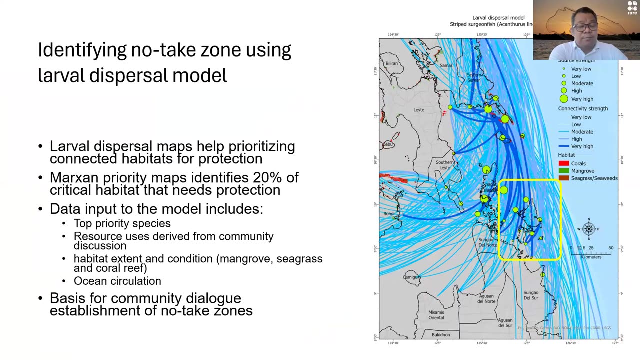 on where areas not to fish as a replenishing area or no-take zone areas. So that is always a the scenario in the local government, in the municipal government. Next slide, please. Next slide please. So that's a challenge. 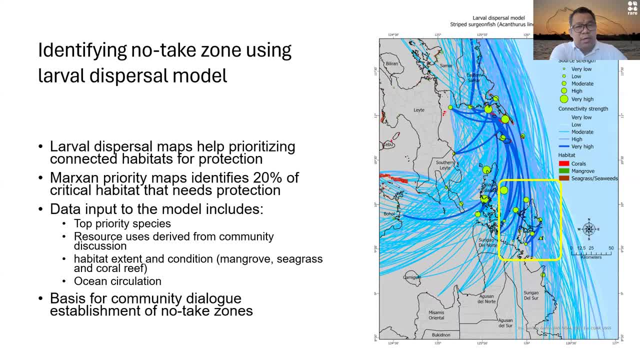 in the Philippines We have more than 800 coastal municipalities, So each municipality has to identify no-take zones as well as manage areas around around it within that municipal water, And then we're using the larval dispersal maps that Courtney and his group 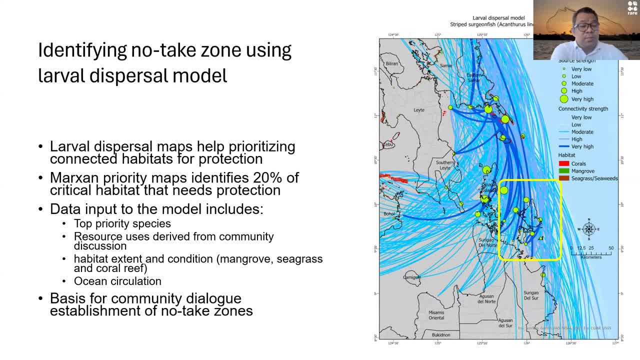 along with many of the scientists that have been involved to present, to identify priority areas connected habitats And we also use a MarkSan model to really prioritize 20 priority areas in the local community. So we have to identify the priority areas in the local community. 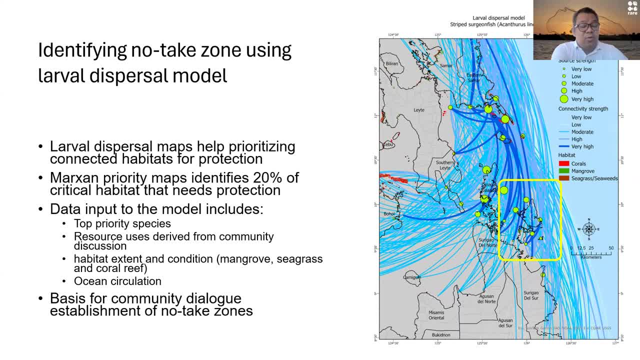 to be under no-take zone or under strict protection. So, in identifying that, you need to have those information, those models, as your way to convince local community or as a tool for community to decide as to where this no-take zone should be established. 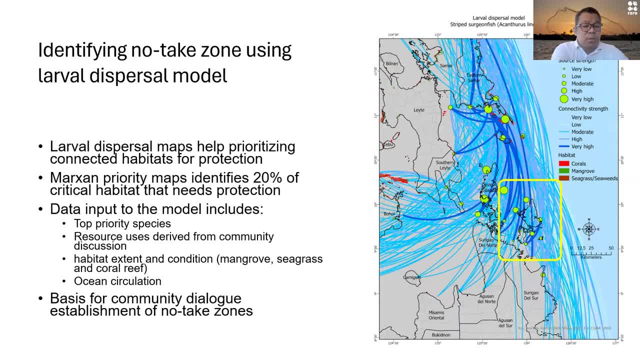 So we do have, we ask them, the priority species, who's using where? the extent of the habitat, the mangrove, the seagrass, as well as we ask you know, we do have ocean circulation data in the country. 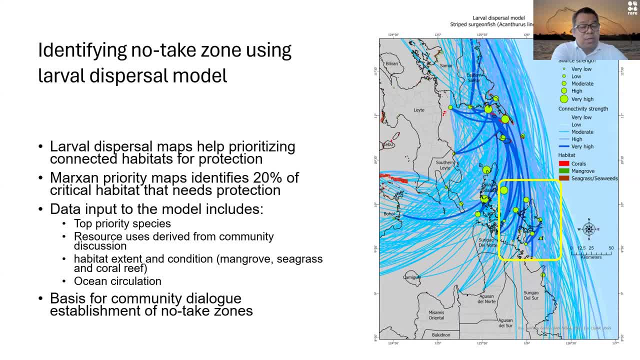 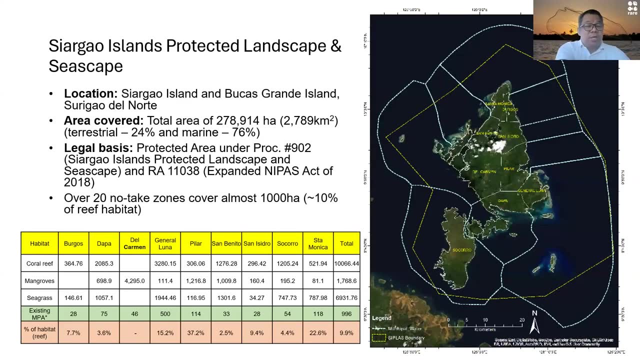 So this becomes now a basis for community dialogue in establishing no-take zone. So I'd like to zoom into one of the sites in southeastern Philippines, in Siagao. Next slide, please. So Siagao is both a national protected seascape. 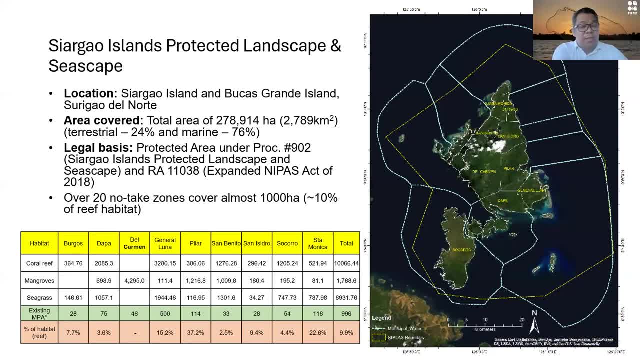 and there's also municipal. six, eight or nine municipalities also have jurisdiction within these waters, So it's a known surfing capital in the Philippines. So, and currently it has around 20 no-take zone over 20 no-take zone. 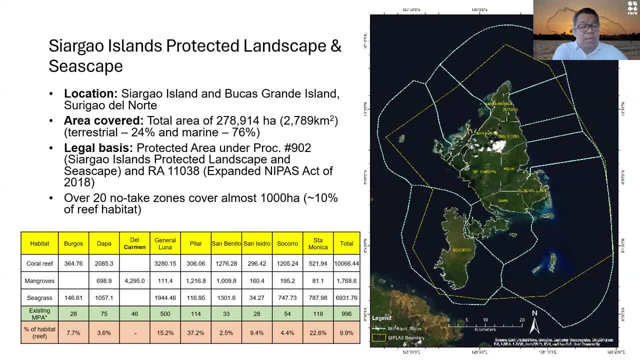 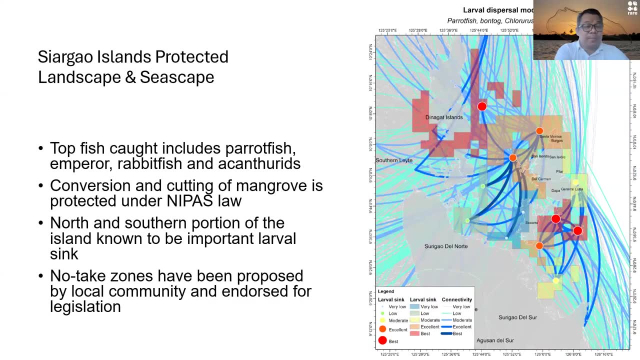 only covering 10% of the critical reef habitats. So the idea is to expand these areas, use larval dispersal maps to identify priority areas and bring this information to the community level. Next slide, please. Yeah, so so in Siagao. 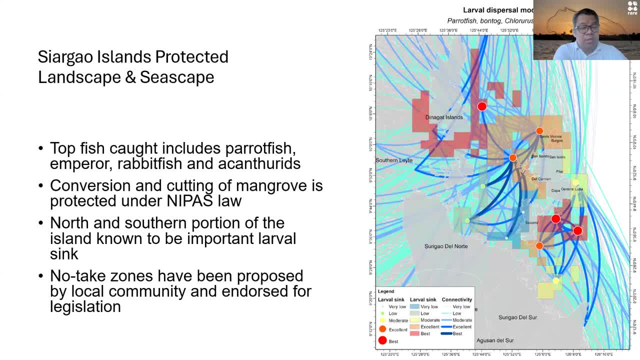 the top fish are parrotfish, emperor. the shrubbed fish are cantoids And we use this, you know, as mentioned by Courtney information, to model the larval source as well as the sink of this important species as a top species. 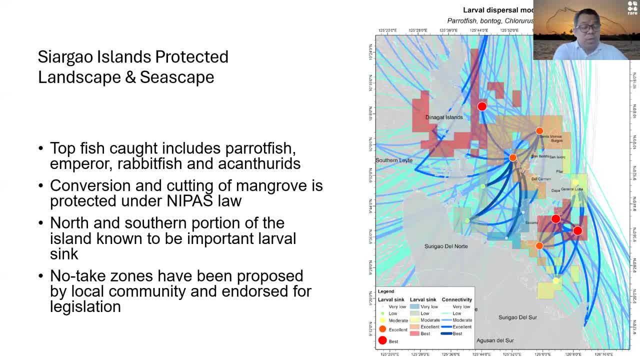 harvested by the fishers. no, And although our mangrove is protected by law, already no more cutting of mangroves in the Philippines, And we've also noticed that in Siagao Island, the northern portion and the southern portion of the islands. 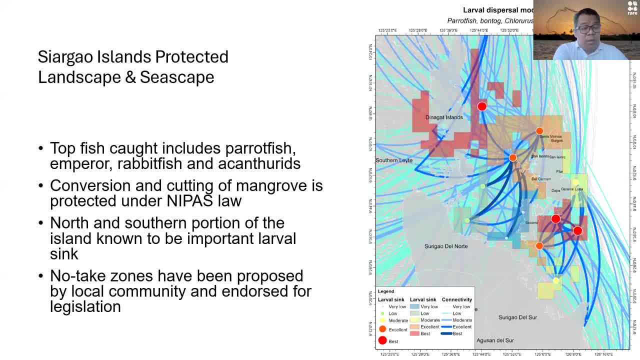 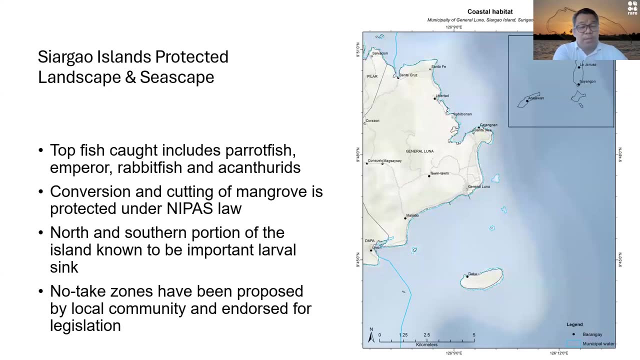 are key, important larval sink. So we give this, bring this to the community and let the community decide as to where to establish this no-take zone. So next slide, please, Next please. So we have this, for example: 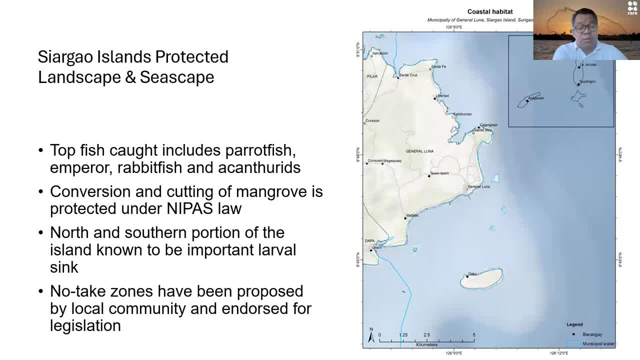 one of the municipality in Siagao, General Luna. This is one of the surfing capital. Next slide, please. We also have map of mangroves- Next slide- And seagrass, as well as the coral reef- Next slide, please. 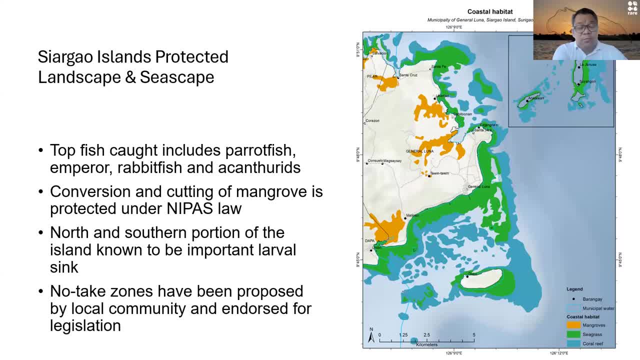 So we do have maps of those habitats, And then these are community drone maps, no? And then we also presented. next slide please. We also presented. we did also survey to establish coral condition in this reef. Next slide, please. 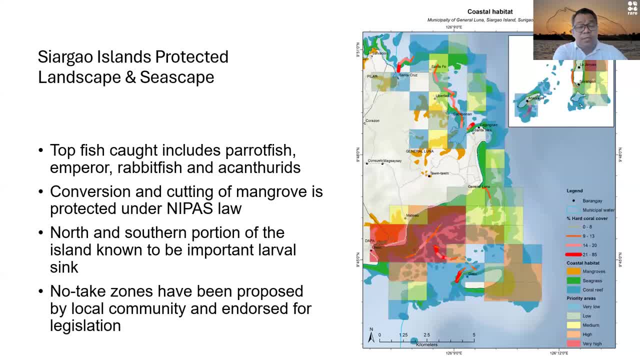 And then, based on the model we've identified, that this area, the red areas, are important, larval sink, and we ask the community to decide if we can put in no-take zone here And then next slide please. And then they've identified: 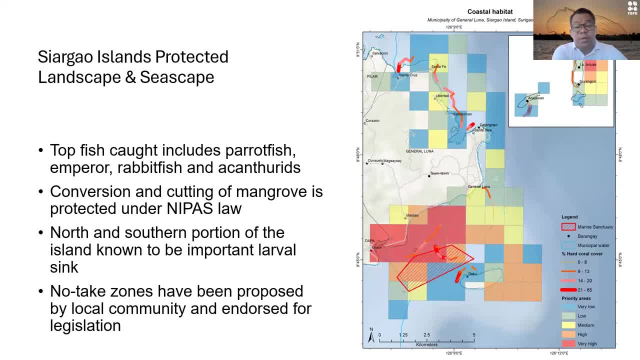 this, you know, red proposed marine sanctuary. I say almost 500 hectare marine sanctuary and they were able to decide- And this becomes a community- agrees on it. There's a regulation already that has been enacted to declare the area as no-take zones. 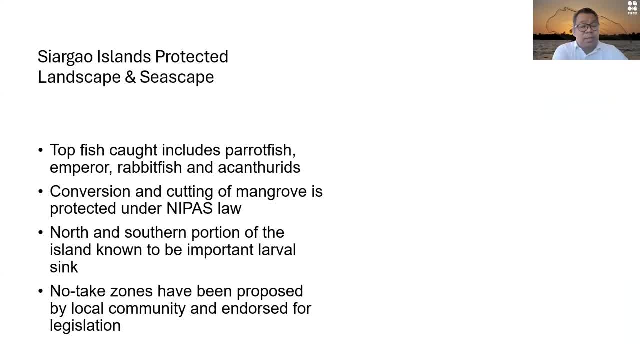 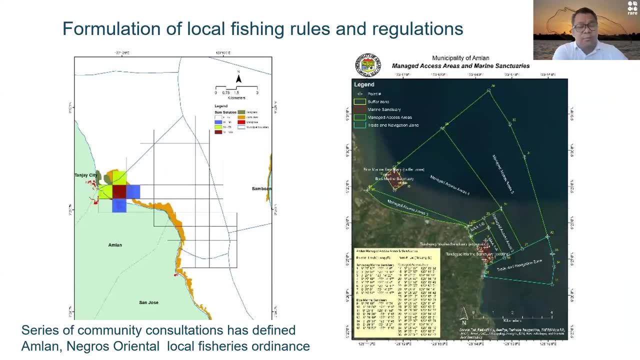 Next slide, please. And this is next slide. And this is happening in many of the rare Philippine sites in the country. This is, for example, in Negros Oriental, in one of the sites. This is the municipal water, The red areas. 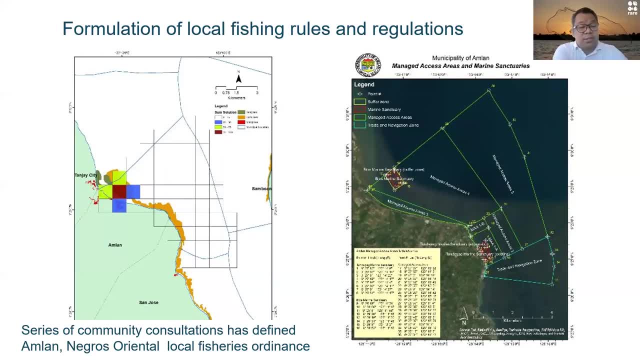 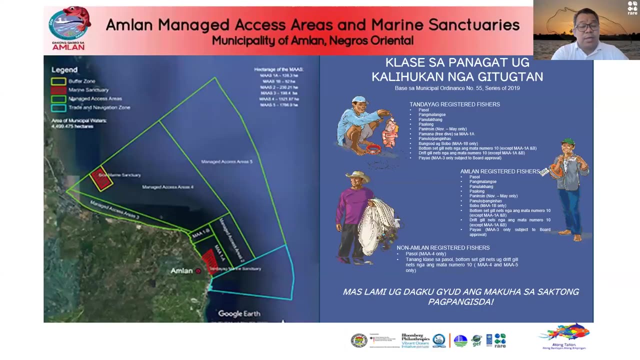 are the no-take zones, based on those models also that suggest that these are key areas, larval sinks or sources areas, And then around it are zones, different zones of different users in those municipal water. Next slide, please. But this is an example. 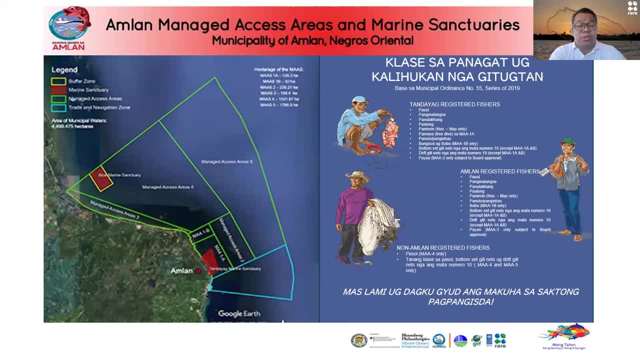 of those rules. In some areas only registered fisher can fish using certain types of gears. The other one allowed from other municipalities can fish, And here in this area there's like certain gears are only allowed at certain seasons. So these are regulations that have been agreed. 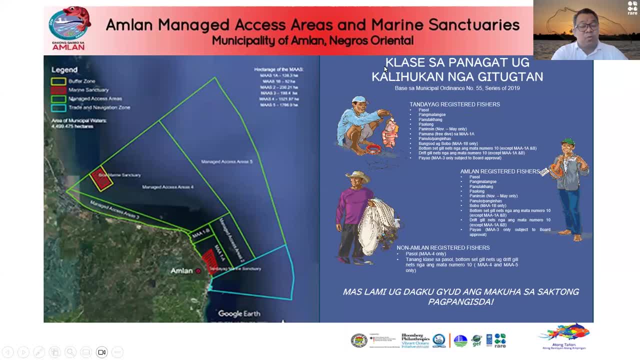 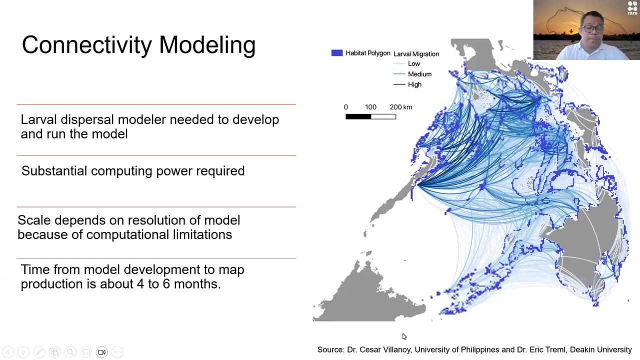 by the fishers, by the community, based on those larval dispersal map, along with other community discussions in the local government. I'd like to go back to Courtney for the conclusions. Thanks, June. So I wanted to touch on quickly about what is needed. 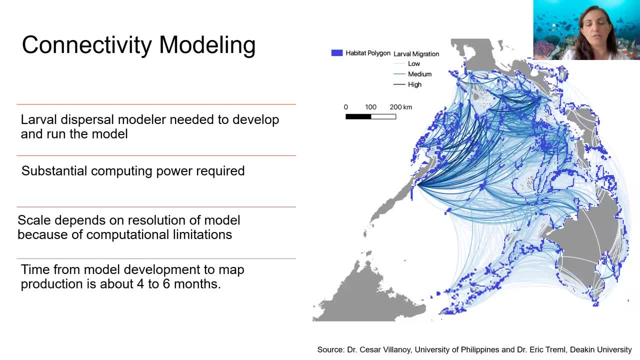 to do this type of work. So we've used models that were developed by Eric Tremel and Dan Holstein, And they have been the ones that are running these models. So substantial computing power is required. Experts are required. The scale depends on the resolution. 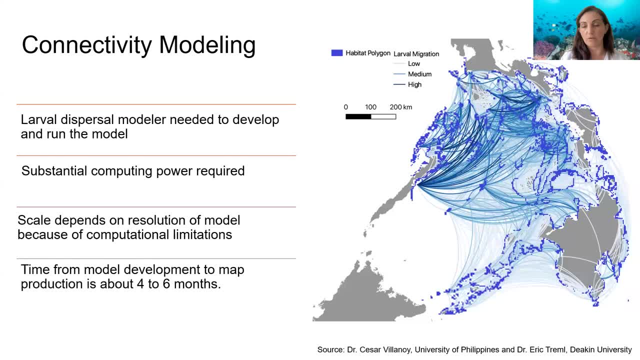 of the model. We're also working with hydrodynamic modelers to develop high resolution hydrodynamic models And so that we can answer questions at a higher resolution, And so the cost really depends on how big of an area you're talking about And if you need. 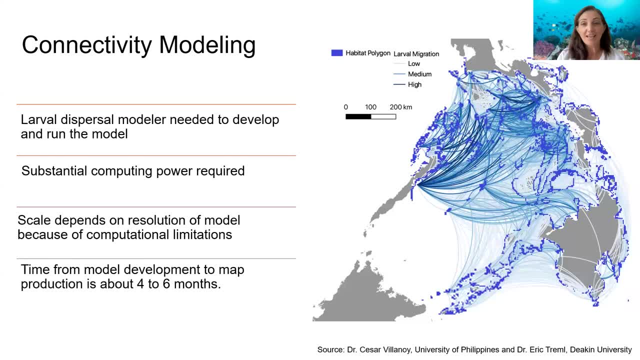 the hydrodynamic model and the larval dispersal model. If you're in an area where we've already run these models, it will be a much lower cost because you can just use that data. So that data is available for use And the time 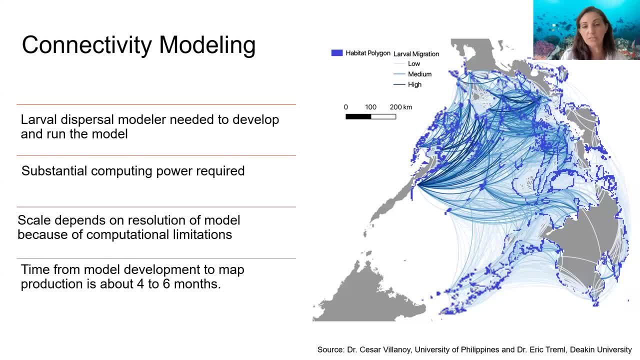 to develop the model, to map production is about four to six months. If you start from scratch, if you use existing data, then it's much faster, as you'll just need to analyze the data, And I'm happy to talk more in detail about any of that. 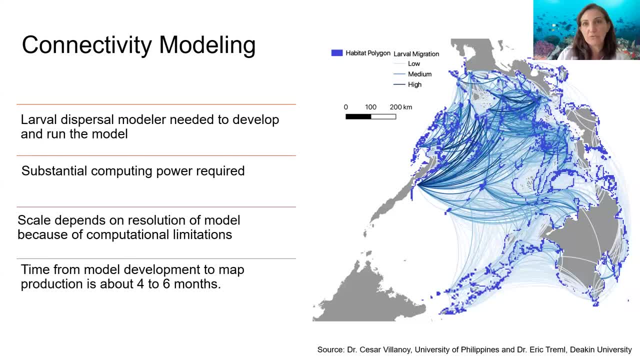 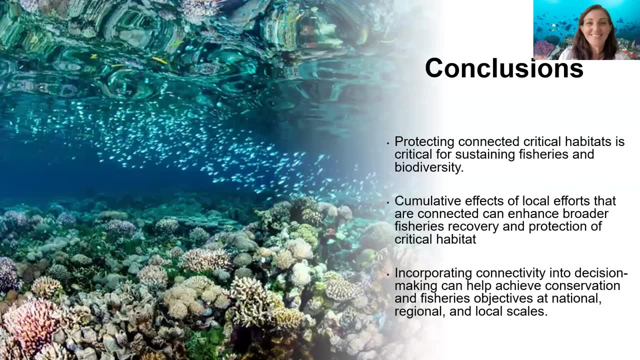 and also about any of the models that we've used to simulate the larval dispersal Next. So, in conclusion, protecting critical, protecting connected habitats is critical, as we all know, So the cumulative effect of those local efforts that are connected can enhance. 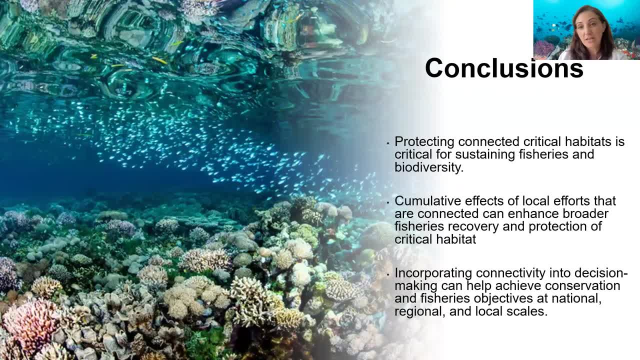 broader fisheries, recover and protection of the critical habitats. So using connectivity data at various scales can help amplify the effects of local efforts And, on that note, incorporating connectivity and decision making can help achieve objectives at national, regional and local scales. And that's it for us. 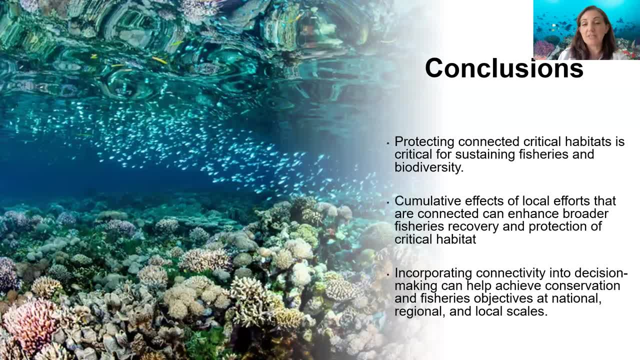 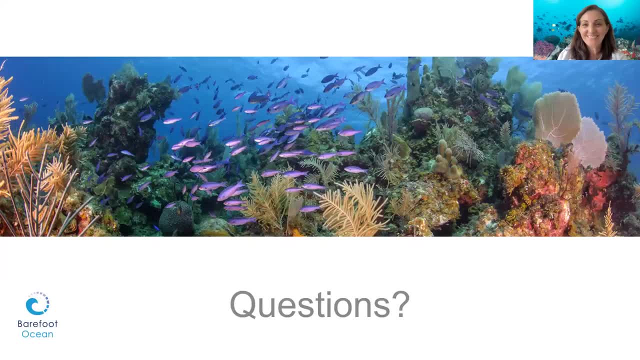 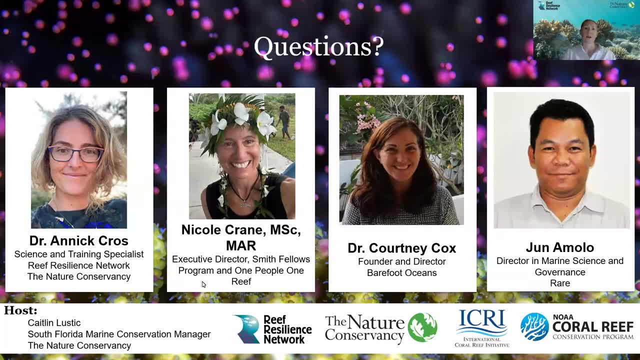 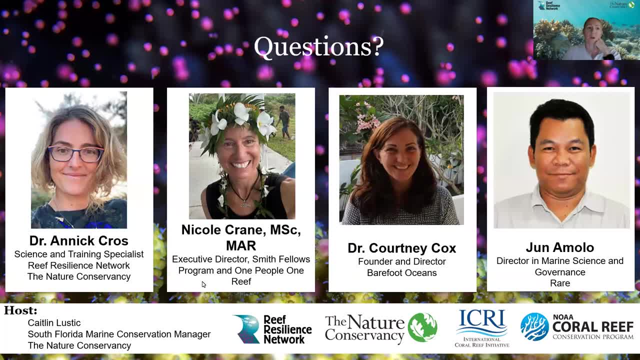 type your question into the Q&A box and I'll read it, or you can raise your hand and I'll call on you to unmute yourself, And we had a couple of questions that were coming in throughout, so I'm going to start with those. 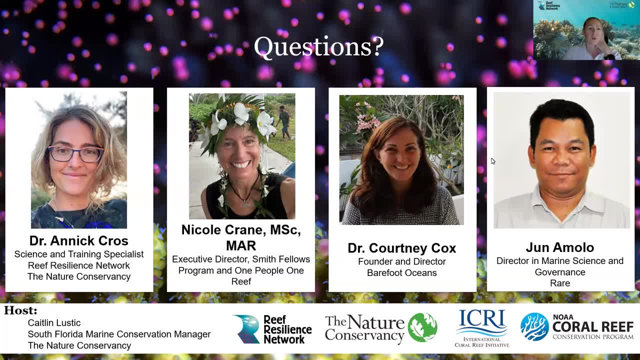 So this one was for Nicol. What is the eDNA entry point equipment cost? What is the cost of supplies to run a purchase to deal with an eDNA sample? I'm going to turn that straight over to Jason Perfect. You just did it all. 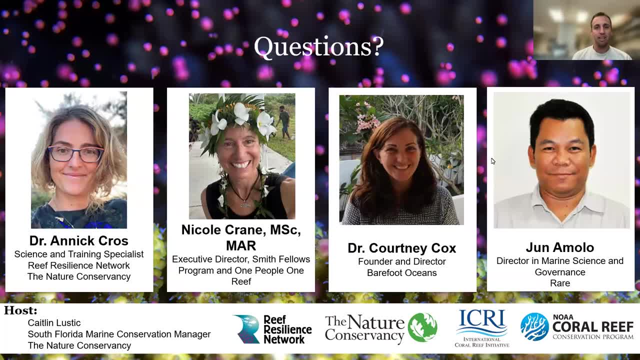 Yeah, it's super. It couldn't be more simple. You know it's a kit that you get, that we got from a lab that costs $200, and it comes with everything from gloves to the filter that you need Filter a liter of water, mail it back to them and a week later you've got your data and 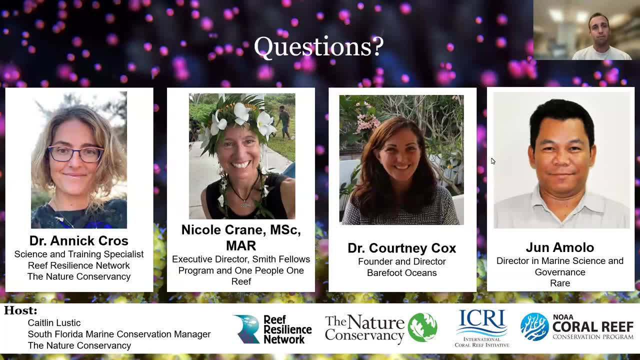 analysis. Great Thanks, Nicole. this was also for you. What were some management decisions that were informed by the analyses that you conducted? Okay, yeah, thank you. Yeah, and I also want to point out that the list of people involved in doing this work 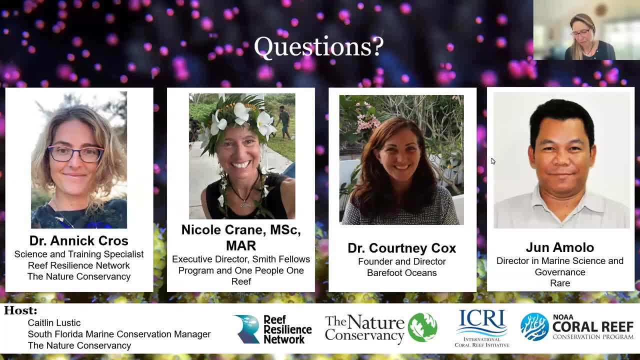 is so long, and so I want to give a shout out to every one of them, because it's such a collaborative project that we have. One of the first things that people did was reinstate a number of their traditional management Plans. I guess you could call them. 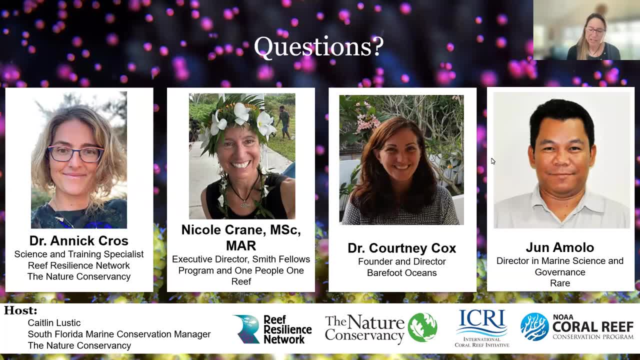 So, for example, on the small island of Falala, they decided to divide the island in half and the reef owner on one half decided to close it to, for example, spearfishing, because they recognized that some of those fish were crucial to coral larval recruitment and success. 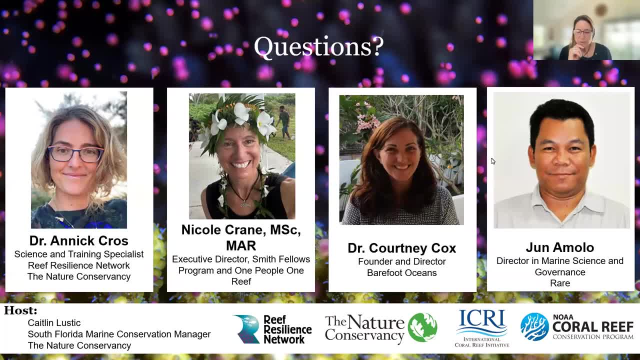 because of their role cleaning the reefs. So that was one thing that happened and they showed an increase in their fish biomass. within gosh eight months They almost doubled their biomass Amazingly quickly. So that's one of the first things that's happened is in recognition of movement and 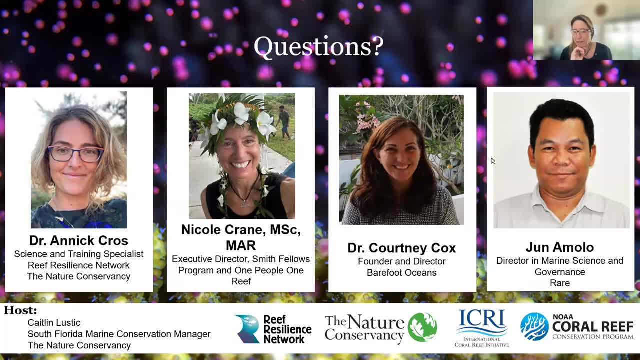 have islands sharing different organisms that people recognize that you can't manage in a vacuum, and so they came together to think about how they could work together, and they're now currently forming an island-wide, an atoll-wide sort of council that works between the different. 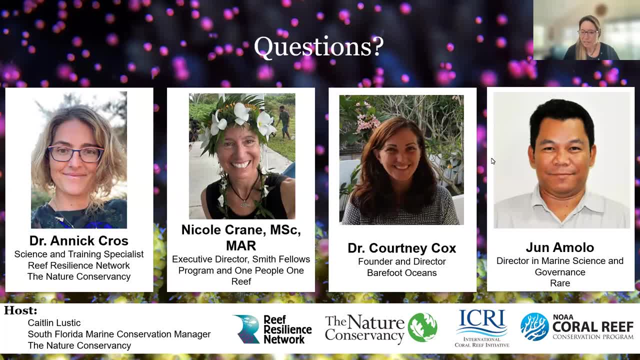 clans, which they haven't had in the past. So those are all things that have been informed in part by the connectivity work and the other work that we're doing out there. Great thanks. Here's a question that came in during Courtney's talk, but I think it could probably go to any of you. 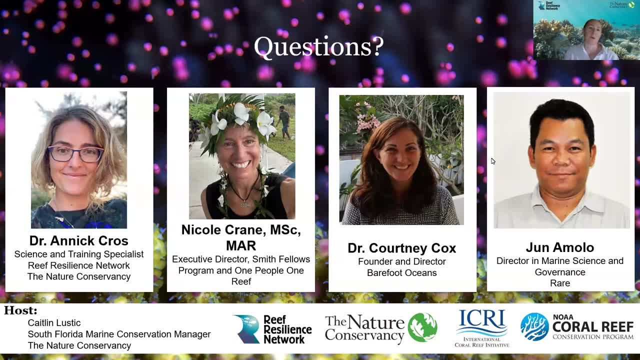 In what instances would larvae export be high? but import is low, Courtney, why don't you go ahead with that one? Sure, In lots of cases they're correlated, But there are in some cases where the export- so self-recruitment, for instance- could be high. 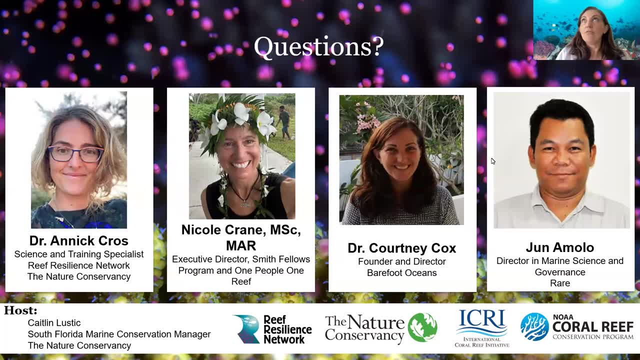 and export could be high, or export is relatively higher than import. If this is the case, there's going to be some challenges there. so these types of things can also identify some of the challenges that some reefs could be facing. how high 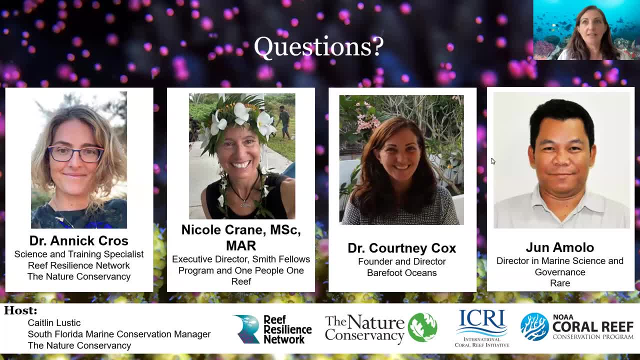 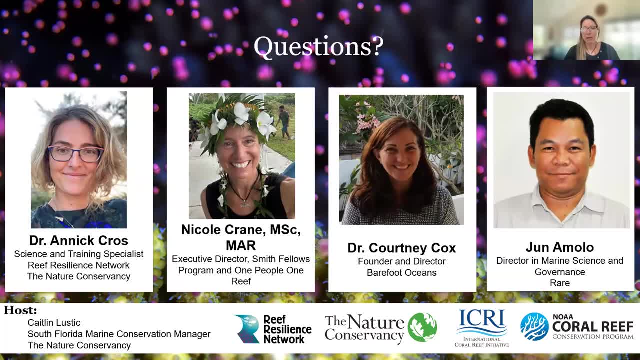 receiving. So these are all really important questions when it comes to thinking about what are the impacts when you've got a, let's say, an island effect of a healthy reef and surrounded by a whole bunch of bleached reefs or reefs that are damaged. So what happens when that? 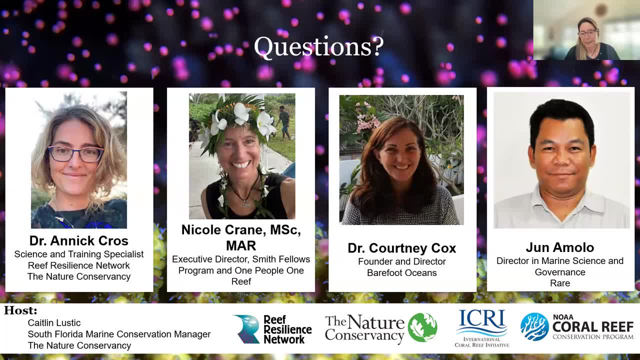 healthy reef keeps putting out larvae but it's not receiving enough. Yeah, And also, just to clarify our export and import metrics: consider both the volume and the diversity So you could have for the metrics that we're using. you could have a low export value if the volume is low. 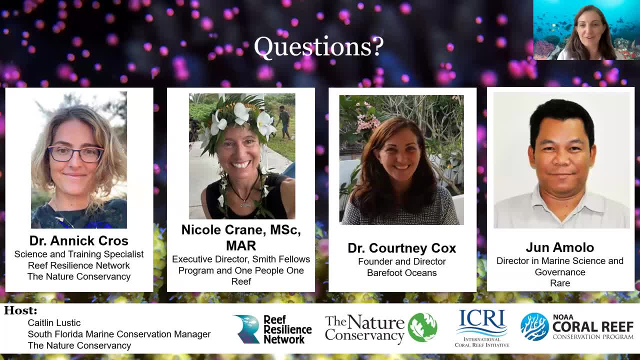 but the diversity is high. Actually, you asked the other way. So if you have a high export, it could be that the volume is high but the diversity is low. So it's considering both of those components in the metric that we're using. 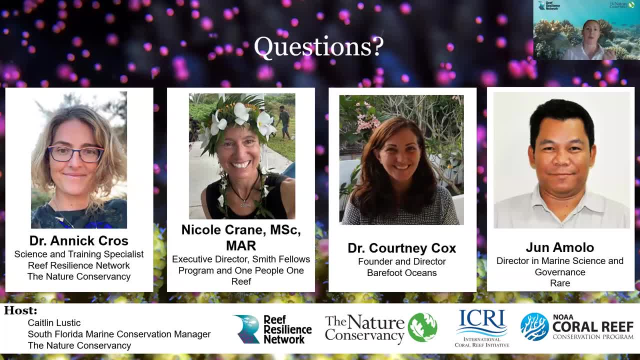 Great Thanks, Let's see, Nicole. you mentioned that the genetic connectivity presents parallels with the social connectivity. Can you speak more about that? Did you measure social connectivity And, if so, what are the relationships between the social and genetic connectivity? 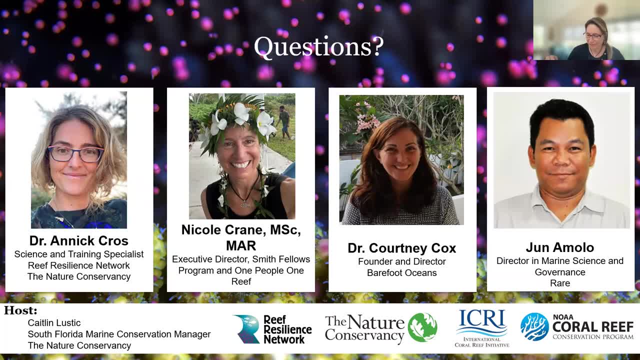 Yeah, So I wish that Magul. I wish that Magul was on the call, but if he is, he would speak up. So what we found is that the main parallel is that connectivity goes both through people and through organisms and the physical environment. So those things are all connected And I think 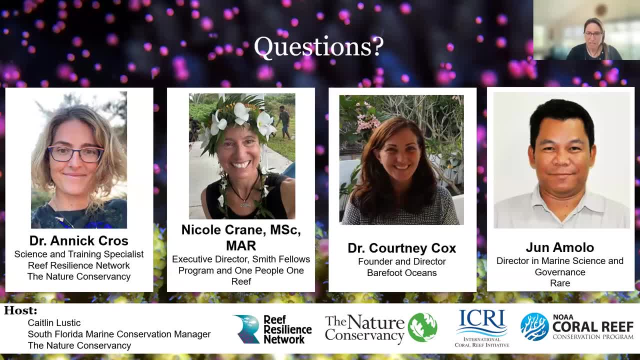 one of the main things we found is that two of the jurisdictions that had not worked together for quite a while actually were the ones that shared full siblings of two of the different fish that we were looking at, And so that's one of the things that we found, And I think that's one of the 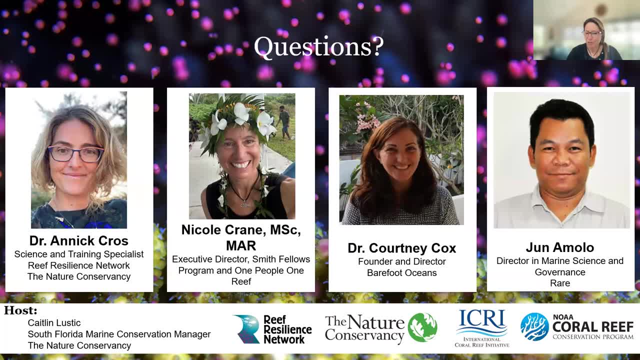 key things that we found is that two of the jurisdictions that had not worked together for quite a while. that was really exciting to them and they realized that if they don't work together- since they do share their fish- if they do work together they can gain a lot more. 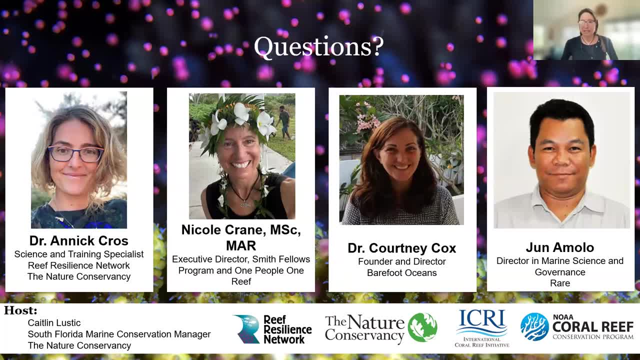 So we're actually right now beginning the process to answer more of that question. So we're having the communities map their jurisdictions, We're having the youth actually work with their elders to try to regain some of that knowledge and to map those jurisdictions, and we're going. 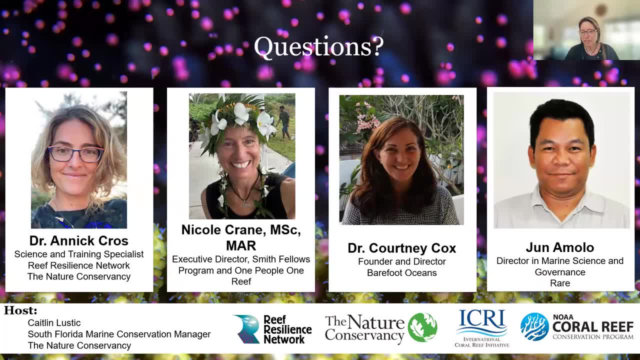 to overlay those onto the connectivity. So the map I showed you of jurisdictions is a sort of our initial map from our talking to people. we've now put it in their hands so we're asking each of them to more fully map all their jurisdictions so we can overlay that on the connectivity. so we're in. 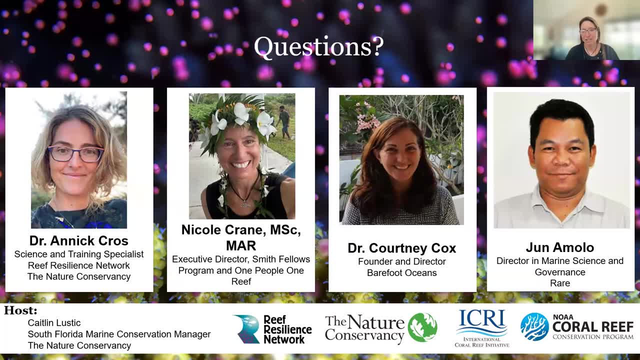 the process of doing that. it's actually really fun they're. they're having a lot of fun doing it and it's i think it's rekindling a lot of interest in the youth about jurisdictions and management, what has been lost and what they can recover. i hope i answered that question. 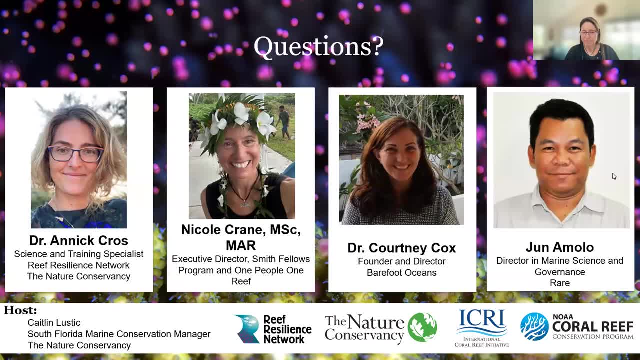 uh, let's see. we have a question for june. when you say that you're sharing the larval dispersal results with the community, are you talking about the municipal level, or do you have interactions with the barangay level, if i'm saying that correctly, for the creation of these no-take zones? 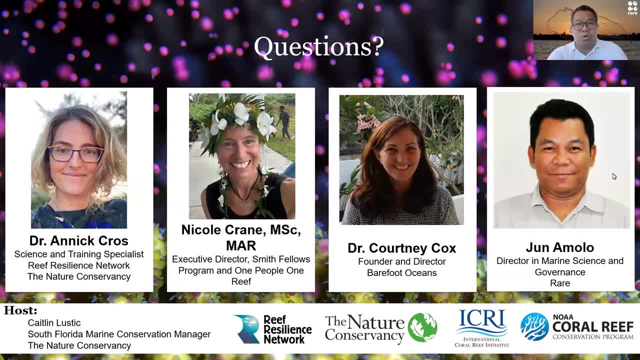 yeah, this is really at the both municipal and barangay or the village level. so you're really talking, you're presenting the map and you're sharing the results with the community to fishers or gleaners or other you know resource users in the coastal zone at the village level. 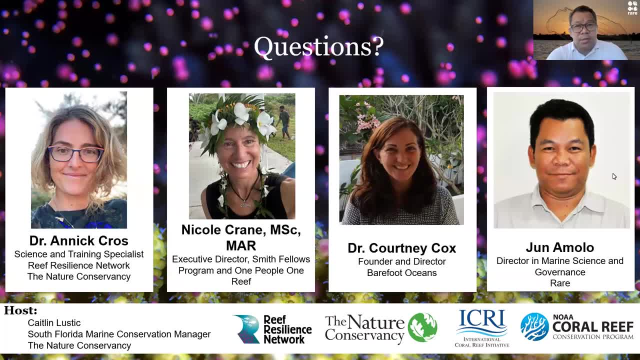 and then they get to input their decision as to where to put these no-take zones, both village and municipal level. um, there's a question: what management strategies are being used to reduce the montipora coverage and restore the reefs? that's a really good question. so initially the people asked us: 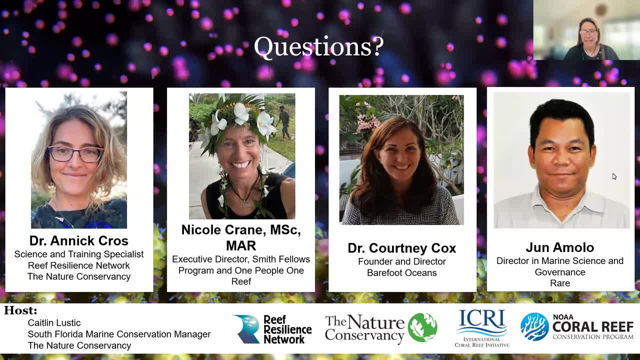 exactly what that question: what should we do? and we don't like to be in the business of telling them what to do because i don't know if it's going to work or not. um, they wanted to know, for example, should we bleach it? should we throw chemicals on it? should we hammer it up, you know, should we? 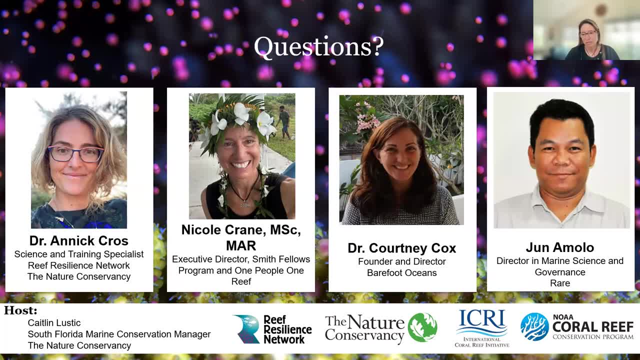 physically. what should we do? and you know, our suggestion was just leave it alone and and see if, if sort of the reefs can take their own course, which they have in some cases. that mog mog example, i told you, is exactly that. so that was really interesting for us to see that there can be some. 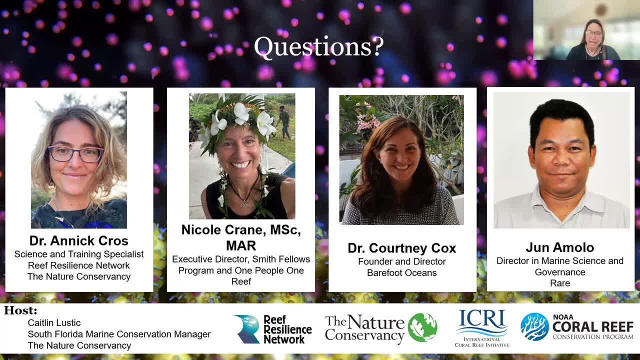 solutions just based on what happens naturally. other than that, there's the best way that the advice we gave to people is: manage for your fish, because it's much easier to manage for fish than it is for corals, because you know unless you're planting corals, which they're not, so that's what. 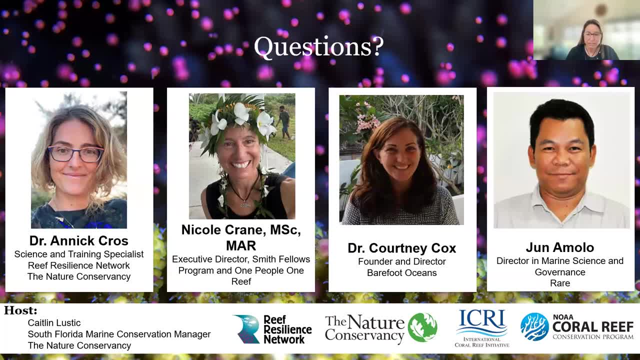 they decided to do- and mog mog was one of the first things that they did- and they decided to the places that managed pretty heavily for their fish. so they they restricted the take of a lot of their herbivorous fish and so you know, i don't know if that's what drove that resilience or not. 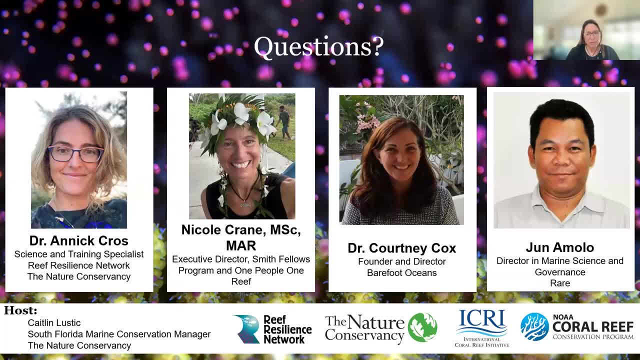 but it was probably a factor. so that's really what we're, you know, sort of proposing to them is that they really think about the fish, because that's what they're eating and that's what they're catching. so it's the easiest thing for them to think about and- and i'll just say a quick comment- 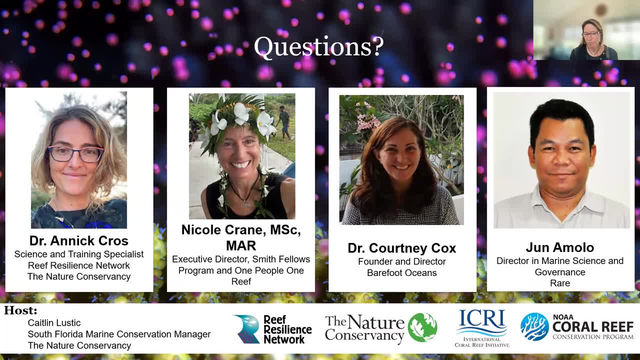 here about mpa, so the places where we work are autonomously governed, so the people can make decisions about their reefs, which i think is really it makes it much easier to manage for them. no, take mpas that are imposed on these people can actually be devastating, because they 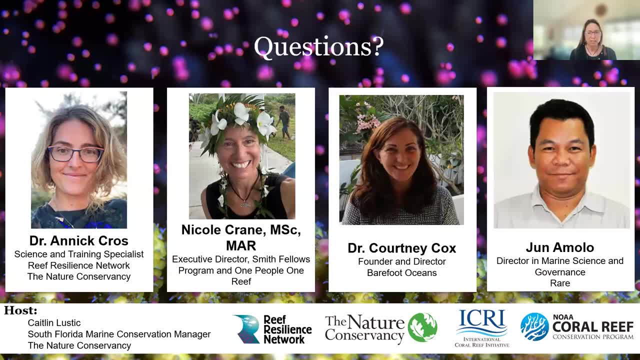 are managed by families and clans, and if you take away somebody's access to a reef, it actually creates a lot of social instability. so this is why we're really embedding all this stuff within their own management system, and i think we're super lucky to be able to do that, because it 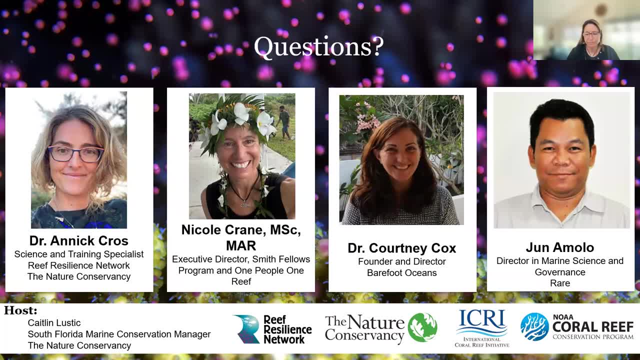 is a place that is managed by the local people. okay, thanks. has there been any attempt to assess the vulnerability of connectivity patterns to projected future changes? are these likely to be durable in the context of climate change? courtney, yours is the big model, so i'd say that's going to be huge for you. 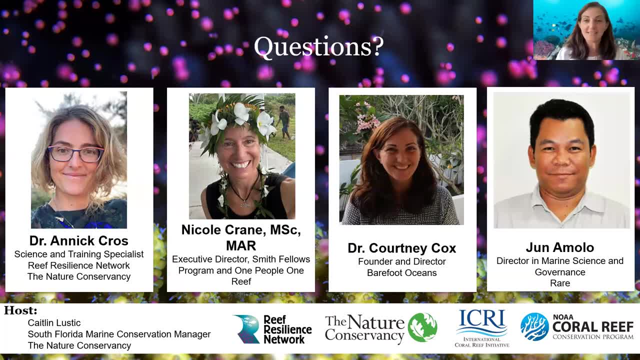 yeah, and the answer is yes, um. so that's a huge, huge area of focus, um on how all of this change um, depending on how we're going to do it. so i think it's a really big question, and i think it's a really big question, um depending on how the temperatures change, how currents change um. so 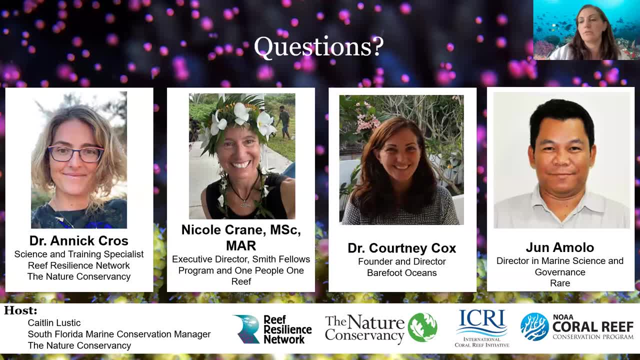 we've been working with the university of tasmania to to look at the effects of temporal changes. so we have been looking at how, because we're also, i guess, to clarify one thing, that the the model that we're using is using 20 years of hydrodynamic data, um, but it is taking an average over those. 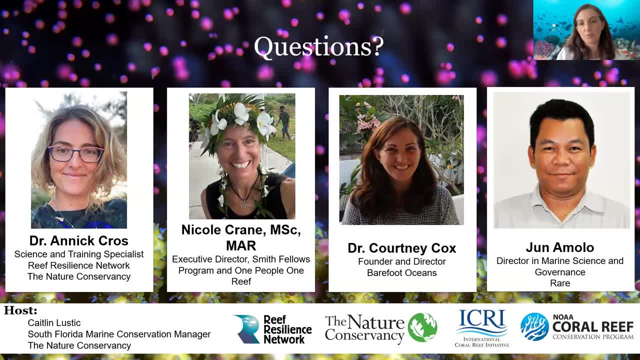 20 years. so we're also looking at the variability um, the temporal variability within those years, and how that changes um, where you would would protect um, but then looking further into the future on how current patterns will change under different climate scenarios: um, yes, but to be determined um and 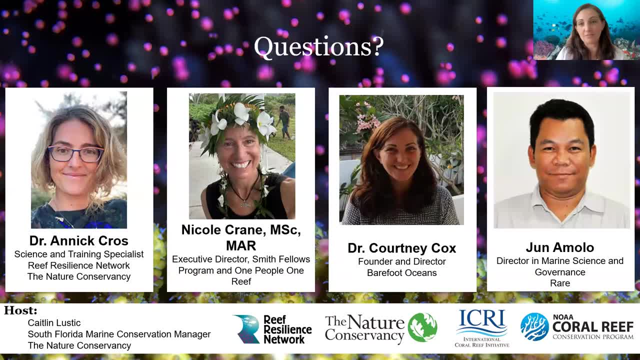 things are going to change and the areas that are that are optimal for protection are going to change, um, the species that are even there are going to change. so i mean that's a big, that's a big question, um, and a big need to understand those impacts. it's a huge question i think we're addressing. 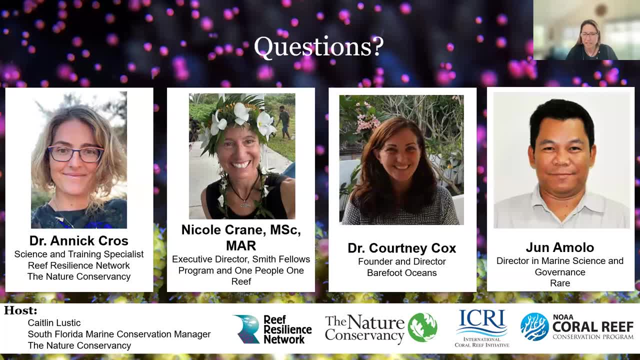 that question, looking at resilience through the human lens and really encouraging, strengthening management as much as we can, given the fact that we can't really project so far into the future that way, um, but any management is going to be helpful and useful and so, and people are going to 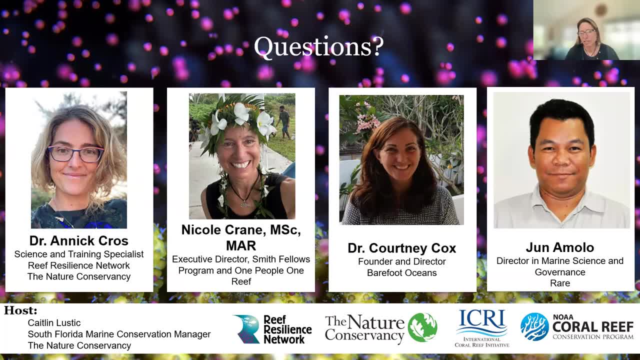 need to eat from those reefs and so for them. they can't really close them down to no fishing. however, strengthening the management around some of these key fish that we know are moving around between the reefs is really all that we can do. to look ahead is to just strengthen that management. 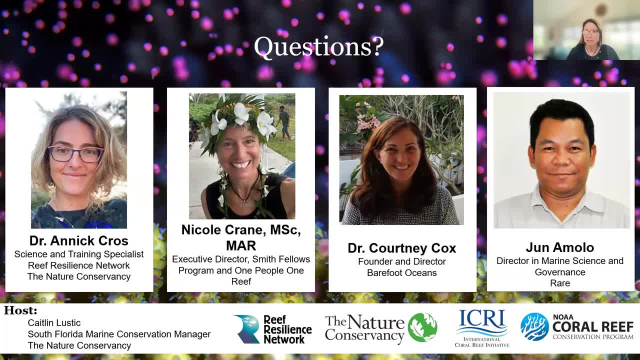 in the best way that we can and then we continue to provide the science behind it so that people can continue to be informed. and that's the resource piece, the science resource piece, to so many island communities. if they can get some of that information as they're managing, it helps them. 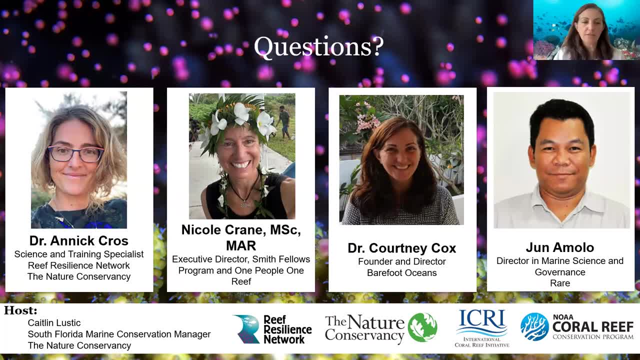 adapt. yeah, just to echo that, um, um, you know, getting this data, even if it's not modeled for the future, like nicole said, if we get this data into the hands of the people who can use it, um, and then, if we need, if we refine the 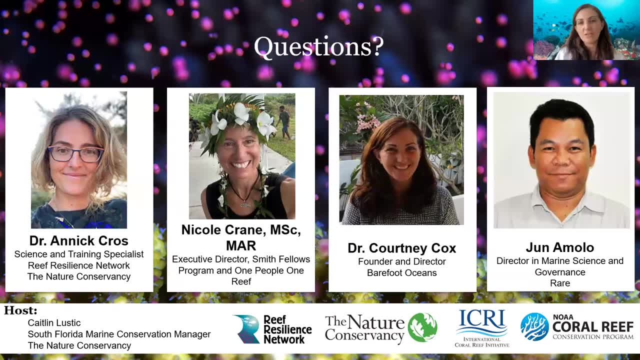 information, then they're equipped and have the capacity to use it. um, and you know, june's talked about that- and teams like rare and other organizations that are working directly with the communities to build that capacity to to use the information, and that's huge. okay, i think we only have time for one more question. um, has anyone explored different human? 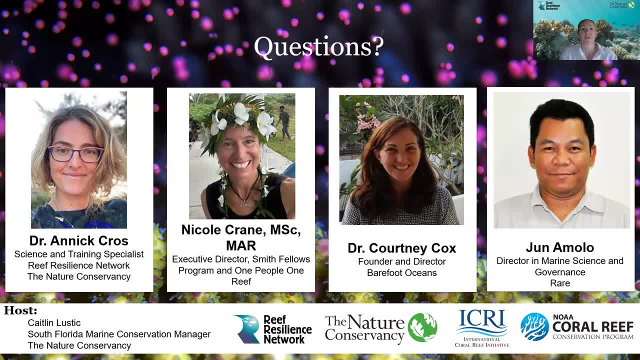 intervention strategies to support or fast track the natural processes that help to restore degraded reefs, especially in areas that are of social significance. maybe we can ask, june that i don't know if you have thought in your strategies about um restoration strategies with your the connectivity data that you've been handed on over. yeah, i think that's a great question. 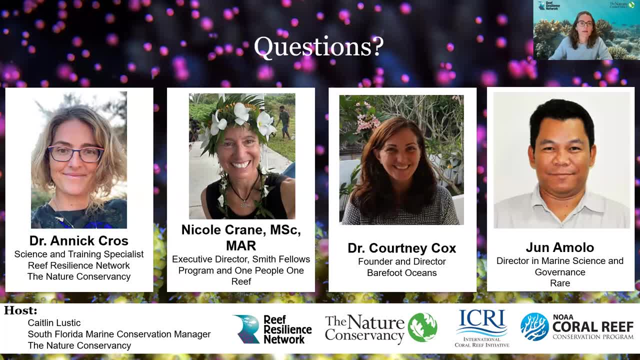 um, although, uh, restoration, uh, that's for me right. yeah, question, uh, yes, uh, so, although, yes, please, thanks, uh, although in the country there's very few organizations that's really looking into restoration of degraded reef, nobody, um, i don't know, maybe one or two organizations that have been. 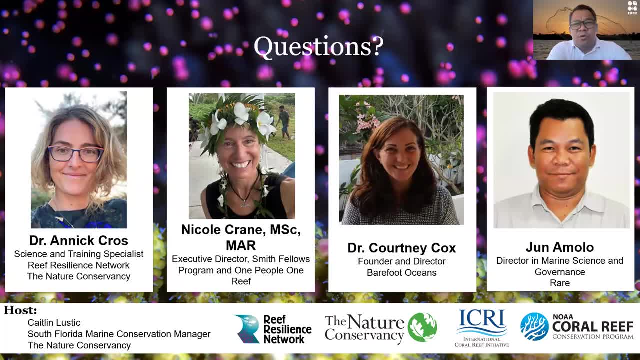 looking into restoration, but right now, uh, the focus is really much on uh identifying uh reef connected. you know highly, you know source or sink reef to protect it from uh. add further, further degradations from. you know you know overfishing or other issues, uh, and then so, yeah, that's, that's more of the focus, but yeah. 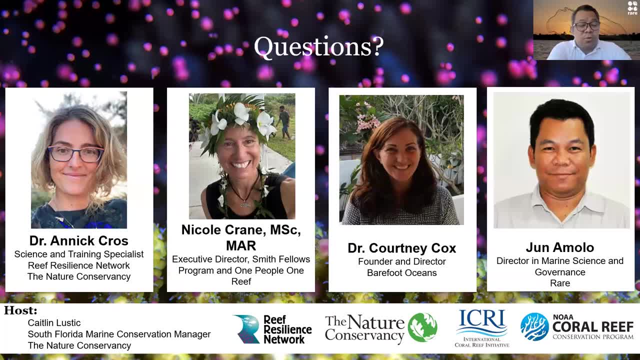 we're very much willing to share this information to organizations that really looking into restorations. uh, right now, i think only you know academic organization are trying to do restoration in in some of these great thanks. that concludes, uh, this webinar. so i just wanna once again thank all of our wonderful 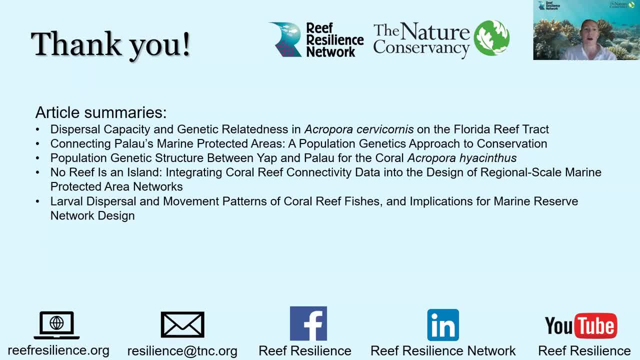 wonderful speakers and the rest of you for being here with us. um, the recording will be made available in the next few days and we will see you next time, bye-bye days. We'll also probably pick a few of the outstanding questions and have those answered. 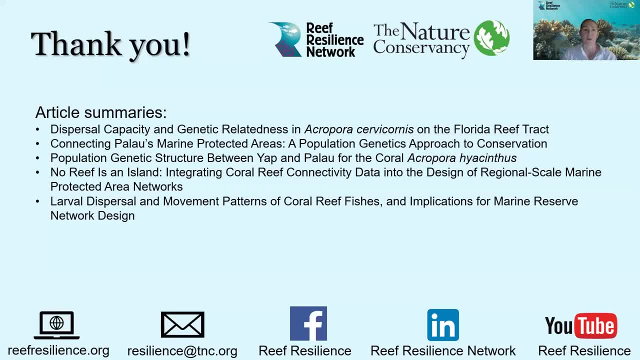 by our speakers and send that out, And the article summary is here. We have a number that are available on the Reef Resilience Network site and we will send links to these as well, If you're interested in learning more about the Reef Resilience Network or have any further questions. 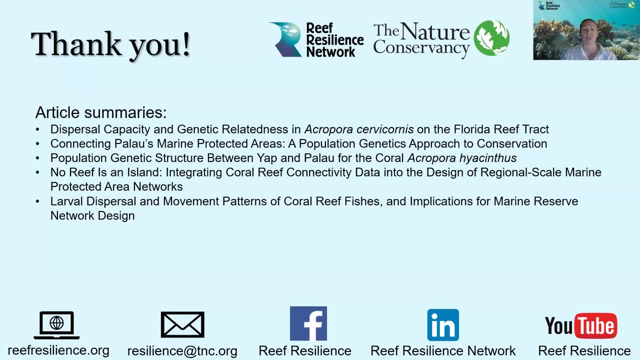 or conversation you'd like to have with speakers. please feel free to reach out to us at the Reef Resilience Network. We can put you in touch. Thank you all for being here. Thanks everyone. Thank you so much. Thank you Everyone. Thank you.